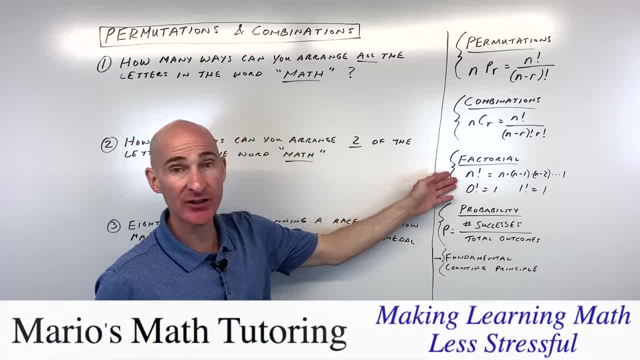 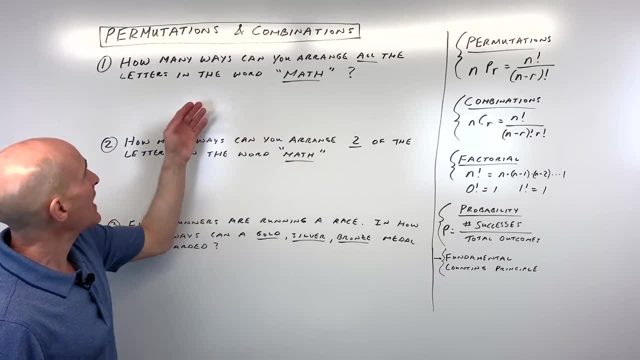 different definitions. We're going to be working with permutations, combinations, factorials, probability in a few of the problems, as well as the fundamental counting principle. So let's dive into the first problem and we'll kind of explain this as we go through it. 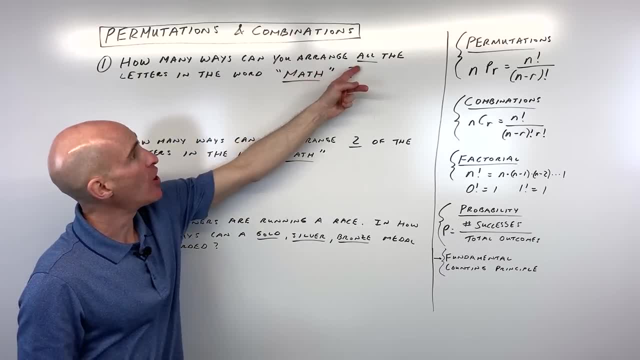 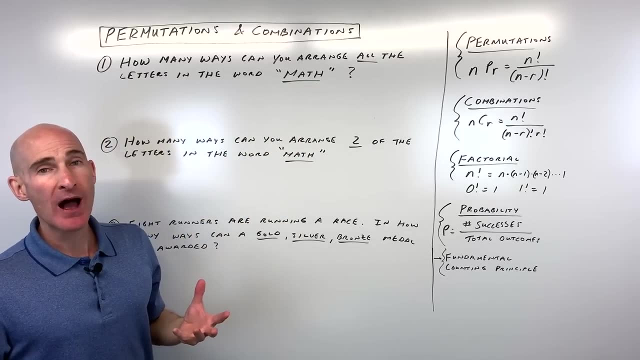 For the first one, it says: how many ways can you arrange all the letters in the word math? So what do you think for that problem? Well, there's a couple different ways to do this problem. One way to do it is to use the fundamental counting principle, and what you would do is you would. 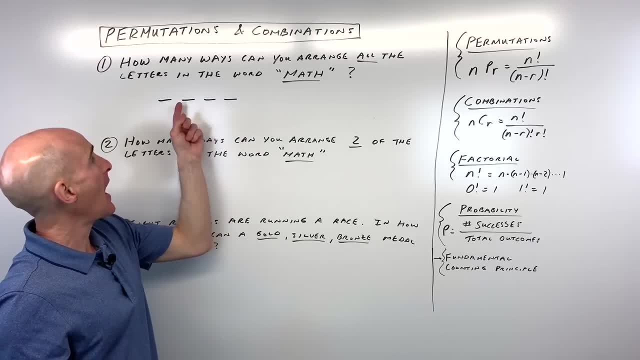 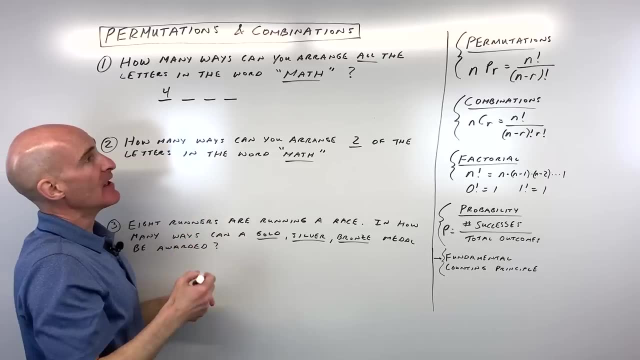 diagram this out. You'd say: there's four letters. How many choices are there for the first letter? So imagine if you were picking these letters out of a bag. Well, there would be four choices right, And then, once you pick one of the letters, there's going to be three left. So you're going to have 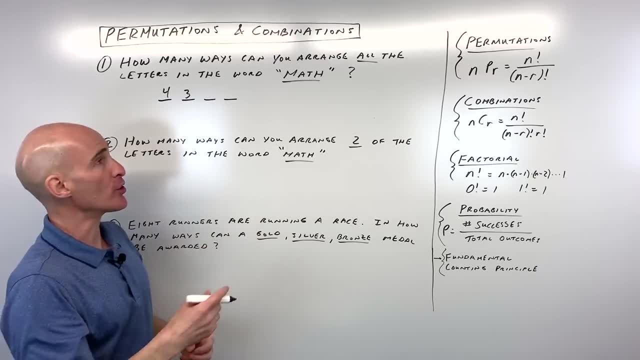 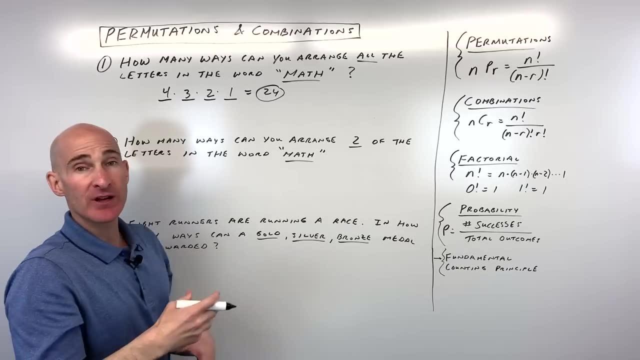 three possibilities for that. So you're going to have three possibilities for that. So you're going to have three possibilities for that Second letter that you pick for the word two and then one, And if you multiply those together, you're going to get 24 different so-called words involving the four letters in math. 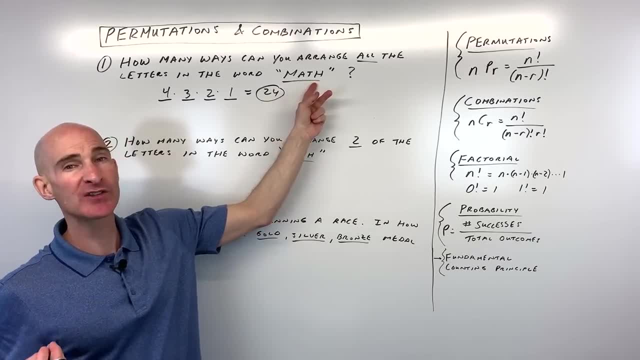 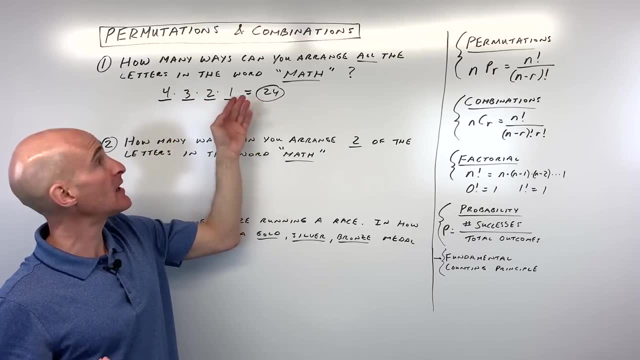 Now notice there's no letters repeated- and we'll talk about some of the problems later on where there's repetitions of a particular letter, But for this one it's just going to be four times, three times, two times one, And this is the fundamental counting principle. 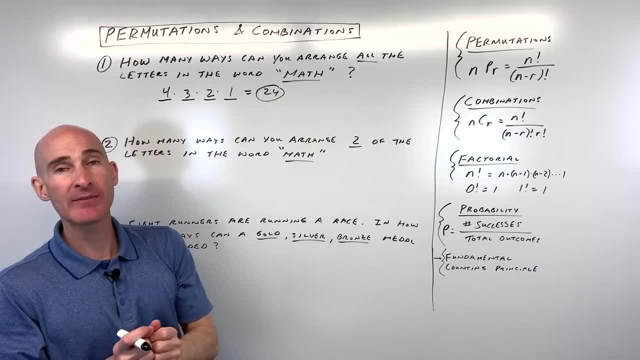 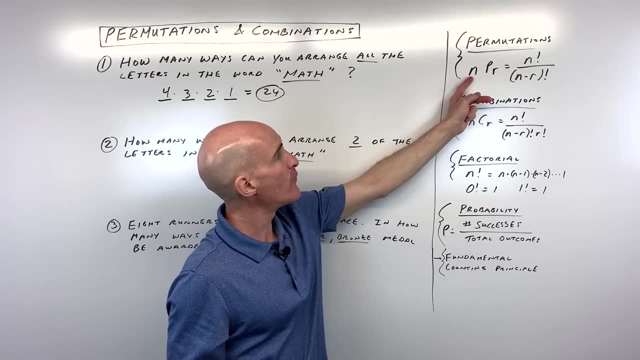 You just see how many choices in each category and you multiply them together. The other way to do this is to use this permutations formula here And what you could do is you could say: out of four objects you're picking, like p for picking or permutations, four p four You're picking. 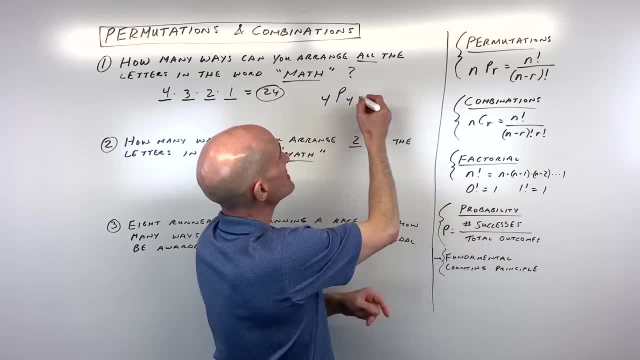 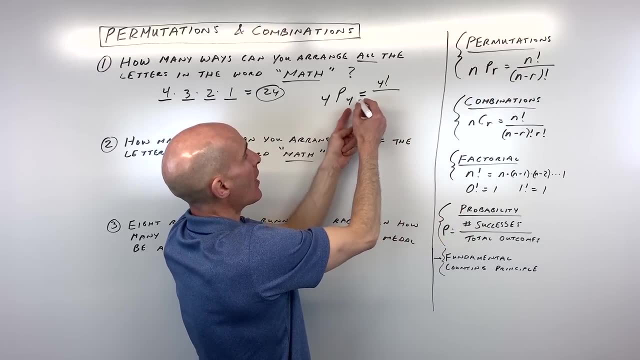 four out of four, And so if we put this into the formula here, you can see that this number that comes in front is our n. That's going to be four factorial over four minus r, which r is four. so that's four minus four factorial. So this comes out to four factorial over zero factorial. 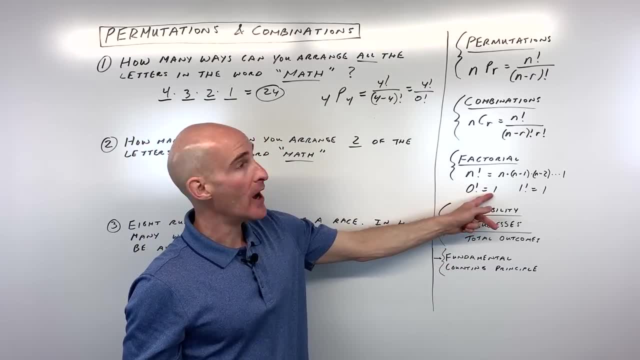 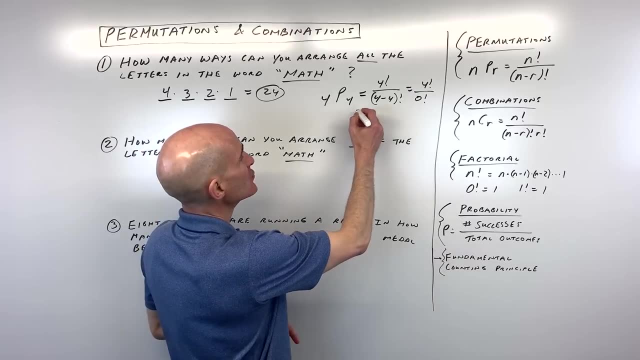 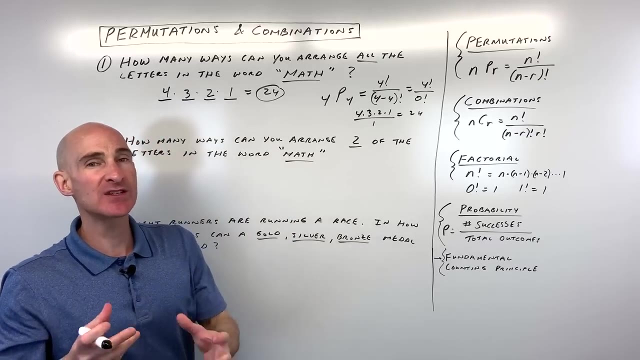 And you want to memorize that zero factorial is actually one, But with four factorial is you start at four and you multiply consecutively down to one. So this would be four times three times two times one, all divided by one, which is the same thing. we got here, 24.. So two different ways to 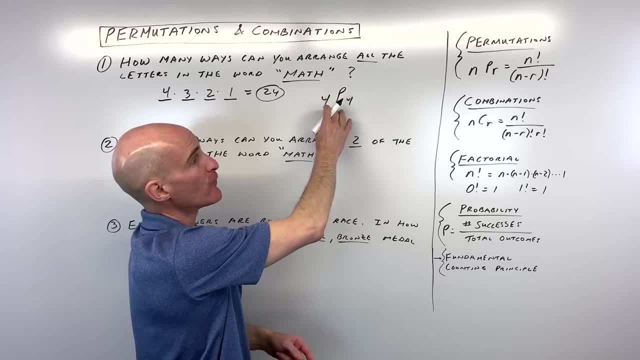 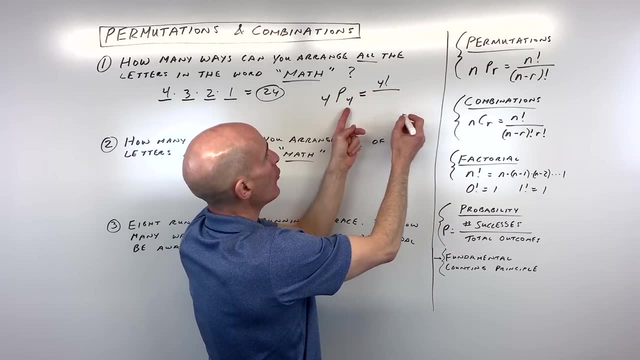 or permutations: four, p, four. you're picking four out of four, And so if we put this into the formula here, you can see that this number that comes in front is our n. that's going to be four factorial over four minus r, which r is four. so that's four minus four factorial, So this comes out to four. 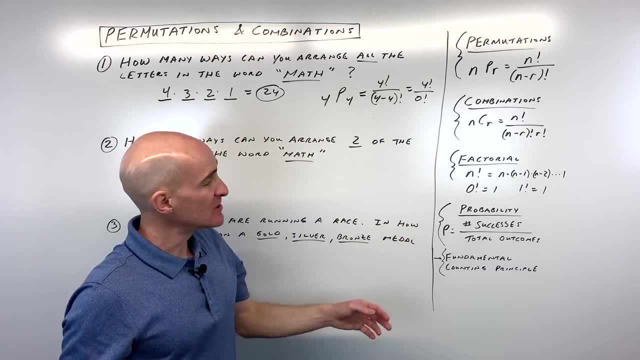 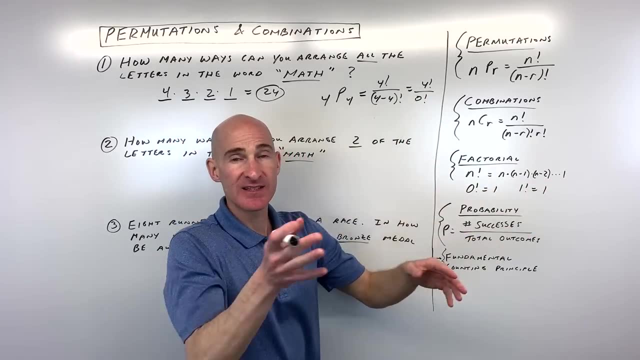 factorial over zero factorial, which is four minus four factorial. So that's four minus four factorial And you want to memorize that zero factorial is actually one. but with four factorial is you start at four and you multiply consecutively down to one. So this would be four times three times two. 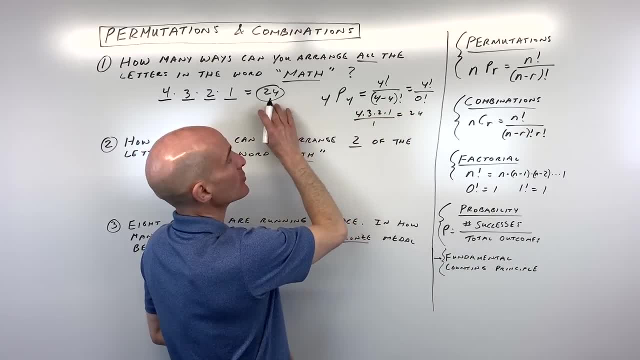 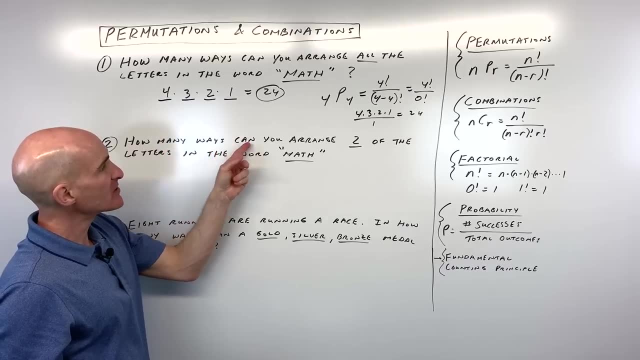 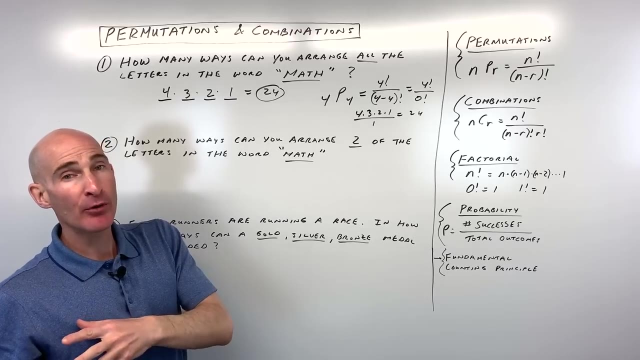 times one, all divided by one, which is the same thing. we got here 24.. So two different ways to look at that one. For number two, it's very similar to number one. it says: how many ways can you arrange just two of the letters in the word math? Okay, what do you think for this one? A couple of 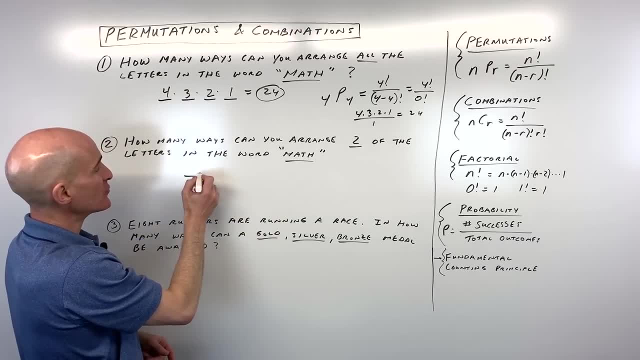 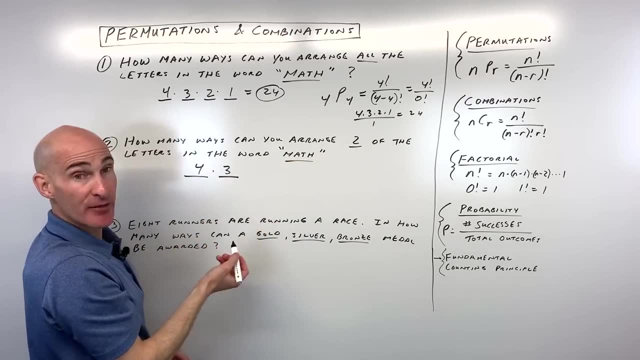 different ways to do this as well. You could use the fundamental counting principle. You could say: there's four choices for the first letter. Once you pick that letter right, how many choices are there in? for the second letter? There's only three. so four times three is twelve. The other way to do: 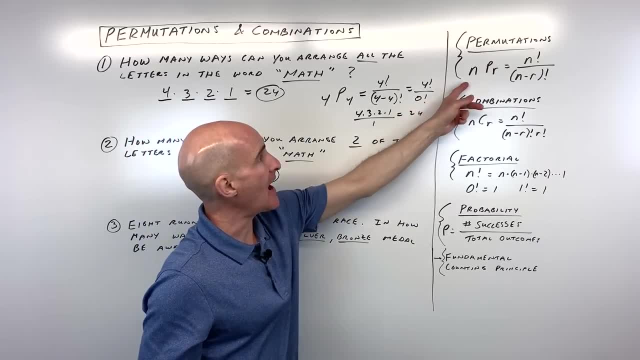 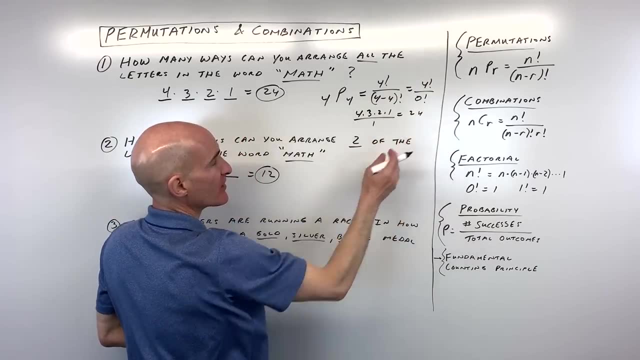 that is, to use this, a permutation formula here, out of n objects, How many ways are there to pick r objects, where the order matters? Okay, so the order is important with permutations, not with combinations. So, for example, this one would be four p two, which is four factorial. 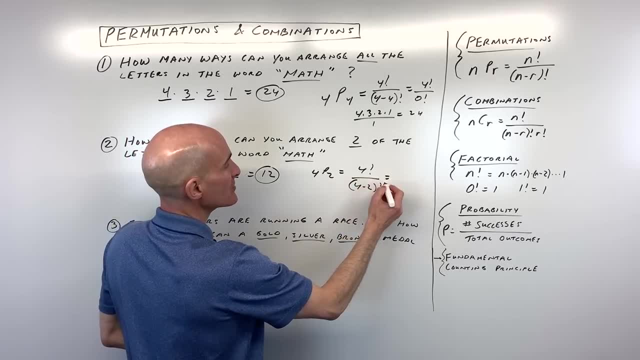 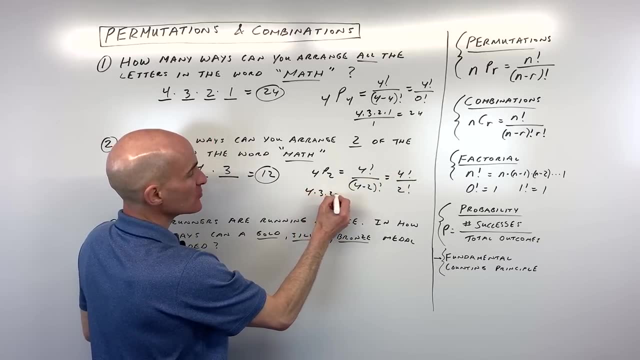 Over four minus two factorial, so that's going to be two factorial in the denominator, four factorial in the numerator. and if we expand this out four times, three times, two times one, over two factorial, which is two times one, you can see that these are canceling and we just get four times three, which 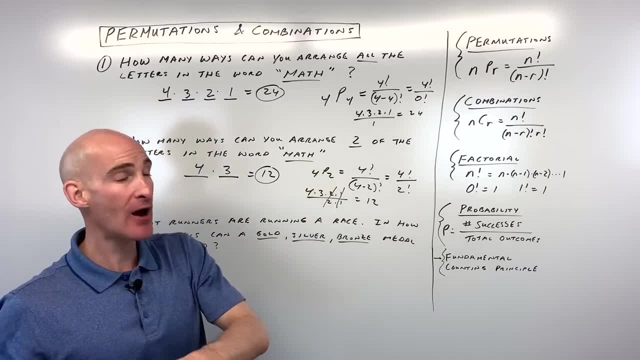 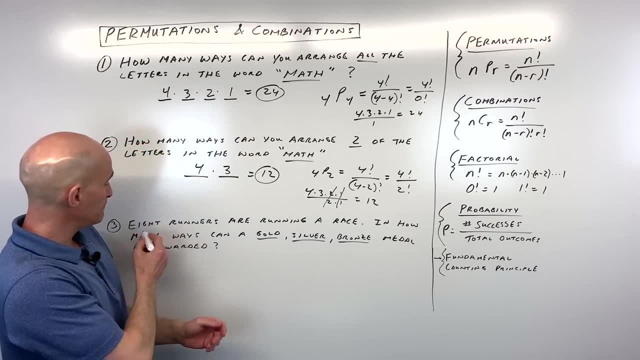 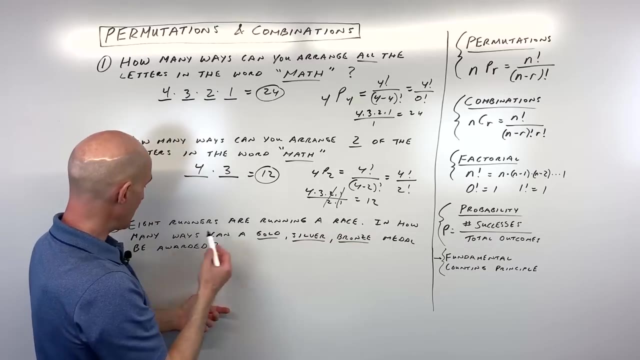 is equal to twelve- The same thing we got here. so either the fundamental counting principle will work, or using this NPR formula will work as well. Okay, for number three. now let's try this one. It says eight runners are running in a row. In how many ways can a gold, silver and bronze medal be awarded? 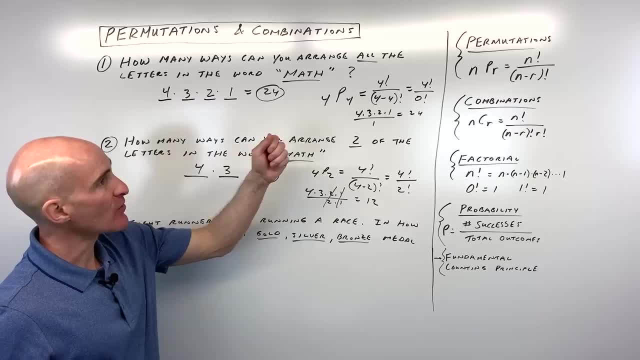 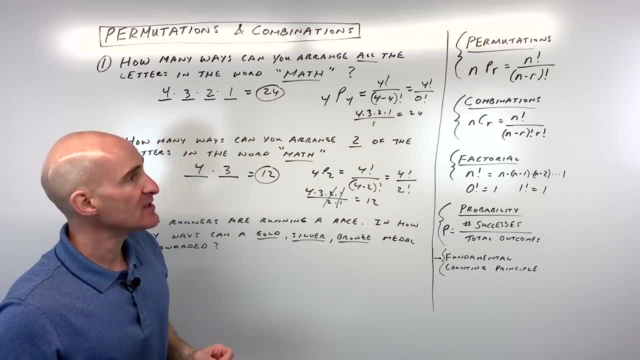 So what do you think for that one? So the question you always want to ask yourself on these problems is: is it a permutation, Is it a combination? Does the order matter or does the order not matter? Well, say, for example, runners A, B and C versus like C, B and A. So here you see, A gets the gold. 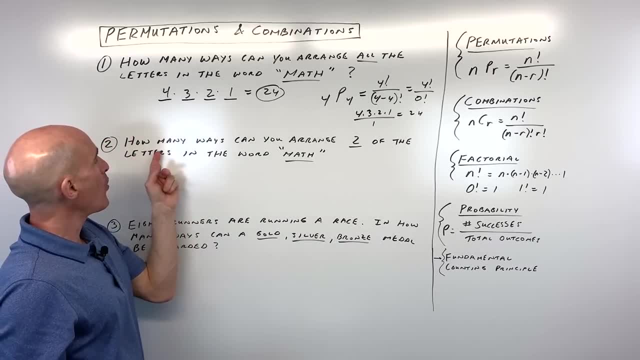 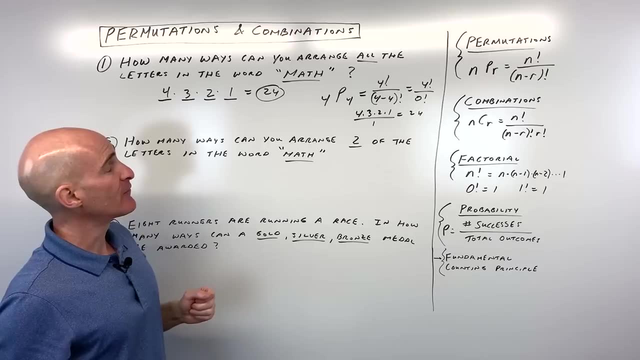 look at that one For number two. it's very similar to number one. It says: how many ways can you arrange just two of the letters in the word math? Okay, what do you think for this one? A couple of different ways to do this as well. You could use the fundamental counting principle. You could say: 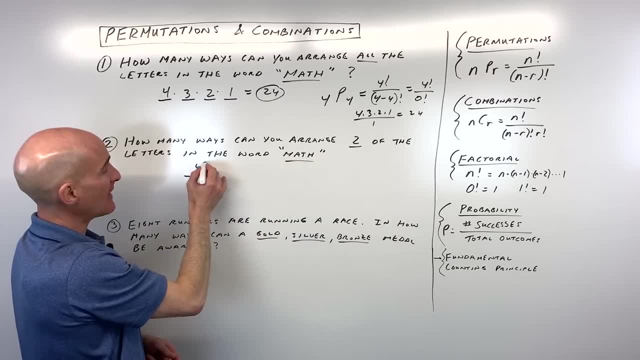 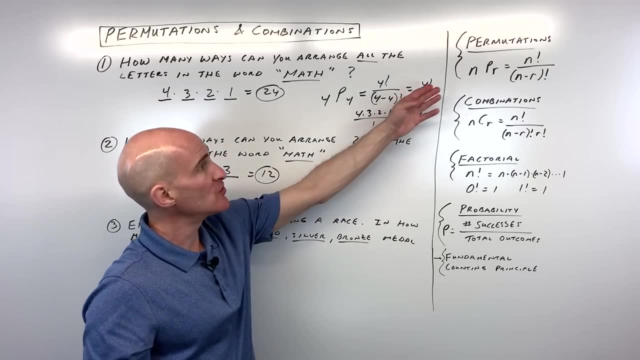 there's four choices for the first letter. Once you pick that letter right, how many choices are there for the second letter? There's only three. So four times three is twelve. The other way to do that is to use this permutation formula here: out of n objects, How many ways are there to pick? 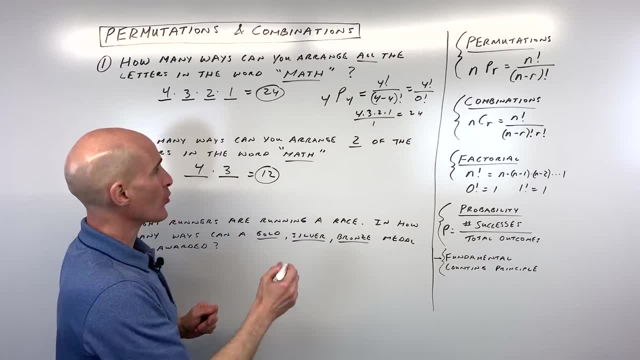 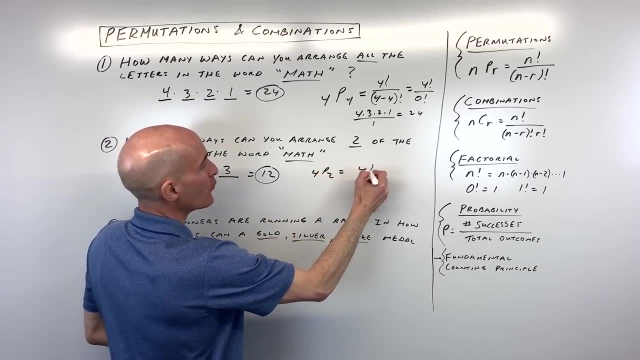 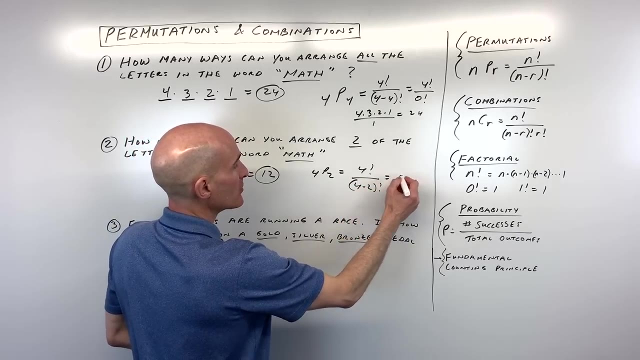 r objects where the order matters. Okay. so the order is important with permutations, not with combinations. So, for example, this one would be four p two, which is four factorial over four minus two factorial, So that's going to be two factorial in the denominator four. 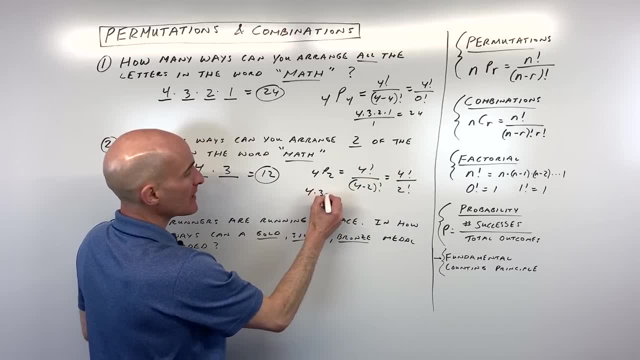 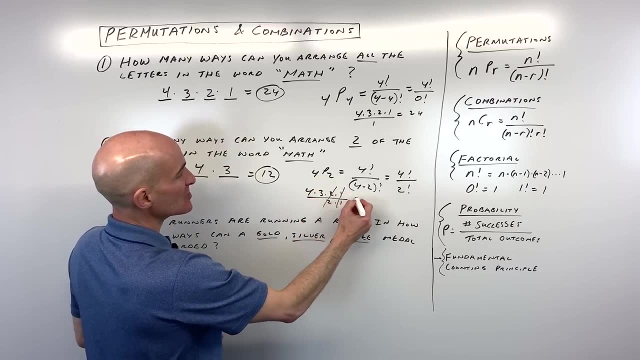 factorial in the numerator and if we expand this out four times three times two times one, over two factorial, which is two times one, you can see that these are canceling and we just get four times three, which is equal to twelve, The same thing we got here. So either the fundamental 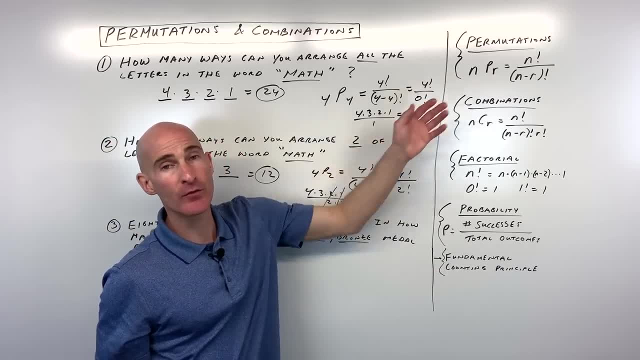 counting principle will work, or using this NPR formula will work as well. Okay, for number three. now let's try this one. It says eight runners are running in a row and the number of runners in a row is eight runners and the number of runners in a row is eight runners and the number of runners 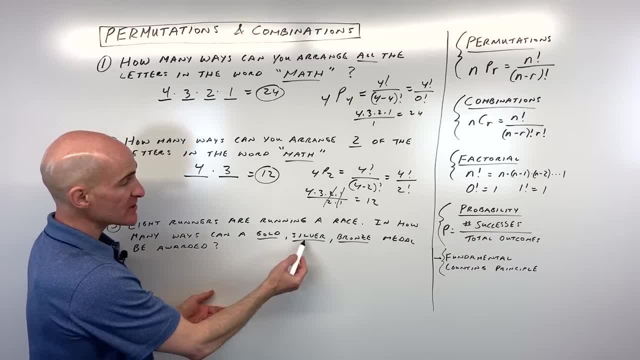 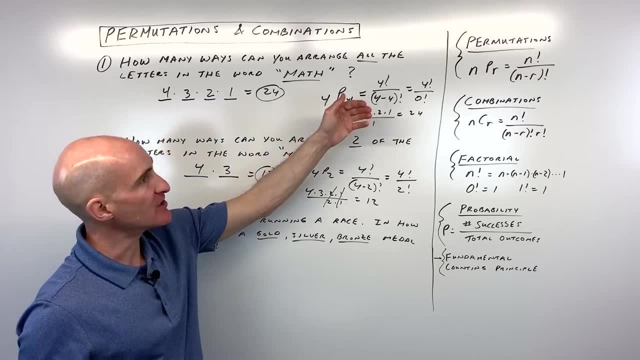 in a race? In how many ways can a gold, silver and bronze medal be awarded? So what do you think for that one? So the question you always want to ask yourself on these problems is: is it a permutation, Is it a combination? Does the order matter or does the order not matter? Well, say for. 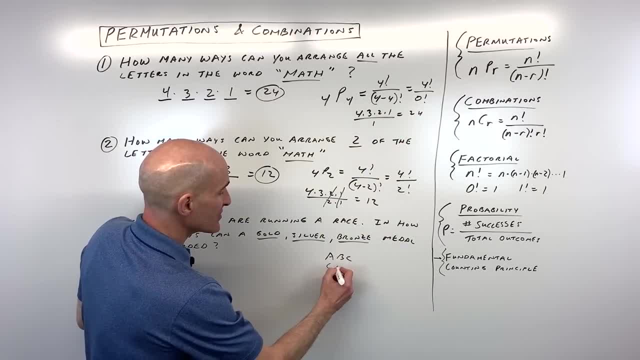 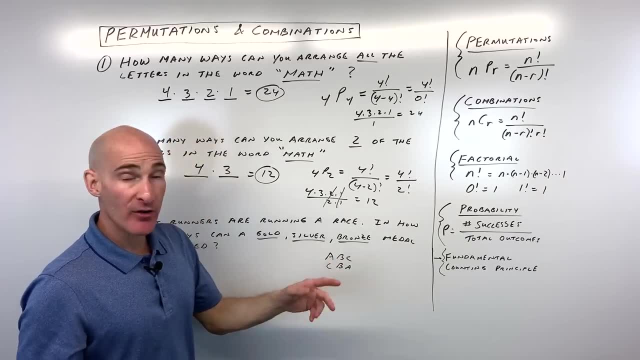 example, runners a, b and c versus like c, b and a. So here you see, a gets the gold medal, whereas here c is getting the gold medal. Same three people are finishing in the top three places, but it's a different awarding of medals. So this would be definitely a permutation. 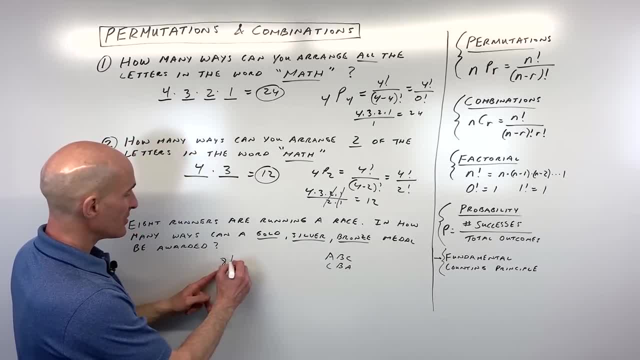 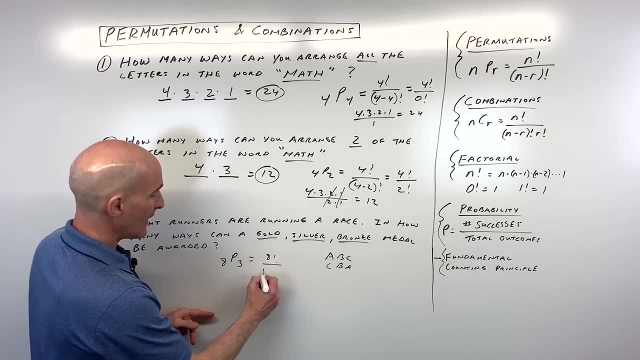 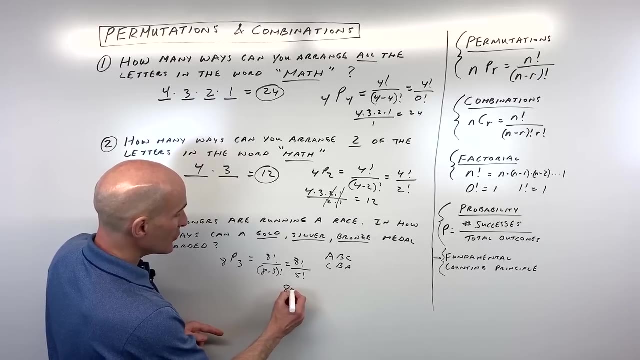 and what we can do is we can say: out of eight runners, you're picking three, okay, or eight. permutation three, which is equal to eight factorial over eight, minus three factorial, which is eight factorial over five factorial, And if you expand this out, you get eight times seven. 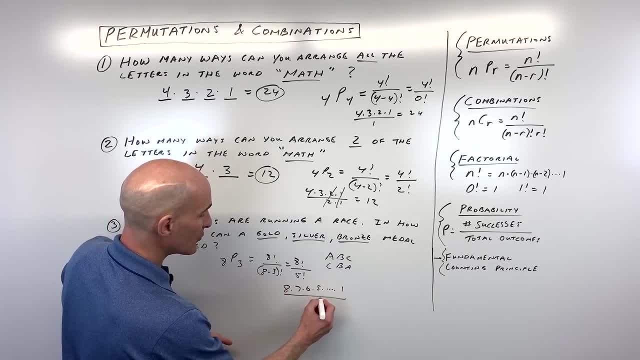 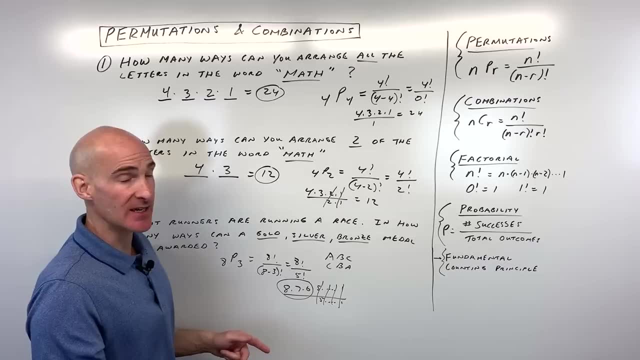 times six times five, all the way down to one. and five factorial is five times four times three, all the way down to one. So these are going to cancel out and you're going to get eight factorial over five and you're going to cancel all the way down. It's just going to be eight times seven times six. 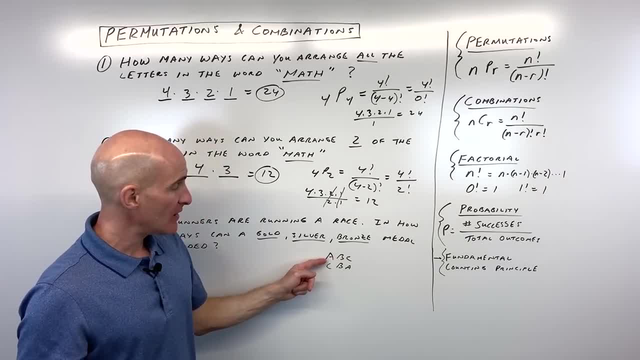 medal, whereas here C is getting the gold medal. Same three people are finishing in the top three places, but they're not getting the gold medal. So here you see: A gets the gold medal, whereas here C is getting the gold medal. Same three people are finishing in the top three places, but they're not getting the gold medal. 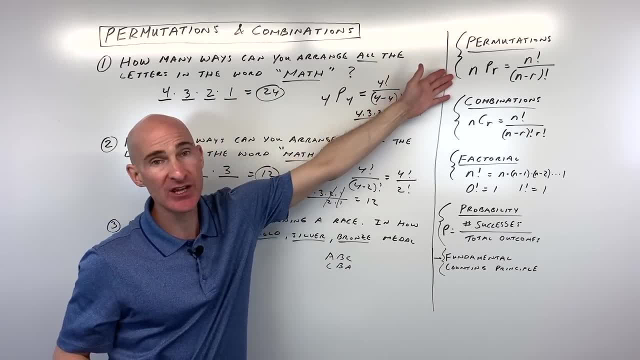 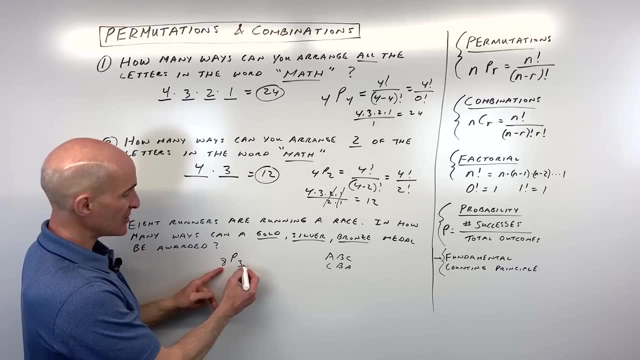 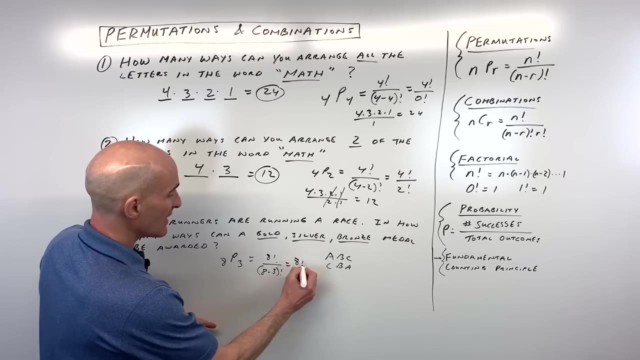 So this would be definitely a permutation, And what we can do is we can say: out of eight runners you're picking three, okay, or eight. permutation three, which is equal to eight factor over eight, minus three factor 40, gross is eight factor over five factor kay. And if you expand this out, you get eight times seven times six times five, all the way down to 1. and 5 is 5 times 4 times 3, down to 1.. So these are going to cancel all the way down to 1.. So if you expand this out of 9, you get 8 times 7 times 6 times 5, all the way down to. 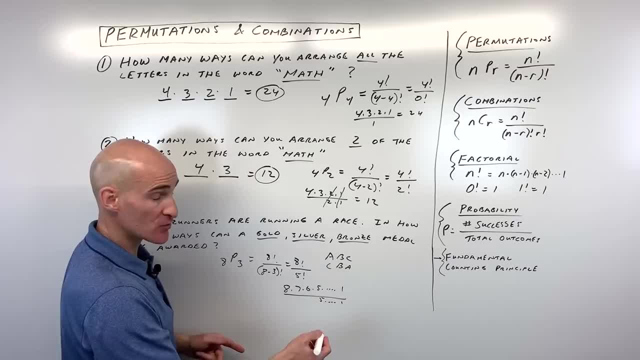 1 plus one And five. factor is 5 times four times three, all the way down to one. so these are going to cancel all the way down to one. So these are going to cancel all the way down to one. so in all, factorial is five times four times three, all the way down to one. so these are going to 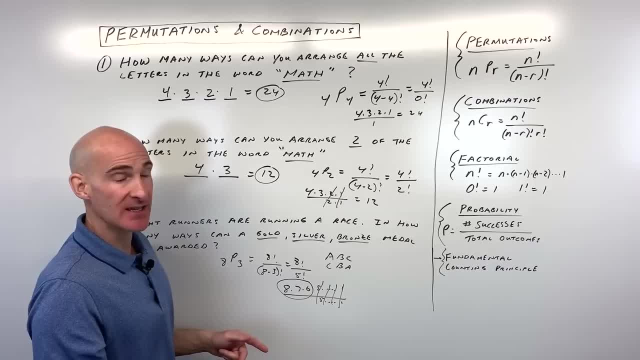 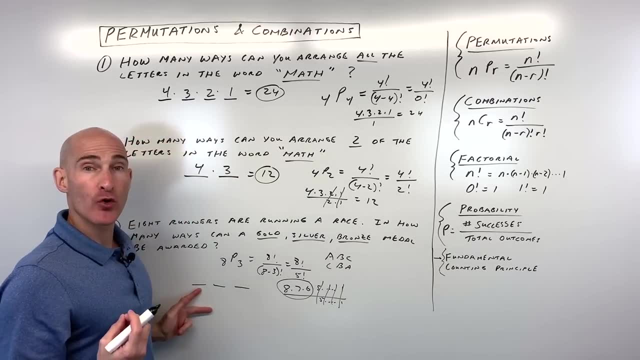 cancel all the way down. it's just going to be eight times seven times six, which makes sense, because if we were to use the fundamental counting principle here, we say: how many ways are there to award, like, a gold medal? well, out of eight runners, there's going to be eight. 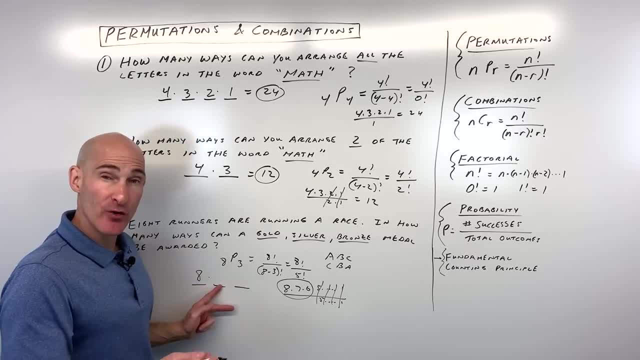 ways to do that. but once you award that gold medal, there's only seven runners left to win that silver medal. right seven and then six left for the bronze. so eight times seven times six, you can see we're getting the exact same result. and just in case you're doing this on: 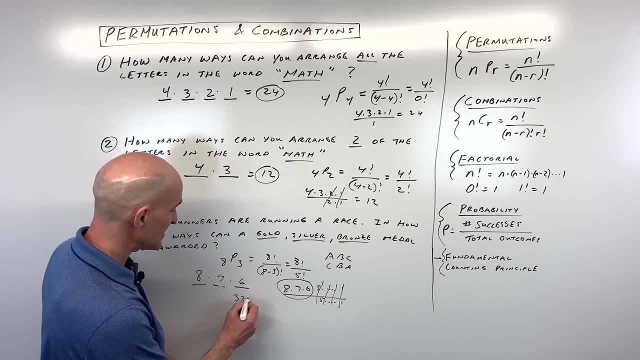 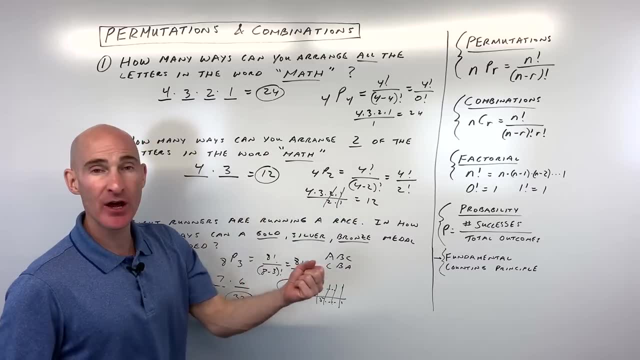 your own. let's get an answer here. that's 336 different ways or outcomes, so we haven't gotten into any probability problems yet, but here we're just talking about the number of possible outcomes. okay, number four. see if you can do this one. we've got 20 basketball players. form teams of. 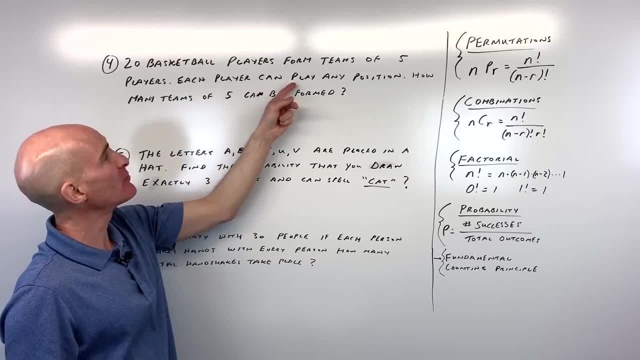 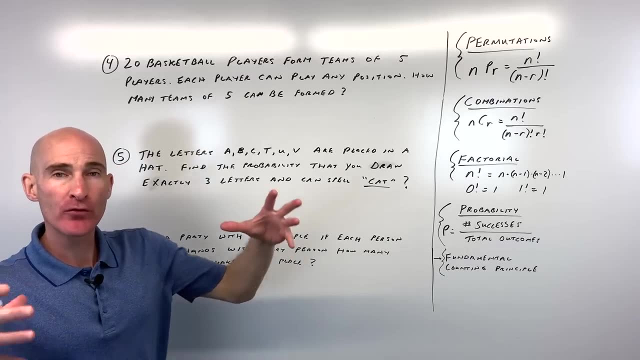 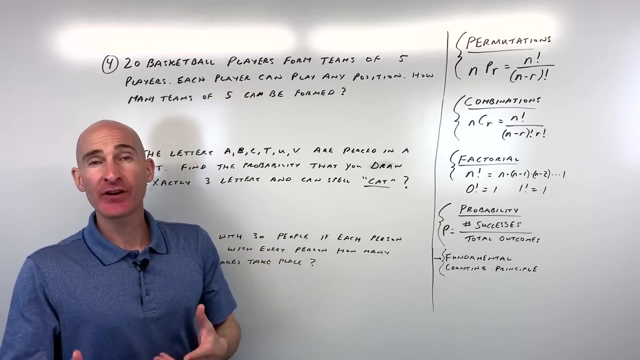 five players in each team, right? each player can play any position. how many teams of five can be formed? so what do you think for this one? when you form these teams of five people, does the order matter? well, in this case, because every player can play every other position, the order doesn't really. 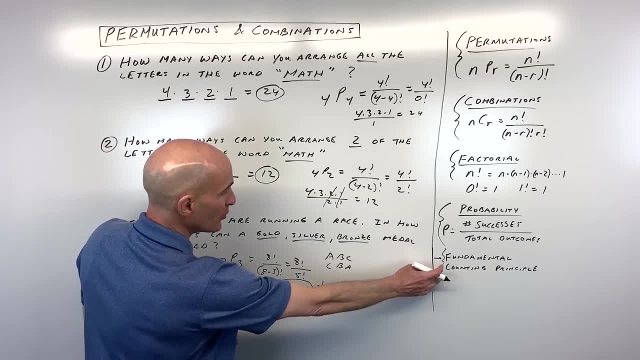 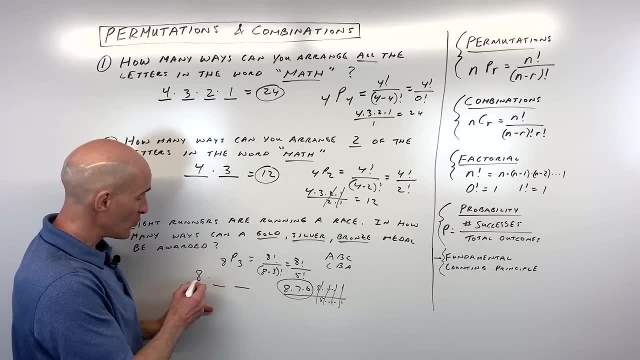 which makes sense, because if we were to use the fundamental counting principle here, we say: how many ways are there to award, like, a gold medal? Well, out of eight runners, there's going to be eight ways to do that, but once you award that gold medal, there's only seven runners. 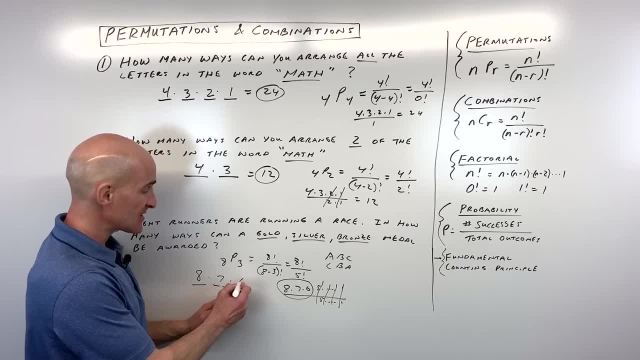 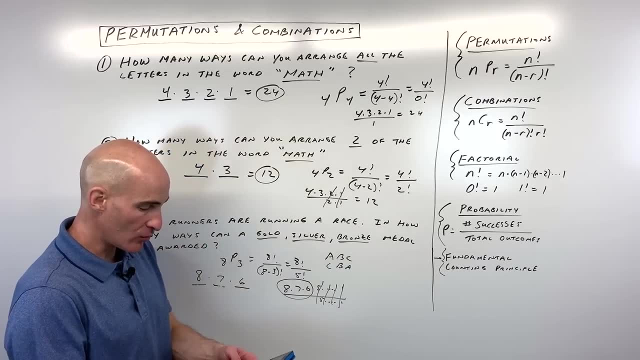 left to, you know, win that silver medal, right seven, and then six left for the bronze. So eight times seven times six, you can see we're getting the exact same result. and just to in case you're doing this on your own, let's get an answer here. That's three hundred and thirty six. 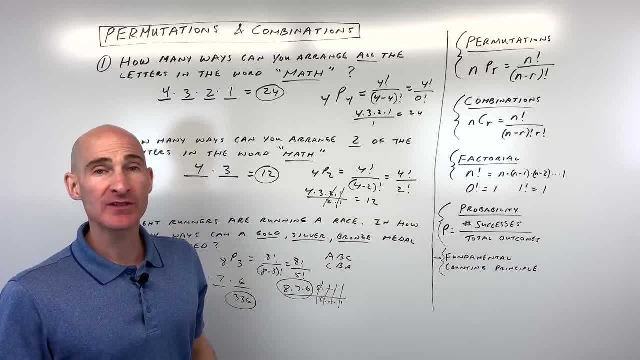 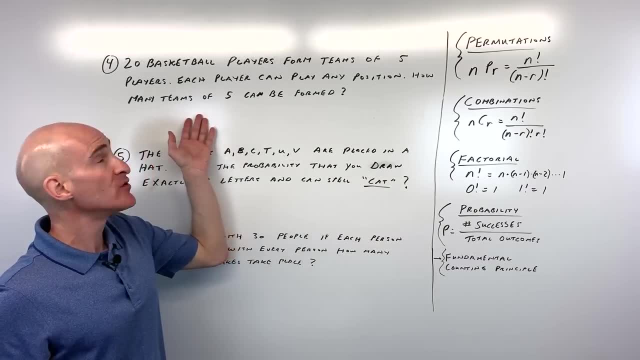 six different ways or outcomes. So we haven't gotten into any probability problems yet, but here we're just talking about the number of possible outcomes. Okay, number four. see if you can do this one. We've got 20 basketball players. form teams of five players in each team, right? 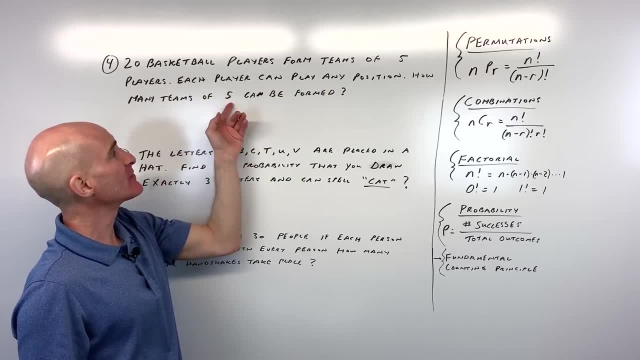 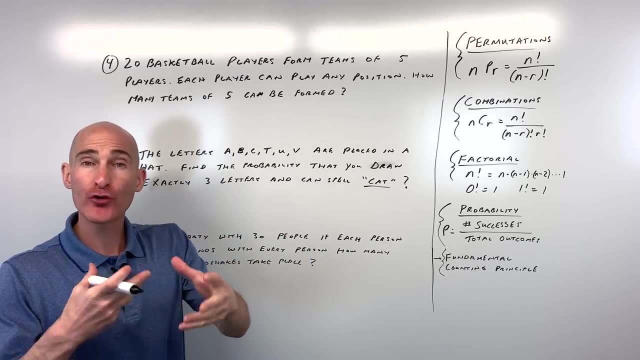 Each player can play any position. How many teams of five can be formed? So what do you think for this one? When you form these teams of five people, does the order matter? Well, in this case, because every player can play every other position, the order doesn't really matter. We're. 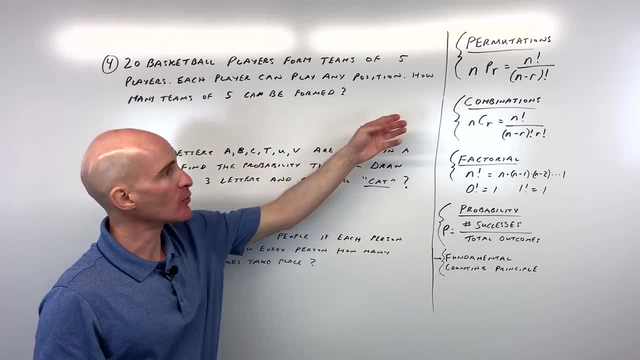 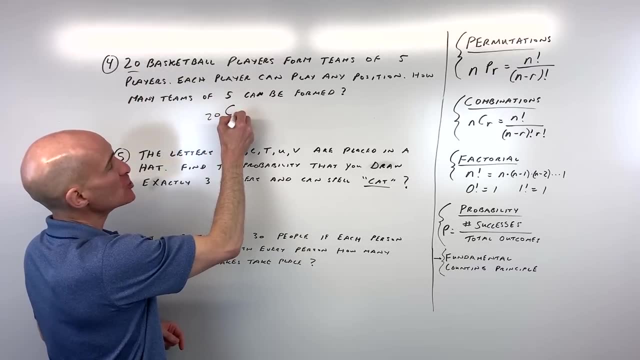 just looking at that particular group of five people. So, when the order doesn't matter, we're thinking combinations. okay, and in this case you can see, out of the 20 players we want to choose five of them where the order doesn't matter. So it's 20 combination 5, which, if you use the 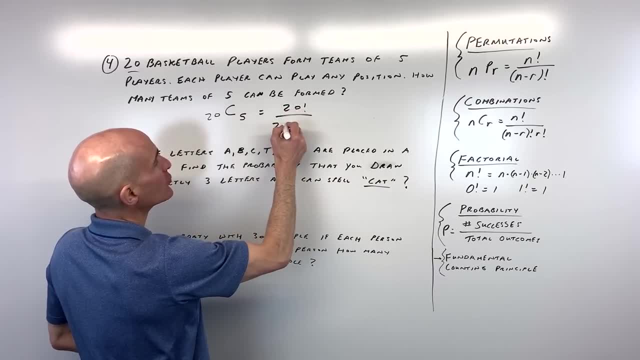 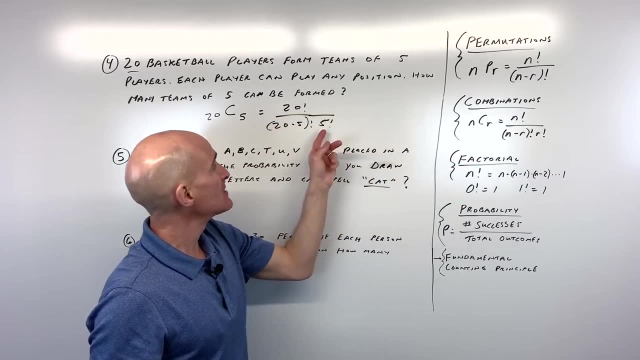 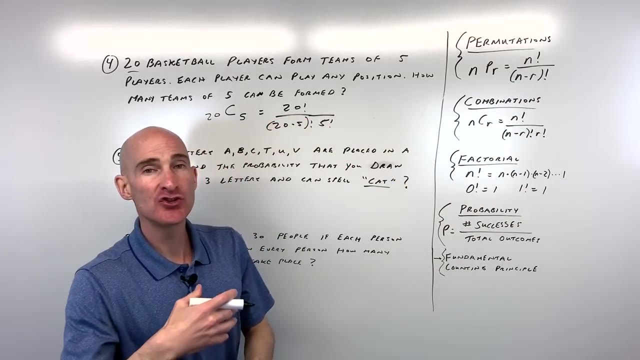 formula. here it's going to be 20 factorial over 20 minus 5 factorial- 5 factorial. Now notice this r value right here. See, the r value is: this is the only thing that's different between the permutation formula and the combination formula, and what this r factorial is doing is it's. 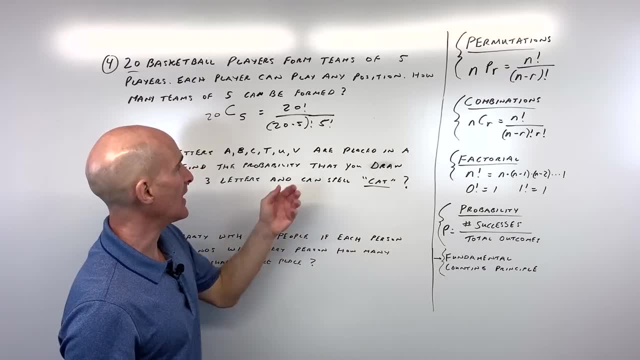 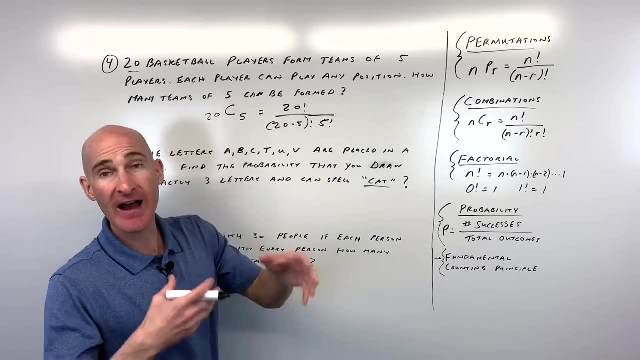 dividing out all the multiples, all the multiplicities, you could say So: 5 factorial, there's really 5 times 4 times 3 times 2 times 1.. There's 120 different ways of arranging five players, but they're all going to be on the same team, So you only count that team. 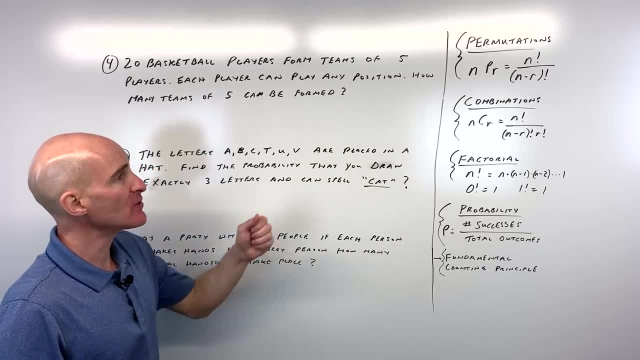 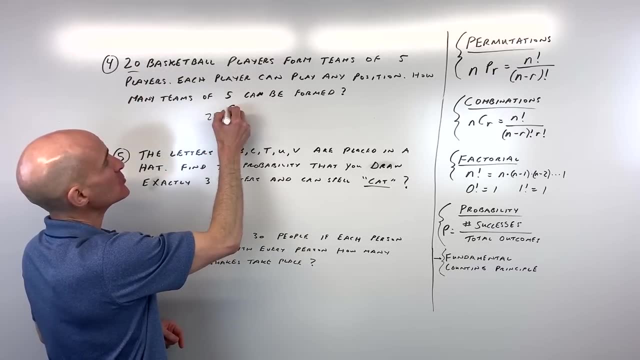 matter, we're just looking at that particular group of five people. so when the order doesn't matter, we're thinking combinations. okay, and in this case you can see: out of the 20 players we want to choose five of them where the order doesn't matter. so it's 20, combination five. 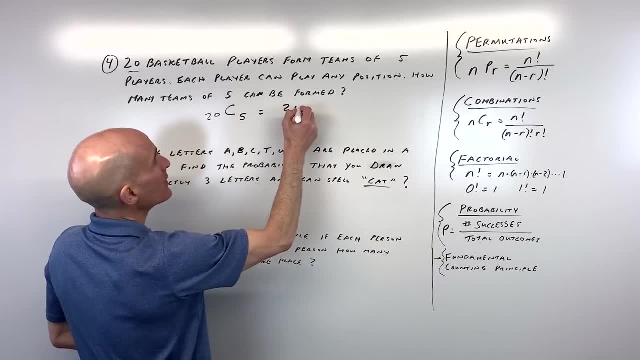 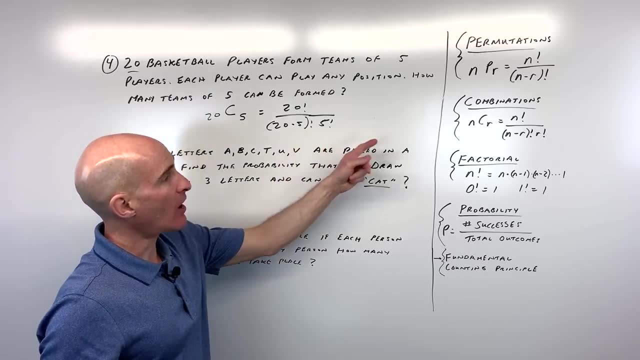 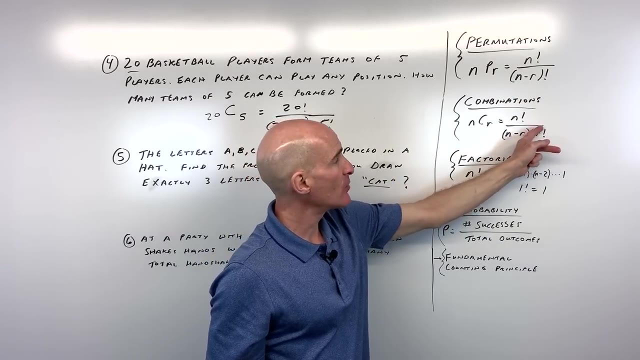 which, if you use the formula here, it's going to be 20 factorial over 20, minus five factorial, five factorial. now notice this r value right here. see, the r value is: this is the only thing that's different between the permutation formula and the combination formula. and what this r factorial is doing is it's dividing out all the multiples, all. 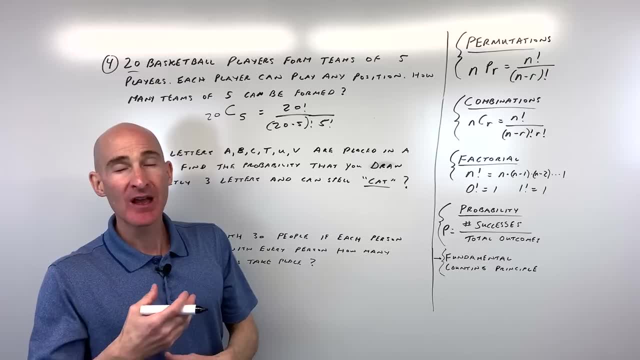 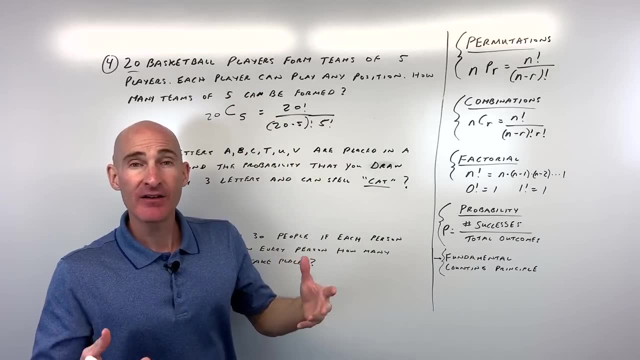 the multiplicities you could say so five factorial, there's really five times four times, three times, two times one. there's 120 different ways of arranging five players, but they're all going to be on the same team, so you only count that team once, not 120 times. so that's why we're dividing out. 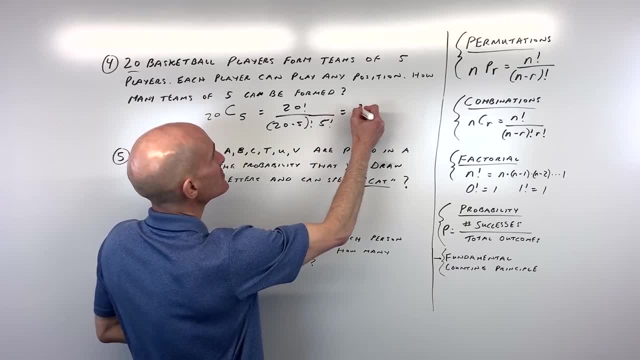 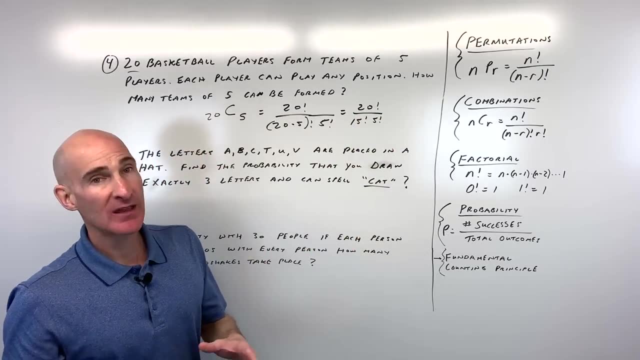 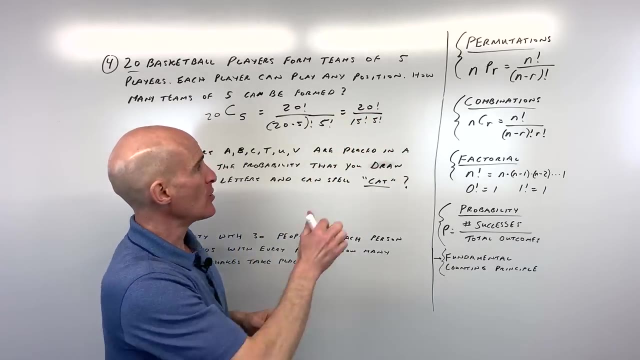 these multiplicities here. so if we simplify this further, this is going to be 20 factorial over 15 factorial times 5 factorial. and you don't want to make the mistake of saying, oh, this is like 75 factorial or 20 divided by 5, that's 4 factorial. it doesn't work that way. you have to actually 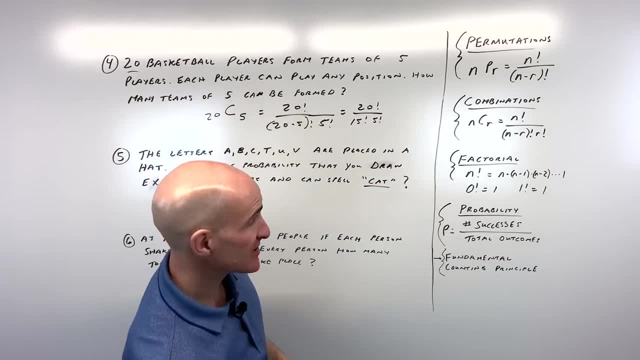 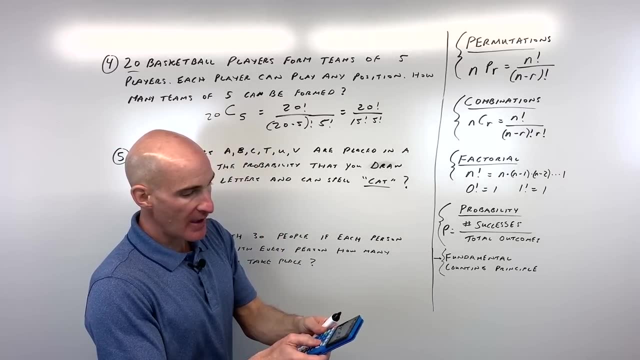 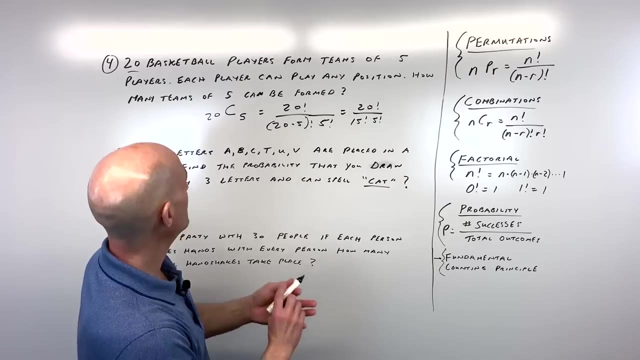 expand this out 20 times, 19 times, 18 times 17, etc. or you can use this combination key on your calculator. it's under the probability menu, so i'm going to do 20 math probability. go down to the combination, so 20, c5 and this is coming out to 15, 504, 15 504 different ways that you could form these five. 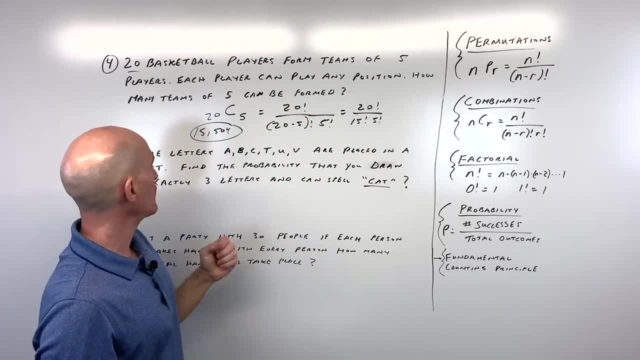 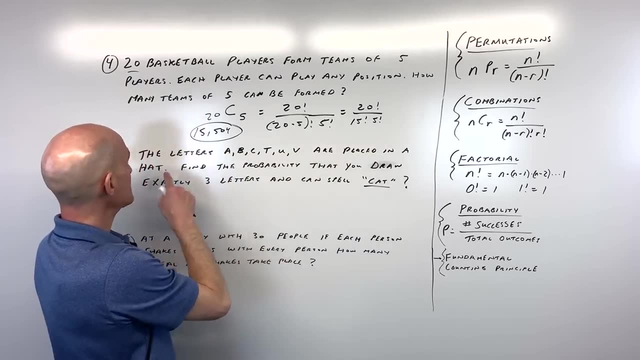 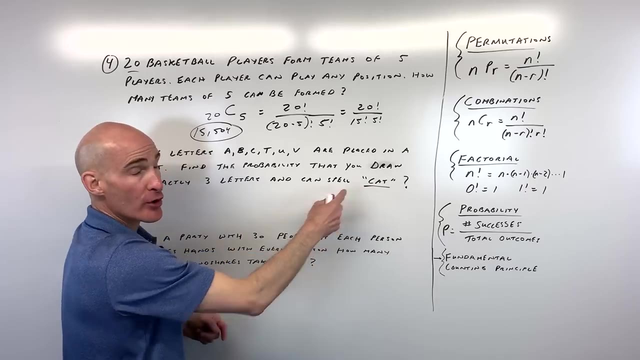 player teams out of 20 basketball players. okay. so for number five, a little different problem. here the letters a, b, c, t, u and v are all placed in the hat. okay, find the probability that you draw exactly three letters and you can spell the word cat, okay. so now we're transitioning a little bit to talking about probability, and so the definition. 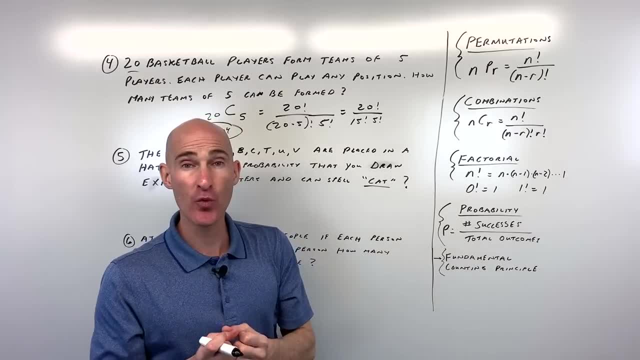 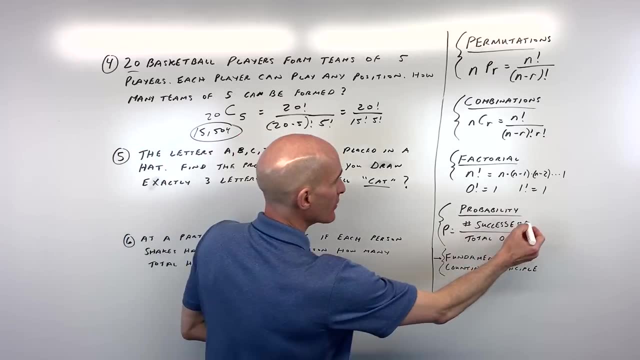 of probability is the number of successes, meaning the number of things that you want, divided by the total possible outcomes. okay, so it's. it's like if you were to spin a spinner and you say: what's the probability, i land on an odd number: one, two, three, four. well, there's two odd. 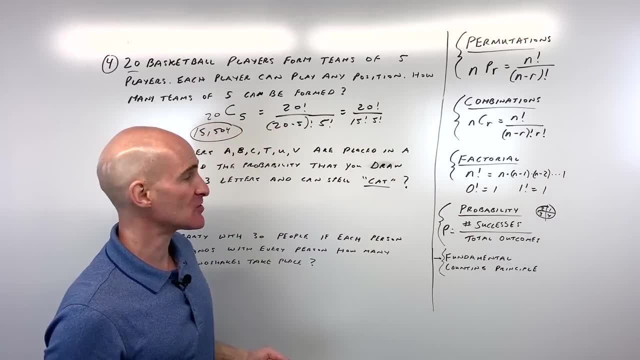 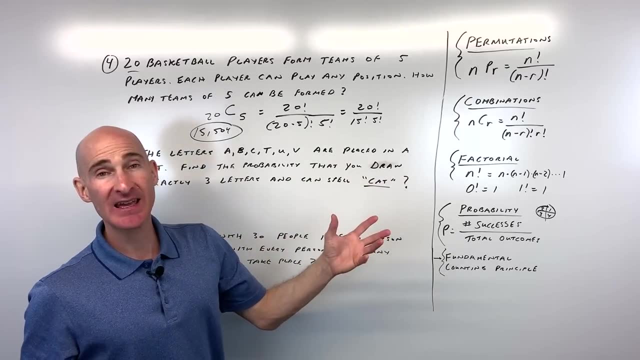 out of four possible. so it'd be two over four, which is one half. that's your probability. so it's what you want, or success is out of the total. so in this case, what do we want? we want the letters c, a and t, right? so we're basically saying: out of those. 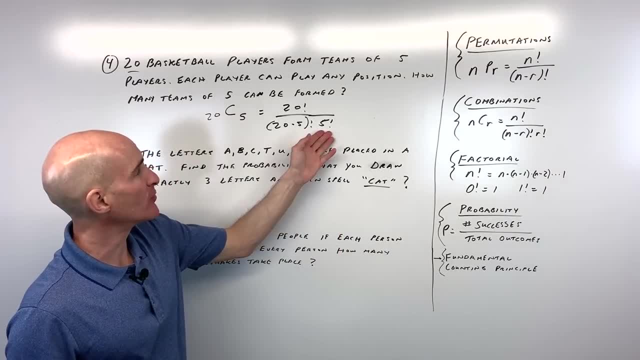 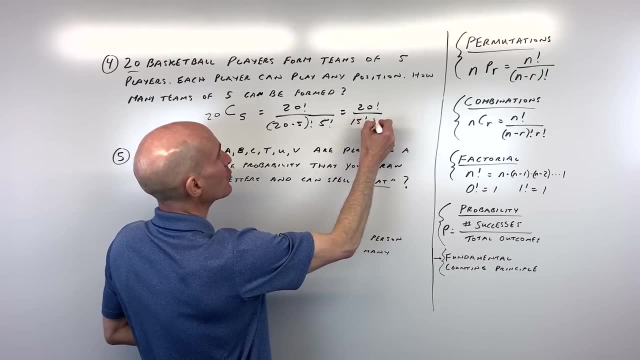 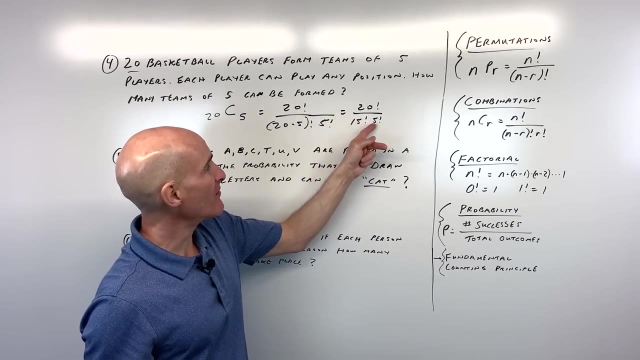 once, not 120 times. So that's why we're dividing out these multiplicities here. So if we simplify this further, this is going to be 20 factorial over 15 factorial times 5 factorial, And you don't want to make the mistake of saying, oh, this is like 75 factorial or 20 divided by 5,. 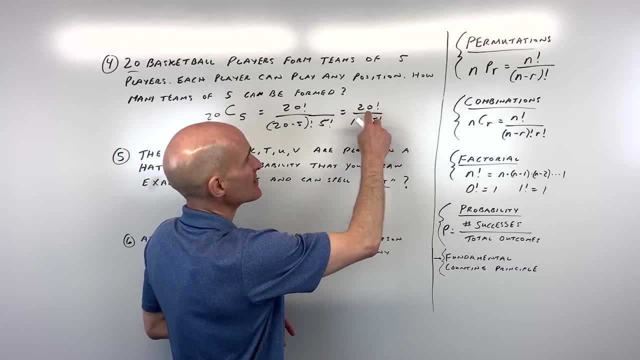 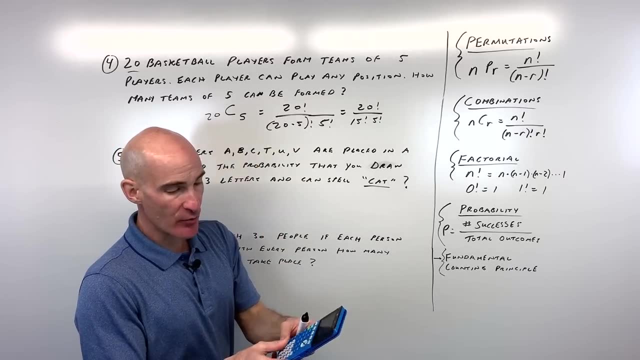 that's 4 factorial. It doesn't work that way. You have to actually expand this out: 20 times 19 times, 18 times 17, etc. Or you can use this combination key on your calculator. It's under the probability menu, So I'm going to do 20 math probability go down to the combination. So 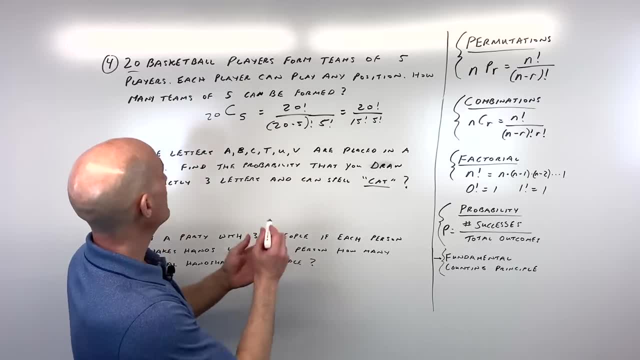 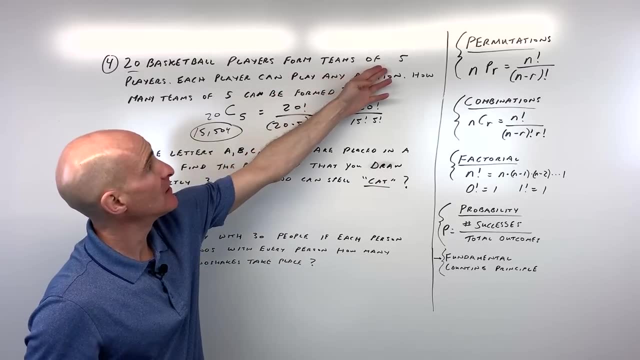 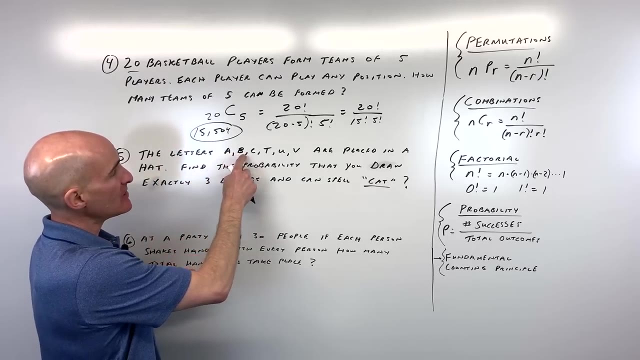 20 c5 and this is coming out to 15,504.. 15,504 different ways that you could form these five player teams out of 20 basketball players. Okay, so for number five, a little different problem. here the letters a, b, c, t, u and v are all placed in the hat. Okay, find the probability that you draw. 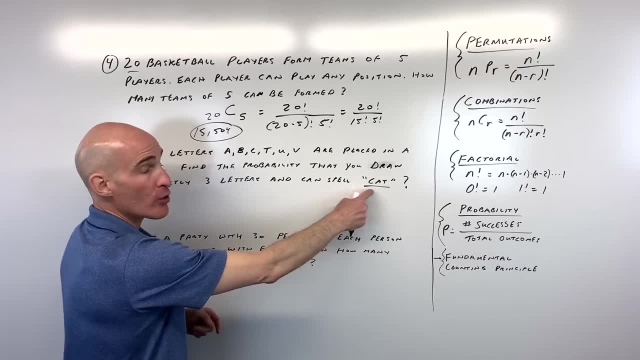 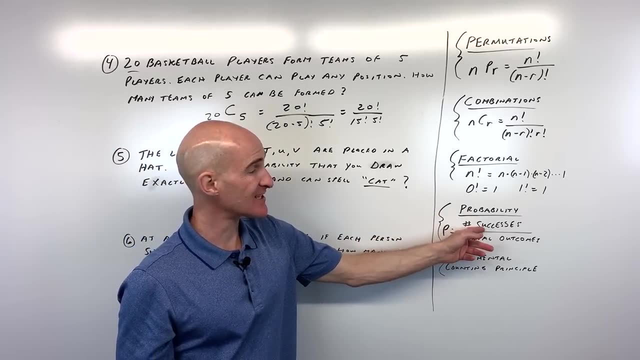 exactly three letters and you can spell the word cat. Okay, so now we're trying to transition a little bit to talking about probability, And so the definition of probability is the number of successes, meaning the number of things that you want, divided by the total. 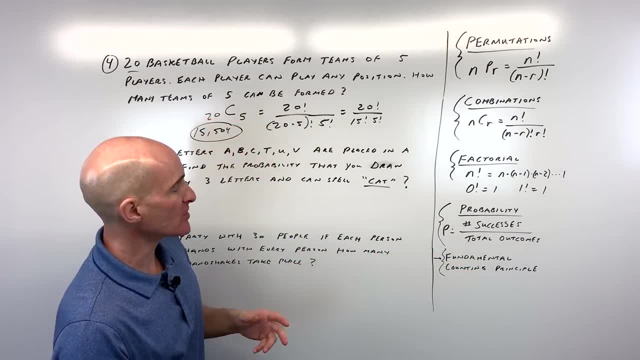 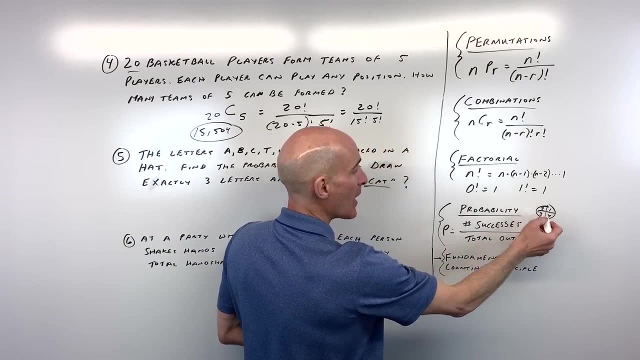 possible outcomes. Okay. so it's like if you were to spin a spinner and you say what's the probability, I land on an odd number: One, two, three, four. Well, there's two odd out of four possible, So it'd be two over four, which is one half. That's your probability. So it's what you. 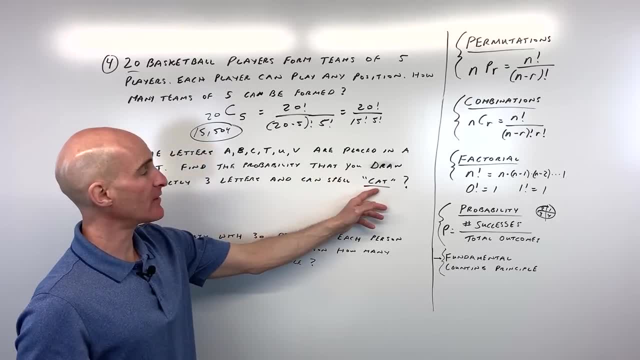 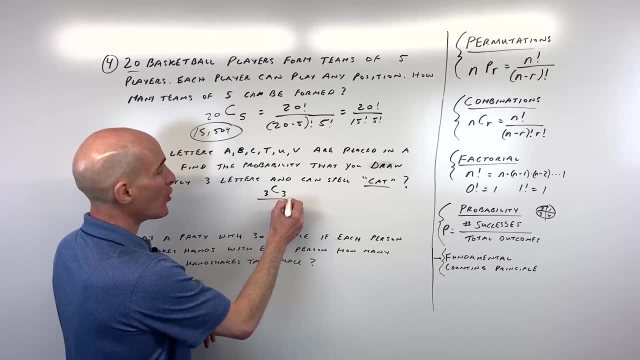 want or successes out of the total. So in this case, what do we want? We want the letters a and t, right? So we're basically saying, out of those three letters that we want, how many ways are there to choose all three? And out of not 20 letters but six letters? 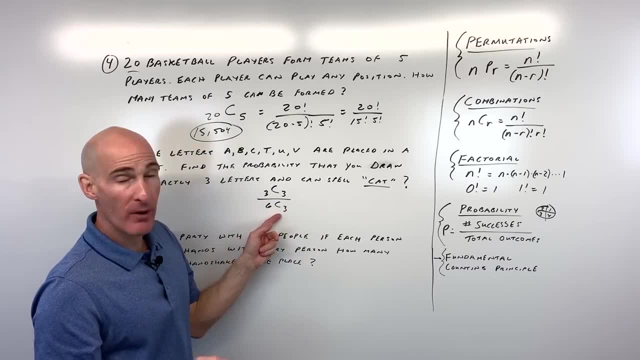 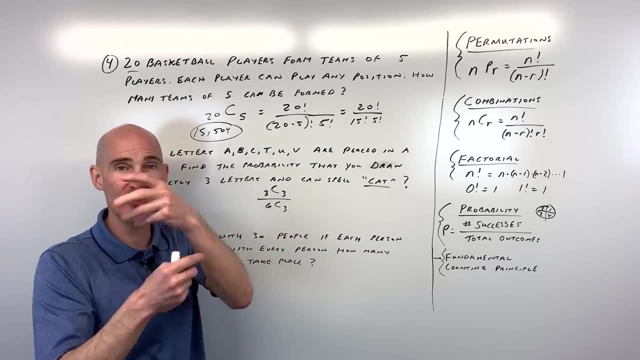 how many ways are there of choosing three letters? So this gives us the total possible outcomes of the ways of choosing three letters, where the order is not important, Because when you get these letters in your hand you can arrange them any way you want. So we don't want to count. 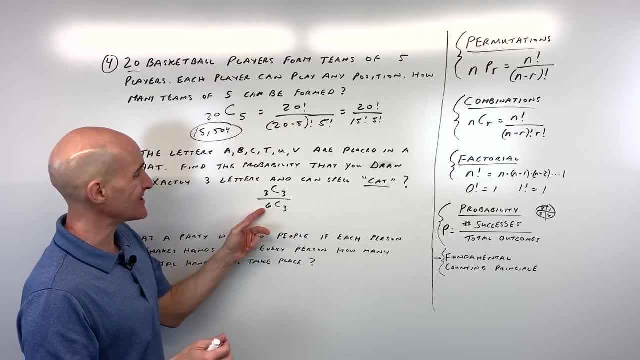 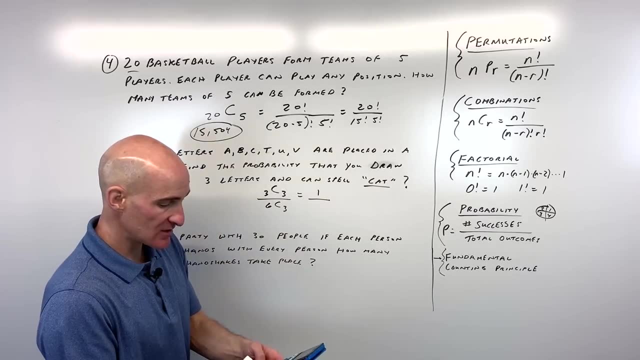 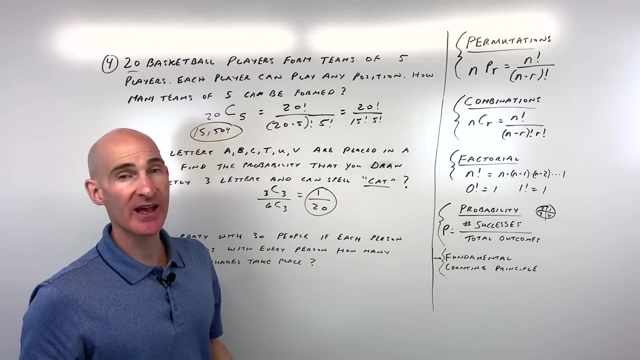 the ordering is different. We want to just count it as one group of three letters out of six, And so 3c3 is going to equal one and 6c3, let's see what that comes out to. six combination three is 20.. So you have a 1- 20th chance of being able to do this Now. this kind of makes sense because 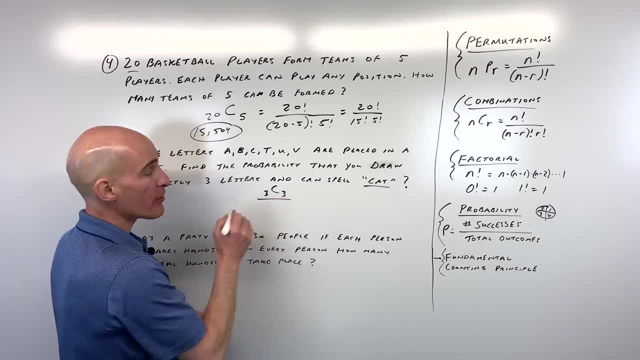 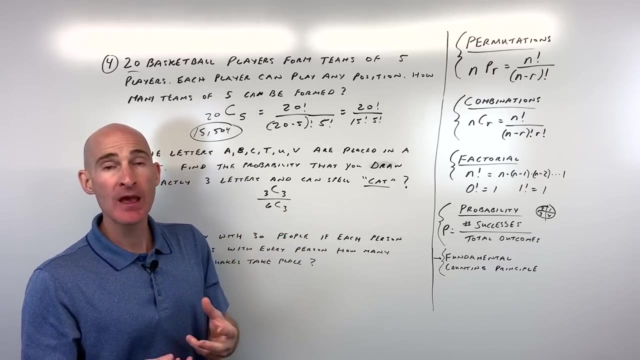 three letters that we want, how many ways are there to choose all three and out of not 20 letters but six letters, how many ways are there of choosing three letters? so this gives us the total possible of outcomes of the ways of choosing three letters, where the order is not important, because when you 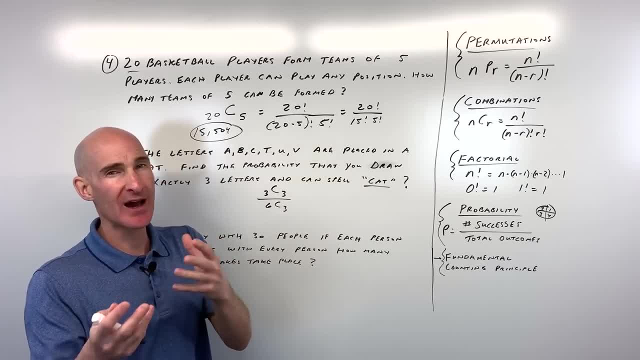 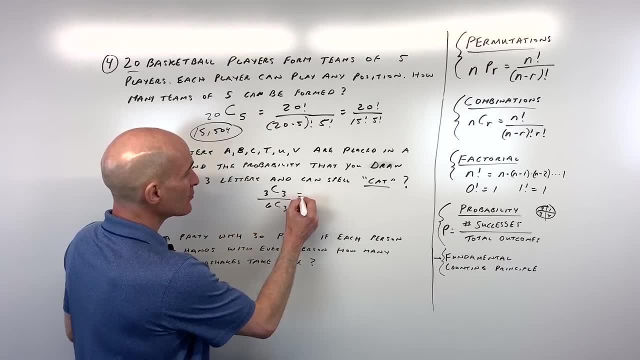 get these letters in your hand. you can arrange them into a new order as a result. you can make a new order any way you want. so we don't want to count them. the ordering is different. we want to just count it as one group of three letters out of six, and so 3c3 is going to equal 1 and 6c3. let's see what. 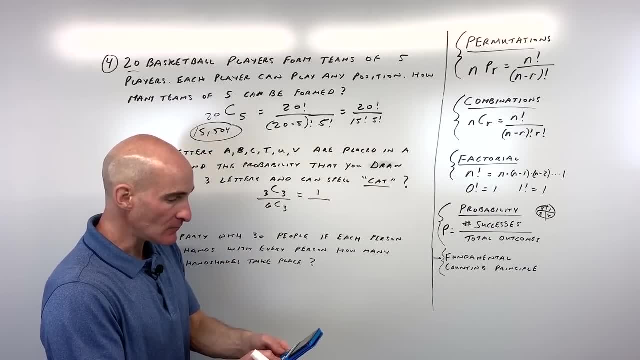 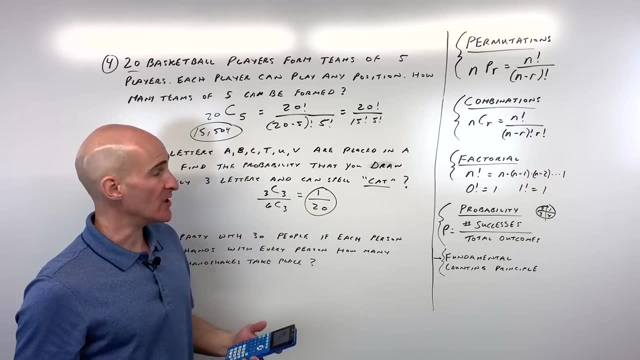 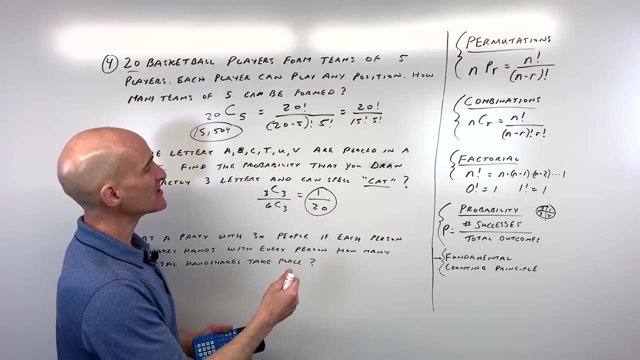 that comes out to six combination. three is 20. so you have a 1- 20th chance of being able to do this. now. this kind of makes sense because out of three, how many ways are choosing all three? well, there's only going to be one way of doing that. or you could say: you know, there's only going to be one. 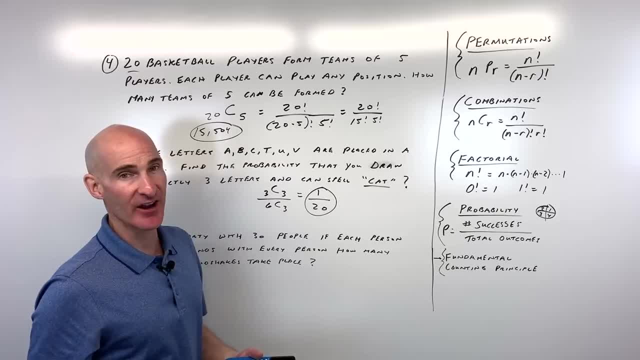 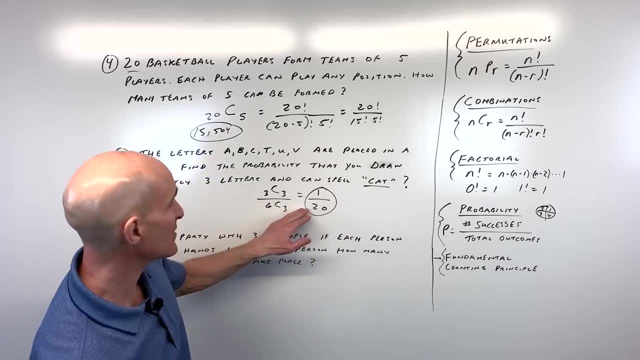 way of getting the success of drawing these three letters cat right out of the 20 different ways of drawing three letters out of out of the six. so different ways to think about it. but combinations because the order doesn't matter. probability because we're trying to figure out the chance. 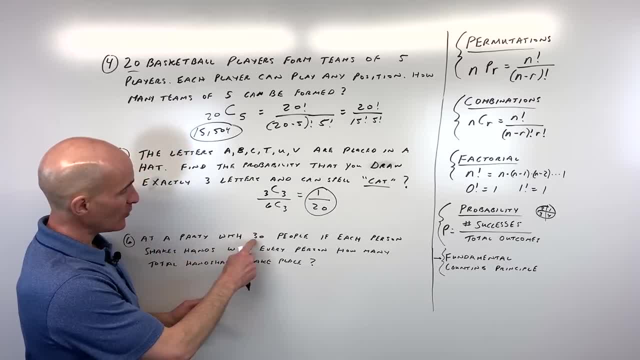 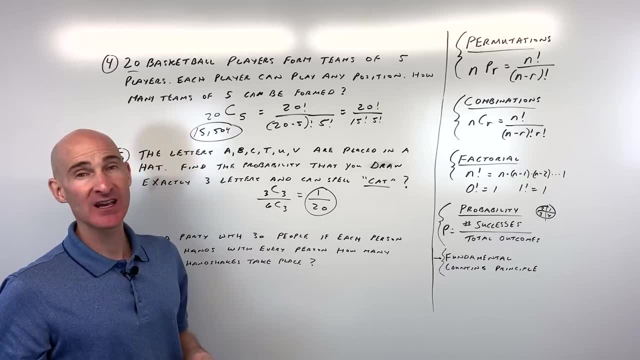 that this occurs. number six: here it says at a party with 30 people. if each person shakes hands with every person, how many total handshakes take place? okay, this is kind of a common problem here. so if you're at a party with 30 people, how many total handshakes take place? 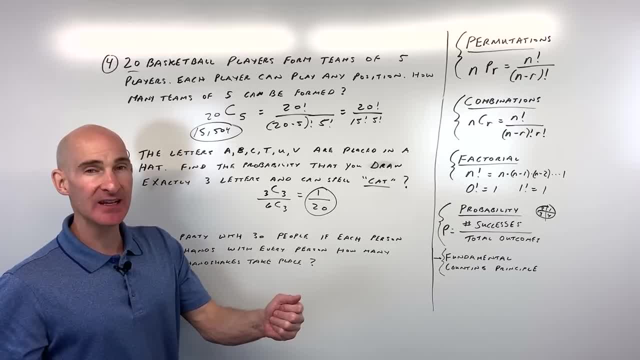 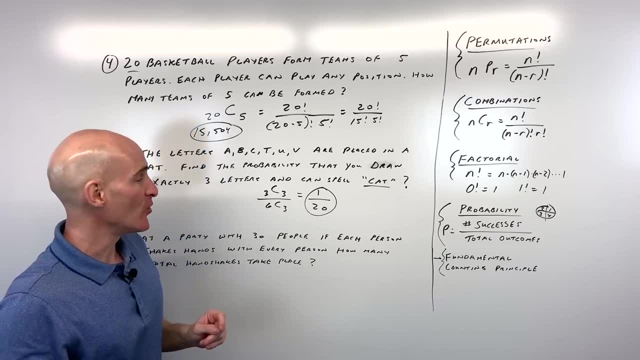 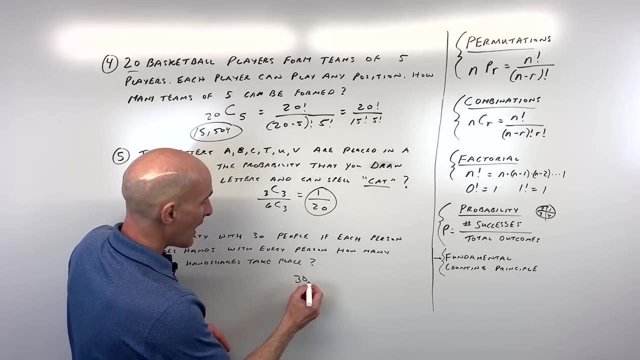 but imagine you're at a party and you're trying to shake everybody's hand. see, the thing is, when two people shake hands, how many handshakes is that? well, it's just one, right? so you don't want to double count. and so what we're thinking here is: we're thinking of: out of 30, how many ways are? 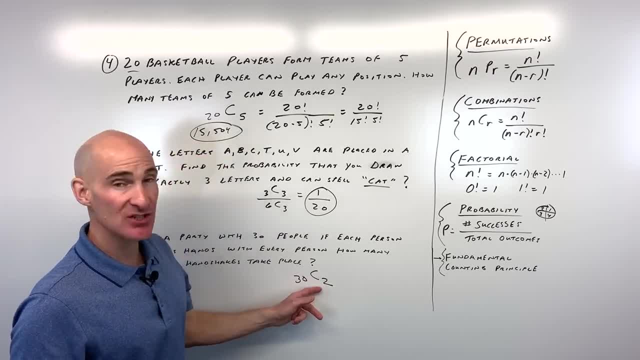 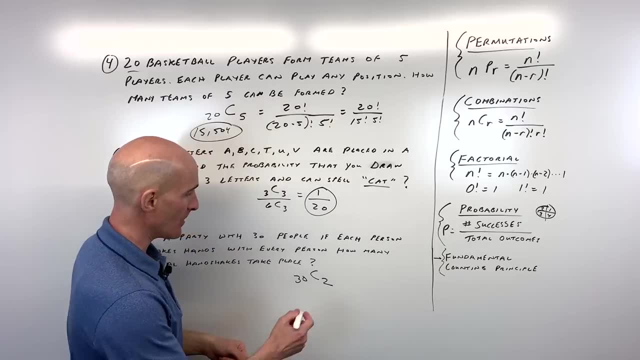 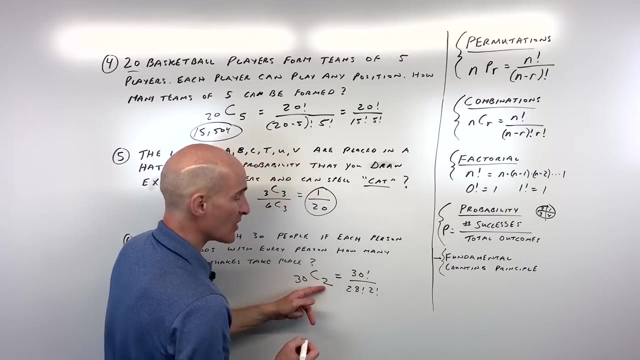 they're choosing two. okay, so 30 c2. so a and b, b and a, that's the same one handshake. so that's why we're not treating it like a permutation, but rather a combination. and 30- c2 is the same one. c2 is going to be 30 factorial over 30 minus 2, which is 28 factorial times 2 factorial. so let's. 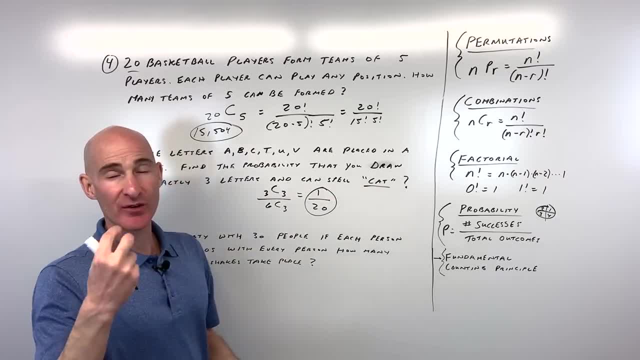 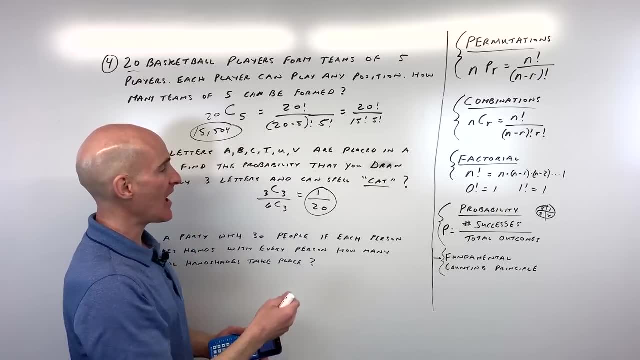 out of three. how many ways are choosing all three? Well, there's only going to be one way of doing that. Or you could say: you know, there's only going to be one way of getting the success of drawing these three letters cat right out of the 20 different ways of drawing three letters out. 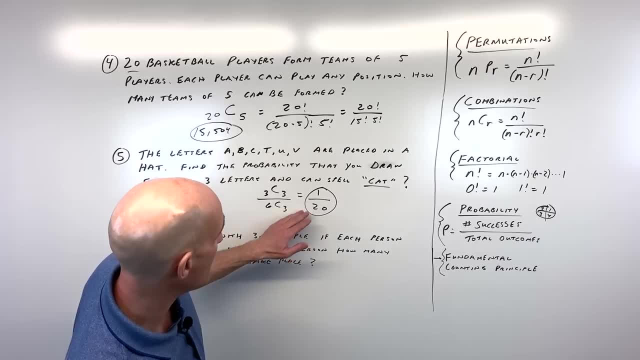 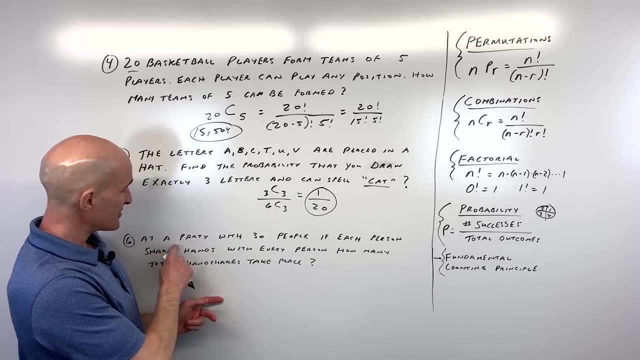 of out of the six. So different ways to think about it. but combinations because the order doesn't matter. Probability, because we're trying to figure out the chance that this occurs. Number six: here it says: at a party with 30 people, if each person shakes hands with every person. 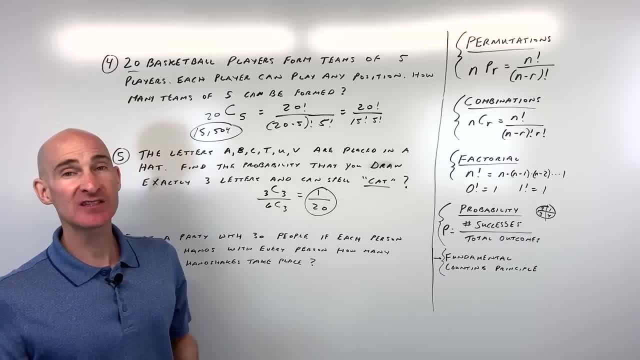 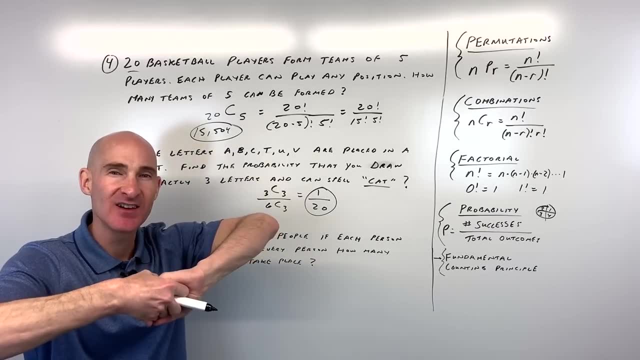 how many total handshakes take place? Okay, this is kind of a common problem, but imagine you're at a party and you're trying to shake everybody's hand. See, the thing is, when two people shake hands, how many handshakes is that? Well, it's just one, right. 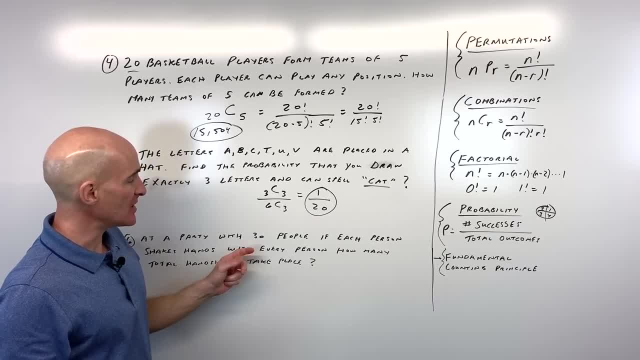 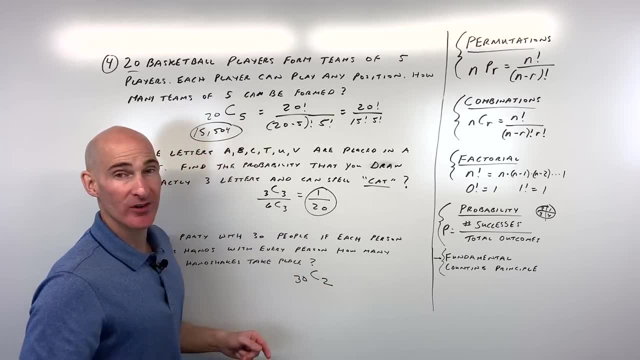 So you don't want to double count, and so what we're thinking here is we're thinking of: out of 30, how many ways are there choosing two? Okay, so 30, c, 2. So a and b, b and a, that's the same one. 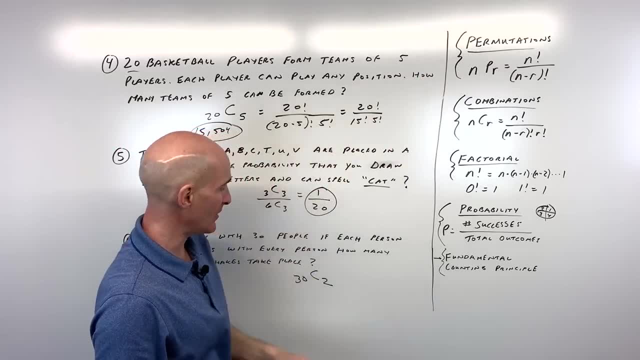 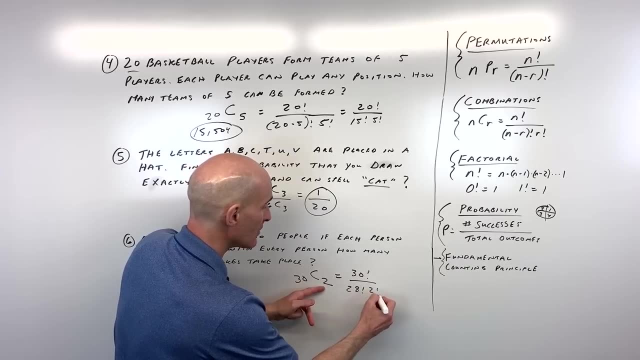 handshake. so that's why we're not treating it like a permutation but rather a combination. And 30 c- 2 is going to be 30 factorial over 30 minus 2, which is 28 factorial times 2 factorial. So let's go ahead and do that on the calculator, that's. 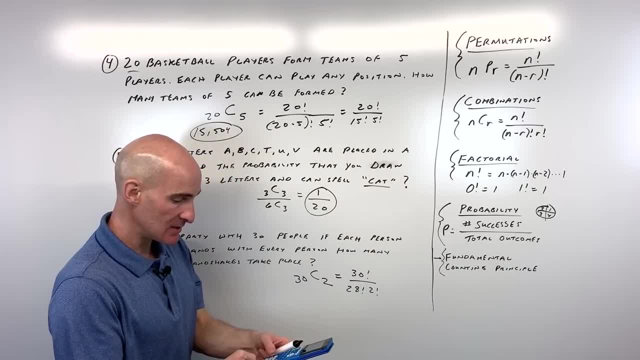 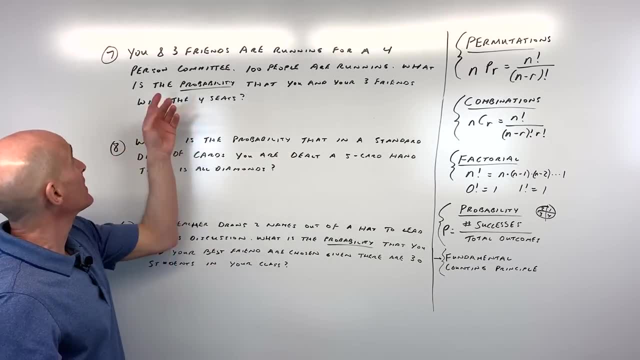 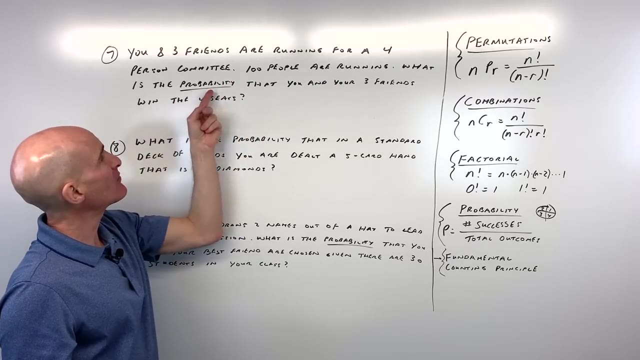 let's see 30. math c: 2.. All right, so that's 435 handshakes. Okay, number seven. let's see if you can do this one. it says you and three friends are running for a four person committee. 100 people are running. what is the probability that you? 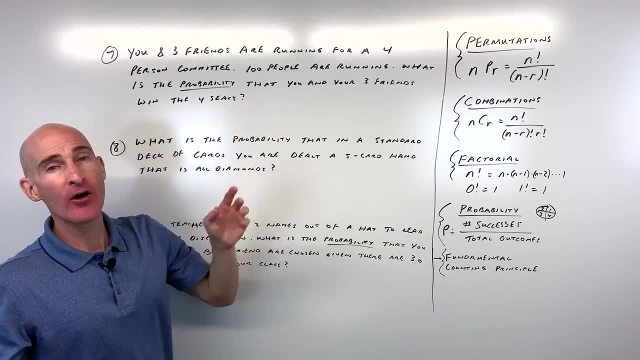 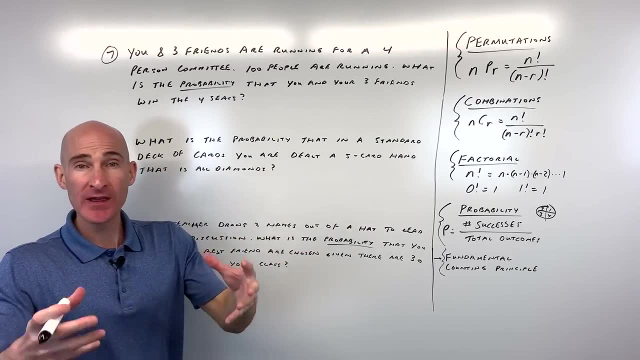 and your three friends win the four seats. Okay, so interesting question. so the first thing is, we're trying to basically figure out that you and your three friends, that's four people, win the four seats. There's only going to be one way that that can happen, or you can think of this as out. 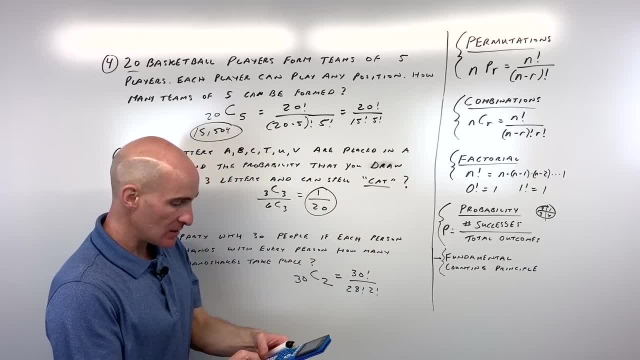 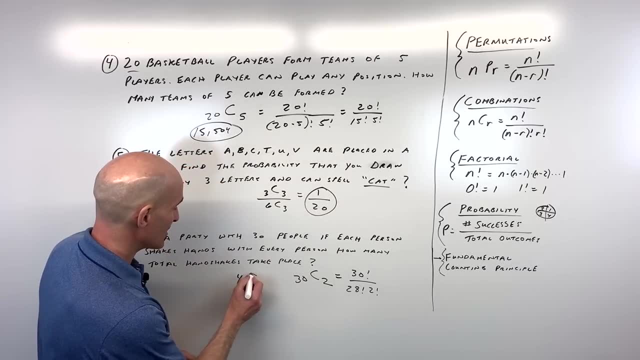 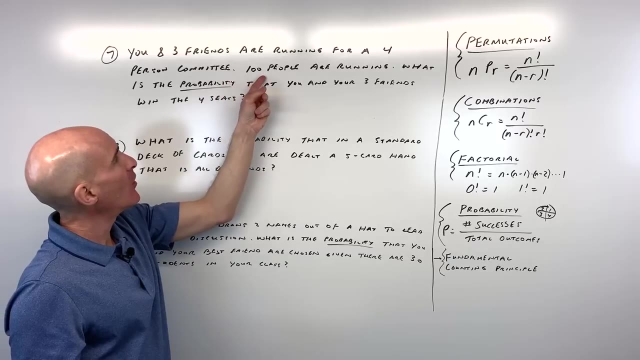 go ahead and do that. on the calculator. that's: uh, let's see 30 math c2. all right, so that's 435 handshakes. okay, number seven. let's see if you can do this one. it says you and three friends are running for a four-person committee. 100 people are running. what is the probability that you and 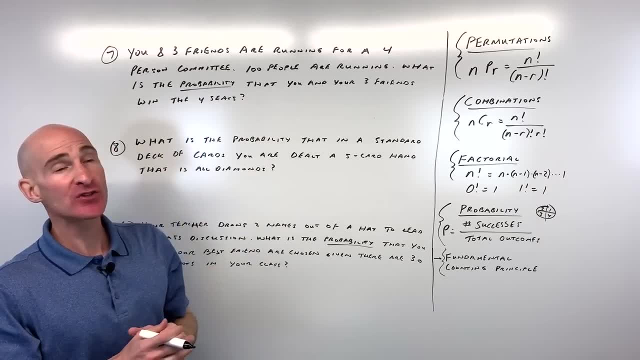 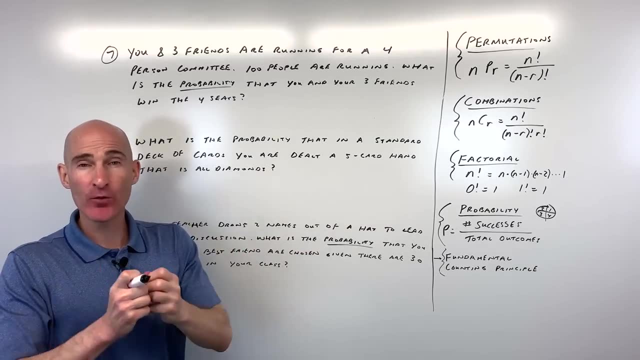 your three friends will have a four-person committee, win the four seats, okay, so interesting question. so the first thing is: we're trying to basically figure out that you and your three friends, that's four people, win the four seats. there's only going to be one way that that can happen, or you could think of this as, out of the four people that you 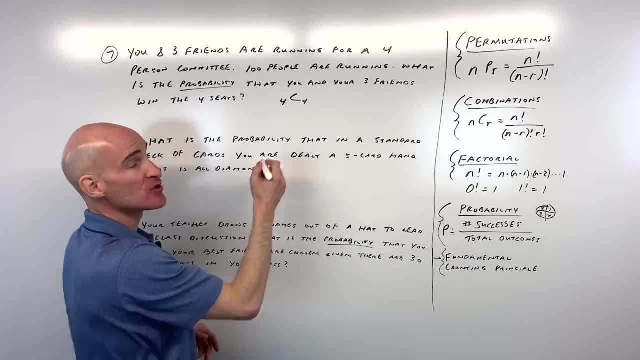 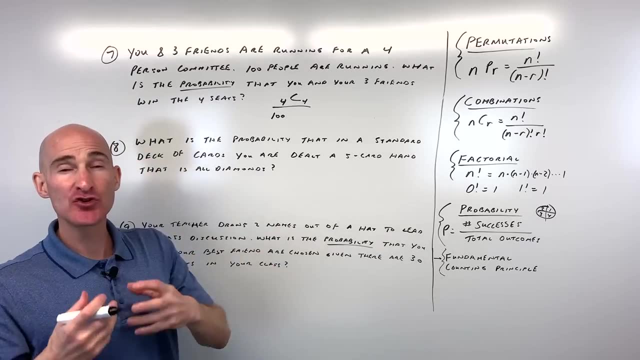 want to win. you know that you're a group of four. how many ways are they choosing all four? so that's only going to be one way. but then, out of a hundred people, how many ways are there to choose four for this committee? now, how do i know that it's combinations and not permutations? 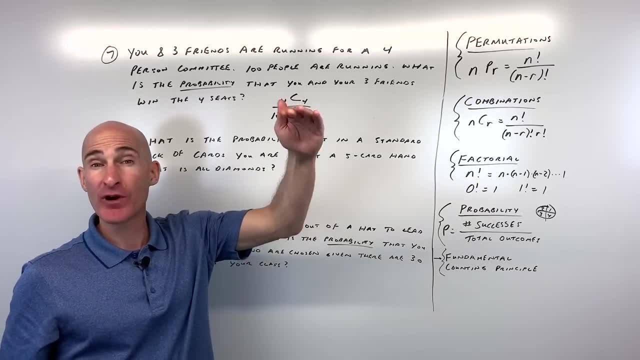 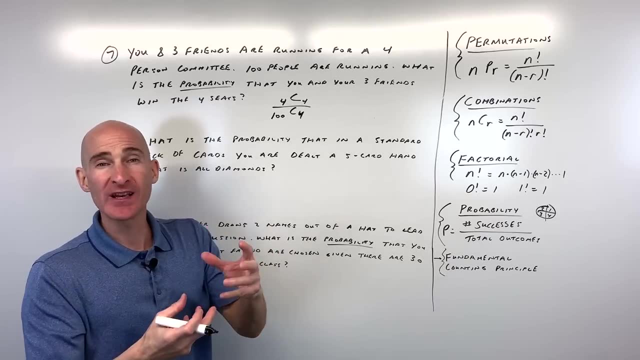 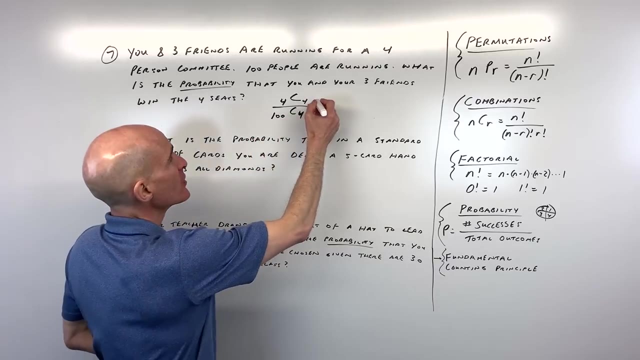 so when you're talking about a committee, it's not like there's a president, vice president, secretary, treasurer. all the positions are basically the same. so when you interchange the, the ordering, it doesn't really matter. it's the same committee. so you don't want to count those as separate uh outcomes. that's why we're using combinations. so here we said four. 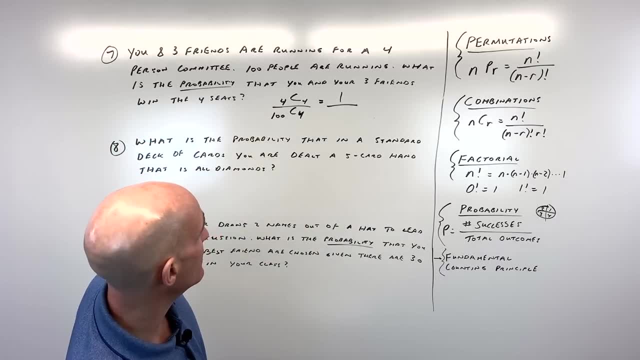 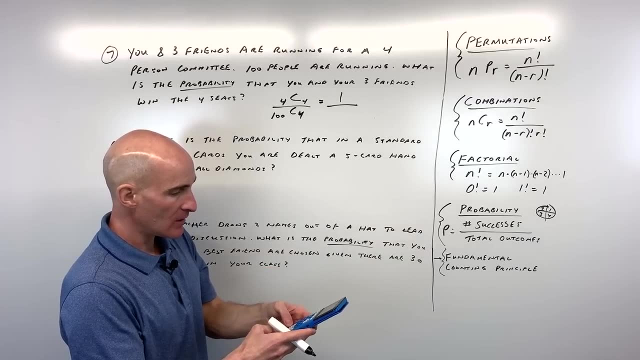 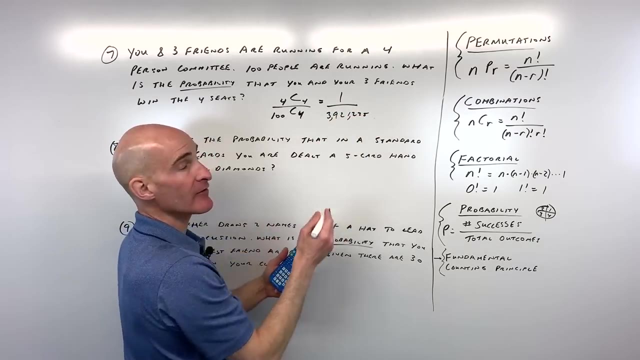 c4, there's only going to be one way that you and your three friends win, and then how many ways are there are? choosing four out of a hundred. let's see what a hundred c4 is. combination four, that's a big number. here we have three, nine, two, one, two, two, five, so one out of about almost four million. okay, so, uh, slim chance. 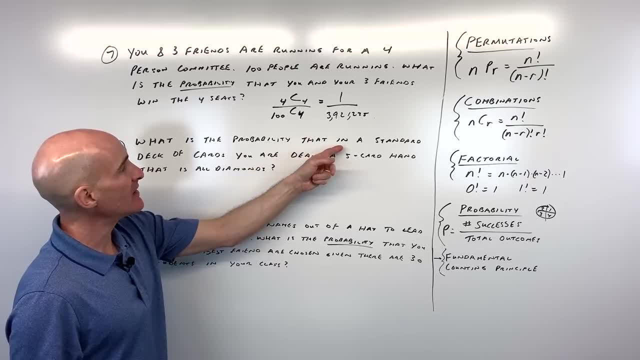 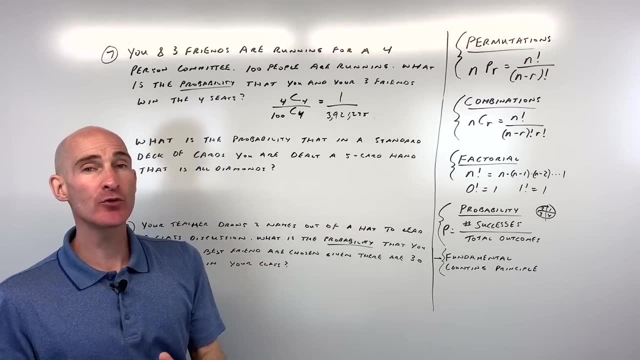 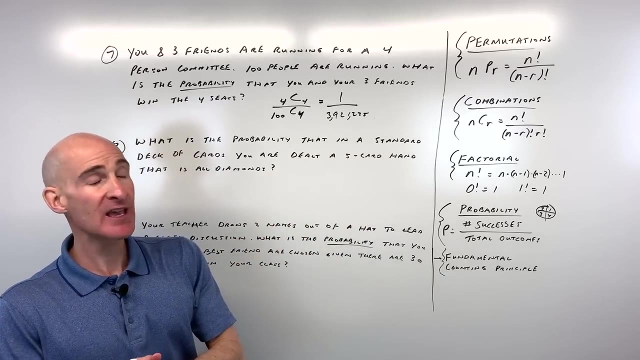 right number eight. now it says: what is the probability? then in a standard deck of cards, you are dealt a five card hand, that's all diamonds. okay, so you have to be familiar with cards to do this problem. but you want to be dealt a five card hand, that's all diamonds. so in this case we're. 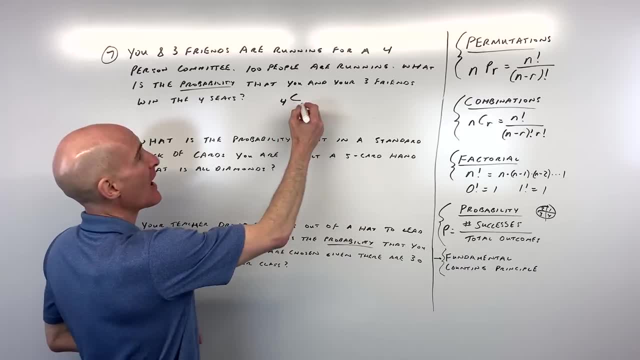 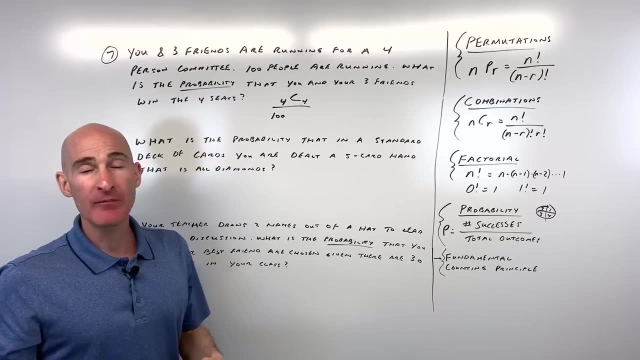 of the four people that you want to win, you know that you're a group of four. how many ways are there of choosing all four? That's only going to be one way. But then, out of a hundred people, how many ways are there to choose four for this committee? 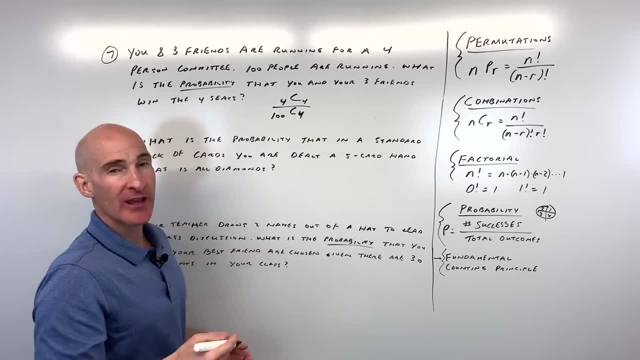 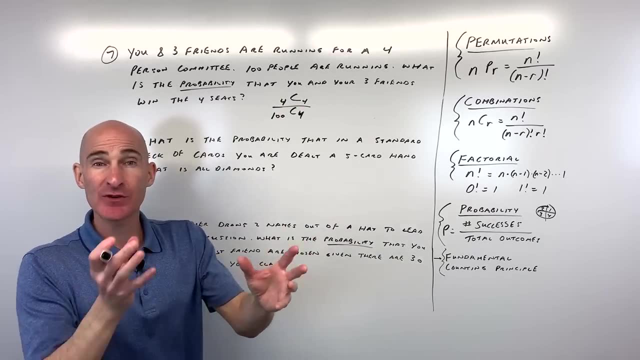 Now how do I know that it's combinations and not permutations? When you're talking about a committee, it's not like there's a president, vice president, secretary, treasurer. all the positions are basically the same. So when you interchange the ordering, it doesn't really matter. it's the same committee. 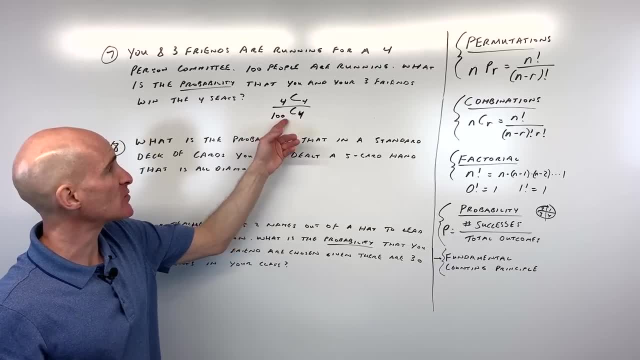 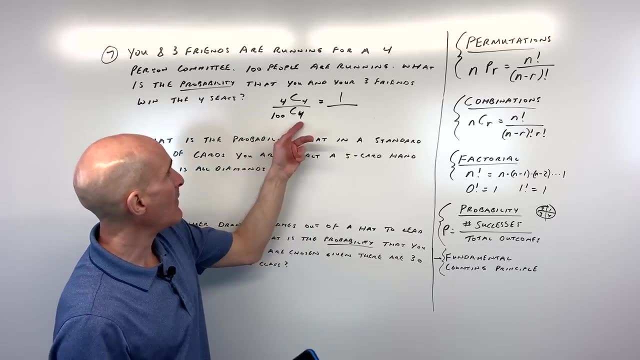 So you don't want to count those as separate outcomes. that's why we're using combinations. So here we said 4C4, there's only going to be one way that you and your three friends win. and then how many ways are there of choosing four out of a hundred? 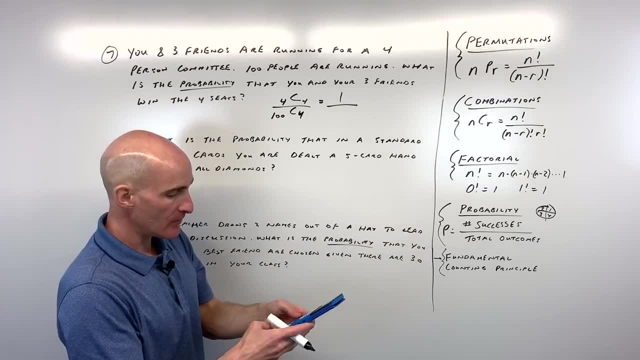 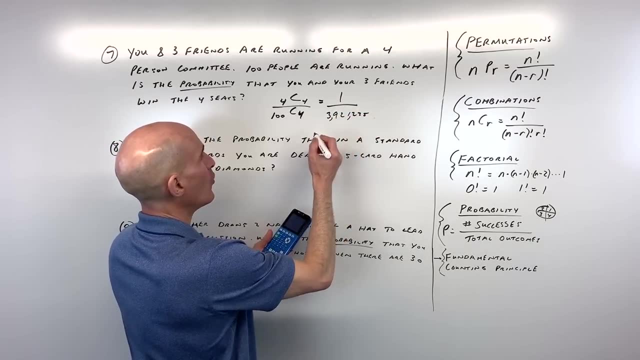 Let's see what a hundred C4 is. combination four, That's a big number. here we have three, nine, two, one, two, two, five, So one out of about almost four million. Okay, So slim chance, right. 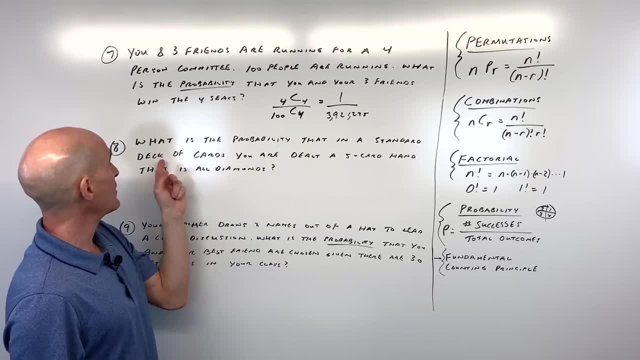 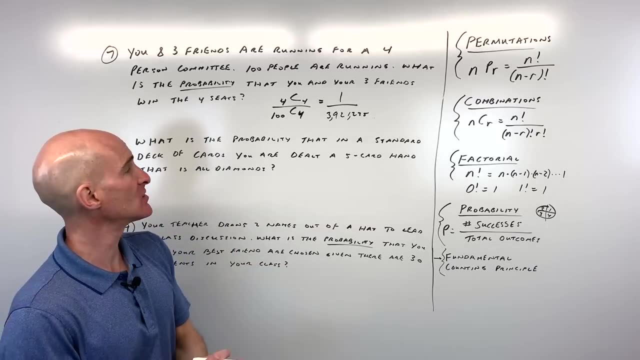 Number eight. now it says: what is the probability that in a standard deck of cards you are dealt a five card hand. that's all diamonds, Okay, so you have to be familiar with cards to do this problem. but you want to be dealt. 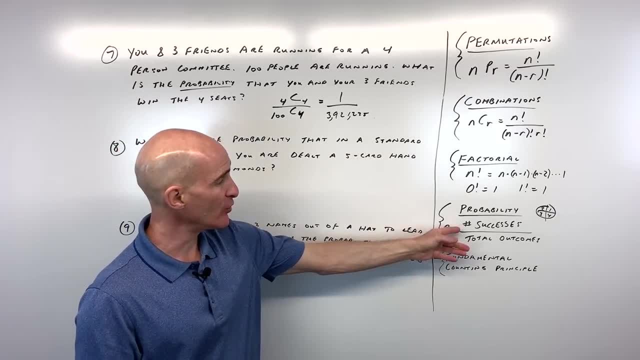 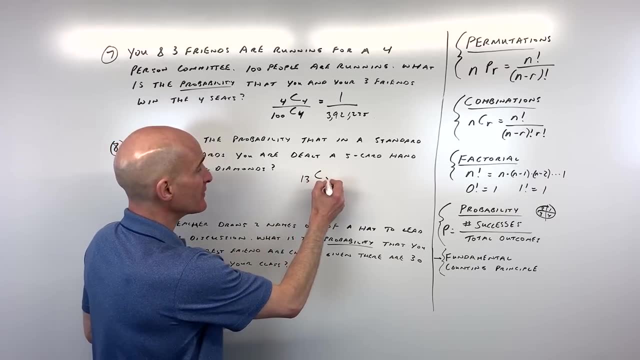 a five card hand. that's all diamonds. So in this case we're thinking about probability. what's the number of successes? Well, out of the 13 diamonds, how many ways are they choosing five? So when you do the combinations, this is how many are in that group. 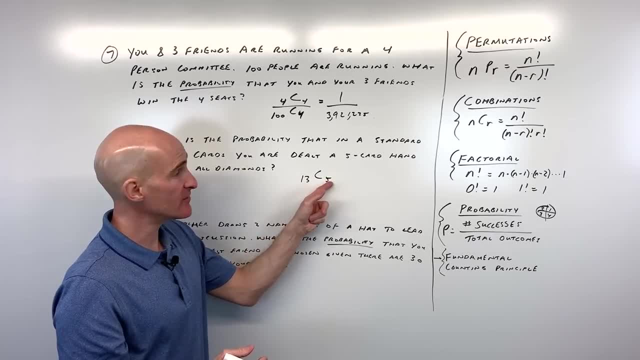 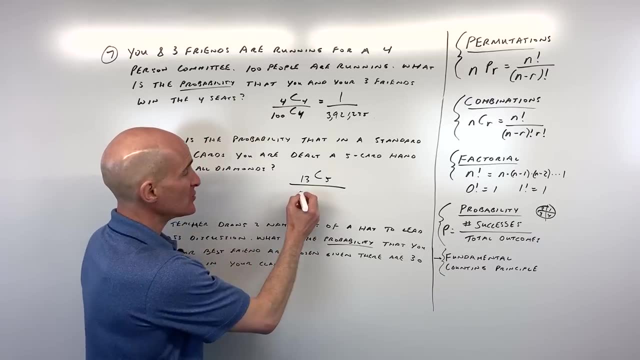 Of what you want, the 13 diamonds, but you're trying to choose five out of that 13,. so how many ways could that occur? But it's probability divided by the total number of outcomes. well, there's 52 cards in a standard deck. how many ways are they choosing five of those 52 cards where the 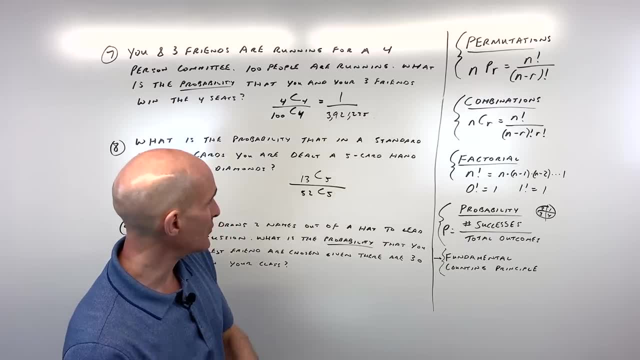 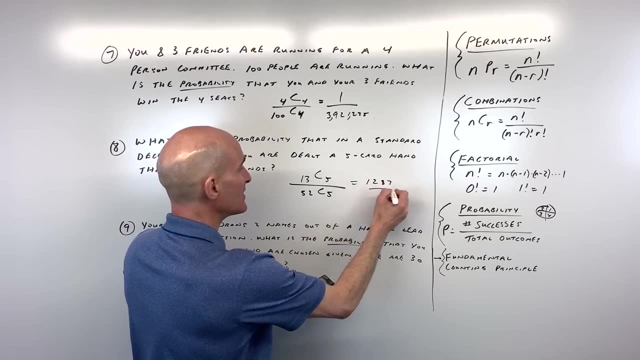 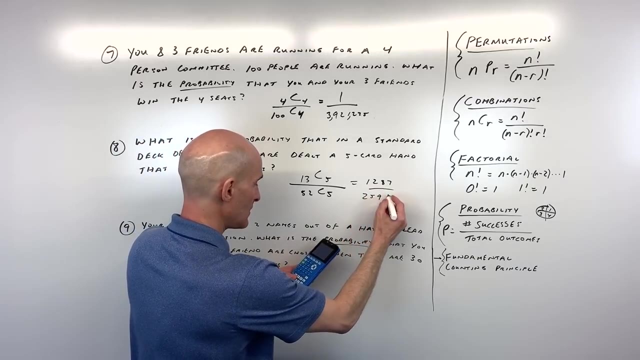 order doesn't matter, So again combinations. So let's see what that comes out to. so 13 combination five- okay is 1,287, and 52 combination five. That is a big number here: 2598960.. 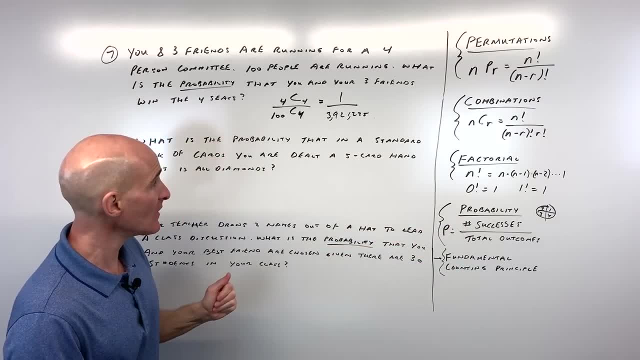 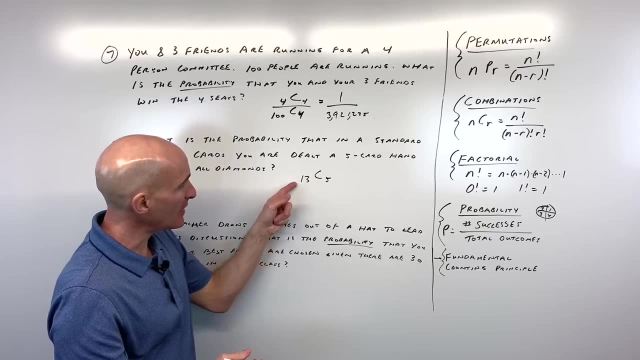 thinking about probability. what's the number of successes? well, out of the 13 diamonds, how many ways, they're choosing five. so when you do combinations, this is how many are in that group of what you want, the 13 diamonds, but you're trying to choose five out of. 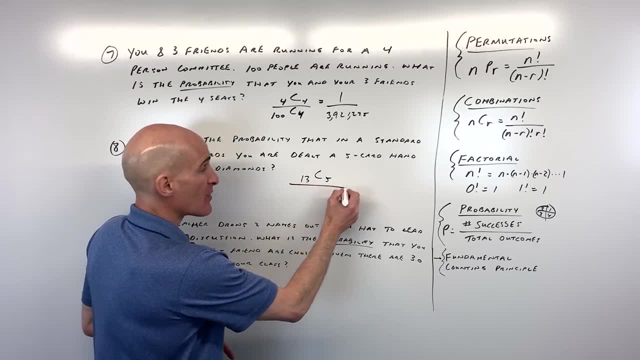 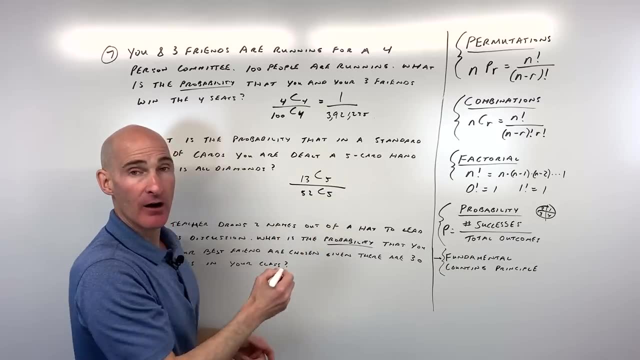 that 13.. how many ways could that occur? but it's probability divided by the total number of outcomes. well, there's 52 cards in a standard deck. how many ways are choosing five of those 52 cards where the order doesn't matter? so again, combinations. so let's see what that comes out to. so 13, combination five. 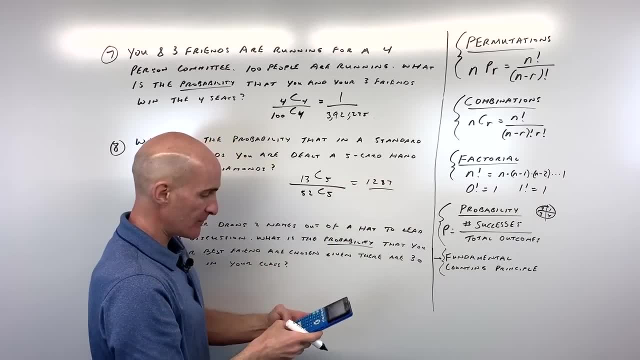 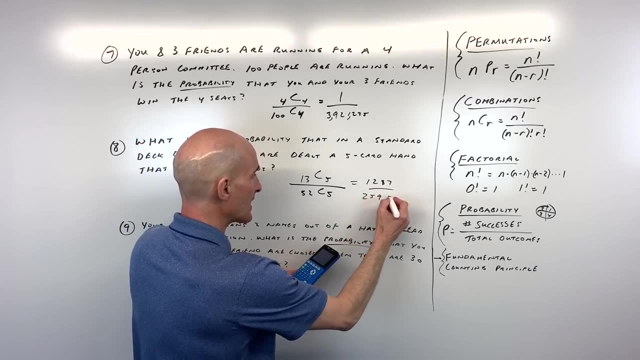 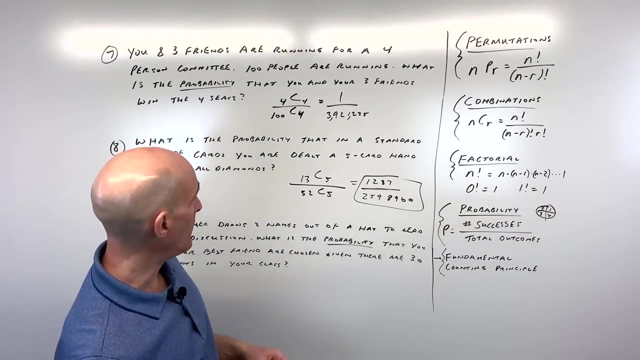 okay is 1287 and 52 combination. five is a big number here, two, five, nine, uh, eight, nine, six, zero. so that's, that's your probability and you could reduce this down or even write it as a decimal. okay. so for number nine, it says your teacher draws two names out of a hat to lead a class discussion. 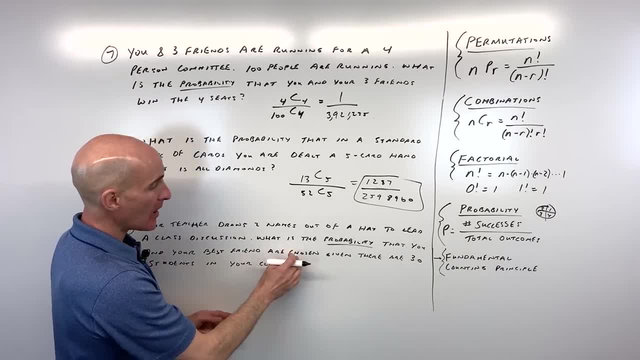 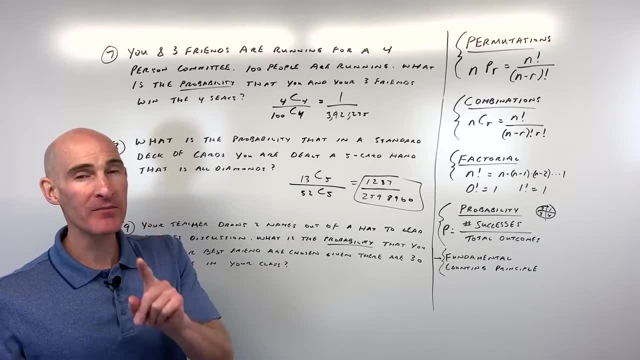 what is the probability that you and your best friend are chosen, given that there are 30 students in your class? okay, so again, we're just assuming in this problem that you just have one best friend, right? not two or three? okay, um, but it says what's the probability that the two names 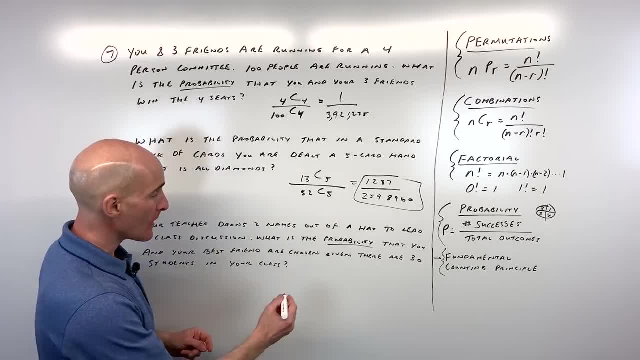 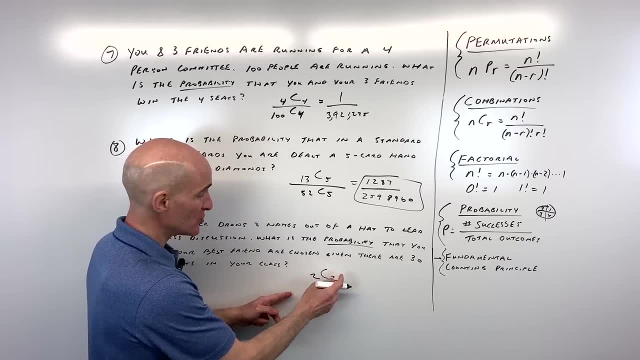 drawn are going to be you and your friend. well, again, there's only one way that it could occur. or, if you want, you could think out of these two people that you want, you and your best friend. how many ways are they're choosing those two? so two c, two or two combination, two, which is one. 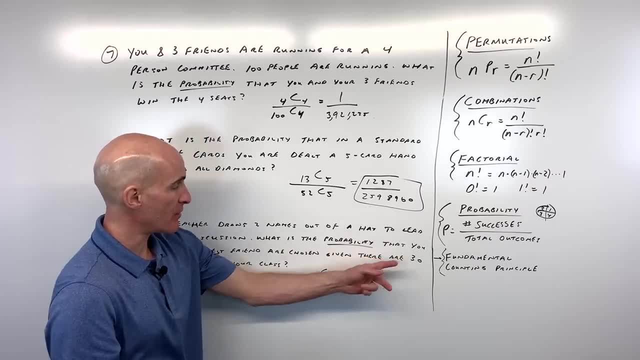 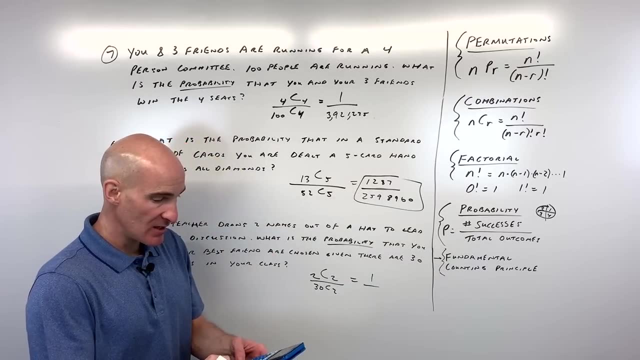 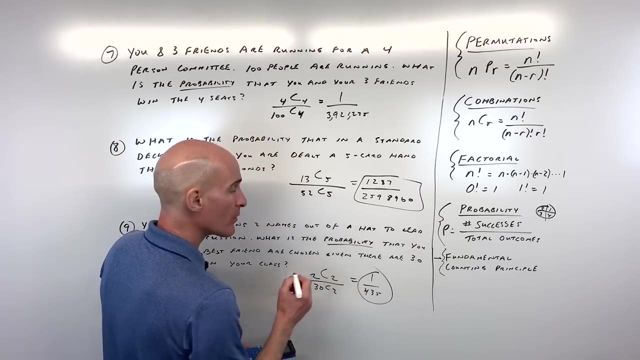 uh, but then how many ways are there of choosing, uh, two students out of the 30? that's going to be 30c2. again, we're using combinations because the order doesn't matter. it's not like it's a president, vice president, etc. so let's see what that comes out to. that's 435, so it's a one in 435, okay. so i'm trying. 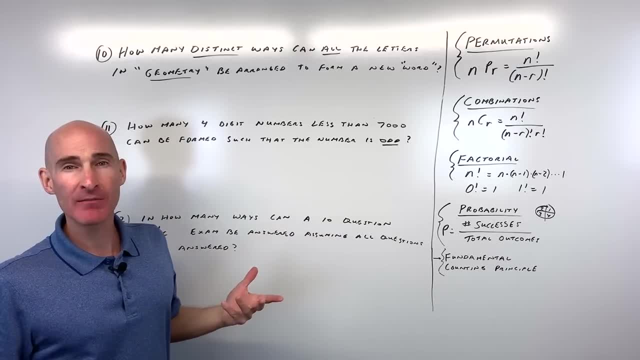 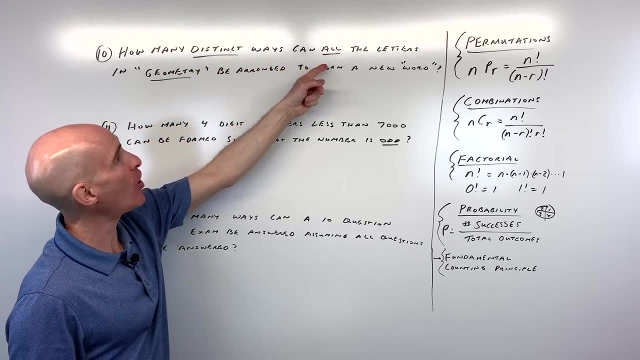 to give you a good sampling of all these different types of problems that come up when you're working with permutations, combinations, probability, etc. so number 10 is a little bit different. it says how many distinct ways can all the letters in the word geometry be arranged to form a new word? so we're. 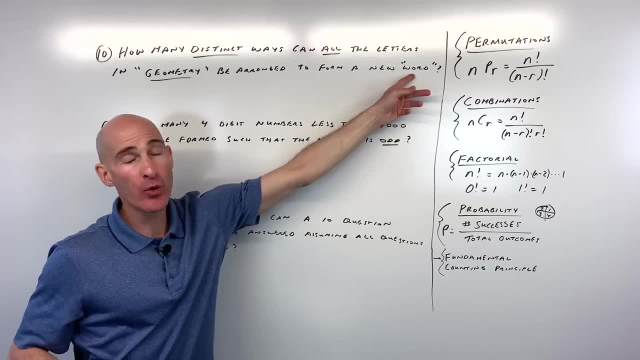 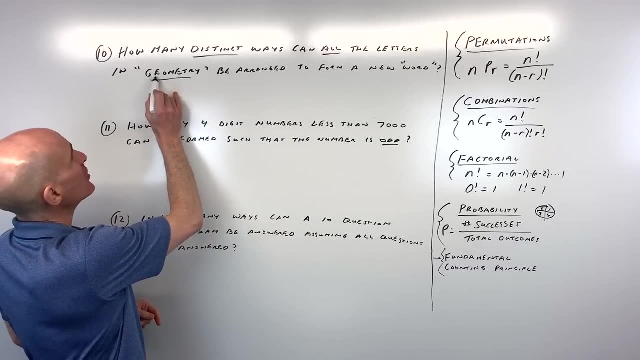 using all the letters and we're making a new quote-unquote word. it might not actually be a word, it's just kind of we're calling it a word. so the first we want to figure out is how many letters are there? there's one, two, three, four, five, six, seven, eight letters. so when you arrange eight items, how many ways are? 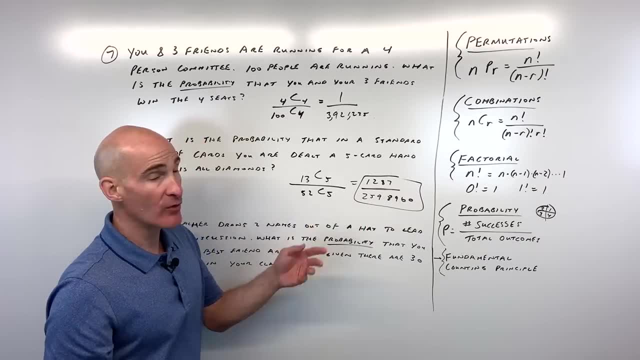 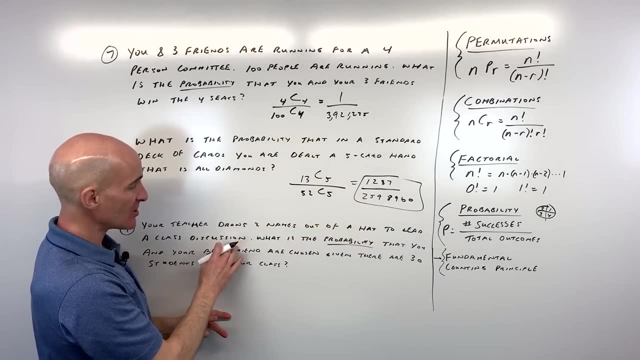 So that's your probability, and you could reduce this down or even write it as a decimal. Okay, so for number nine, it says your teacher draws two names out of a hat to lead a class discussion. What is the probability that you and your best friend are chosen, given that there are? 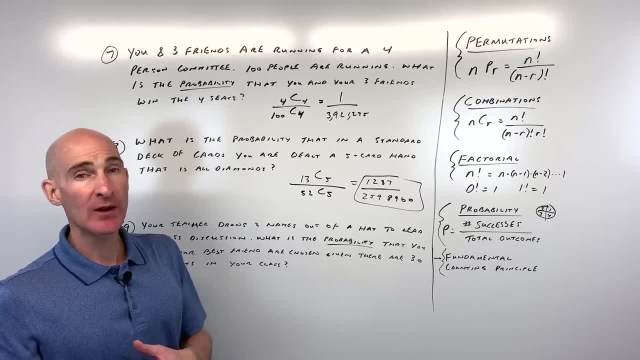 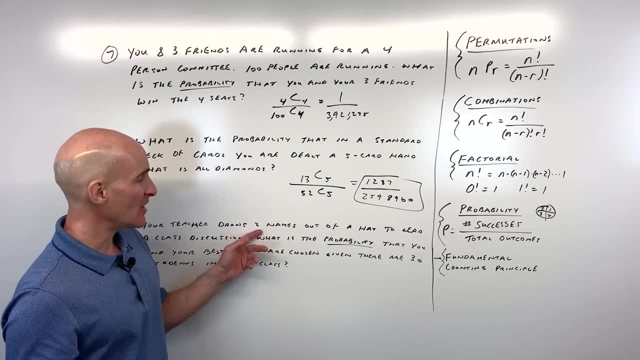 30 students in your class, Okay. so again, we're just assuming in this problem that you just have one best friend right, Or three, okay, but it says what's the probability that the two names drawn are going to be you. 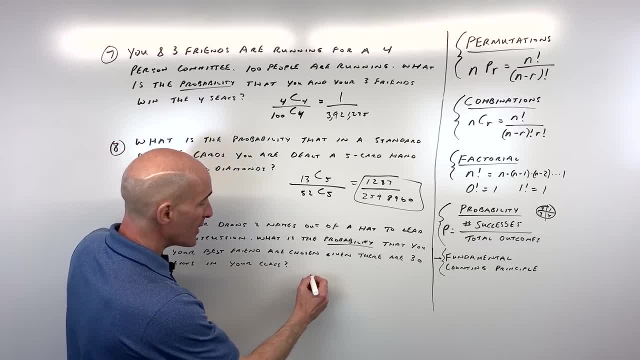 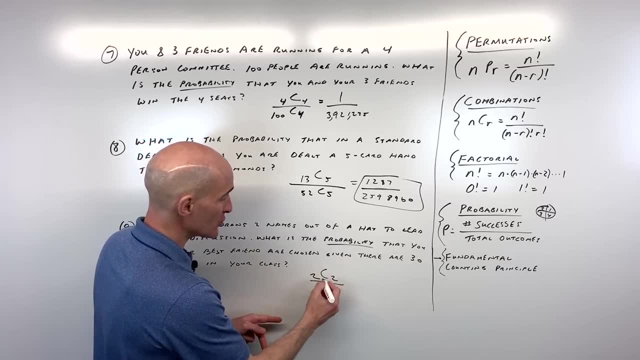 and your friend. Well, again, there's only one way that it could occur. or, if you want, you could think out of these two people that you want, you and your best friend. how many ways are they choosing those two? So 2C2 or two, combination two, which is one, but then how many ways are there of choosing? 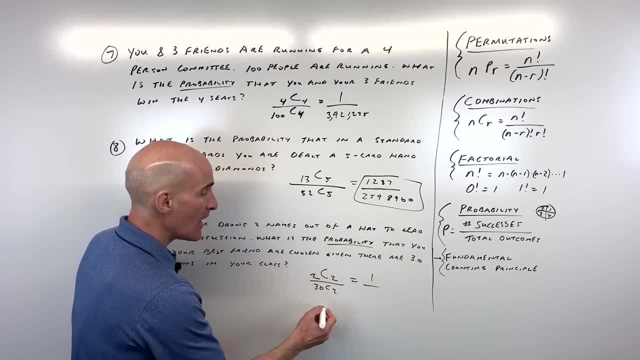 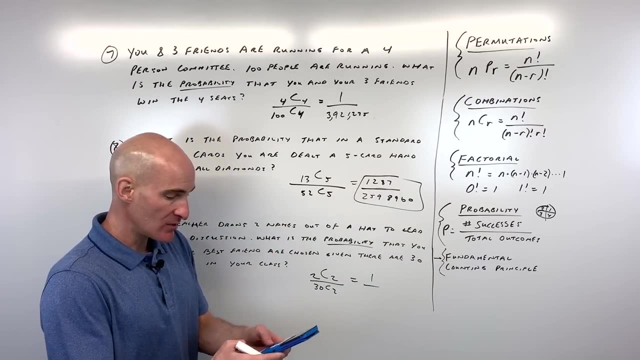 two students out of the 30? That's going to be 30C2.. Again, we're using combinations because the order doesn't matter. it's not like it's a president, vice president, etc. So let's see what that comes out to. that's 435.. 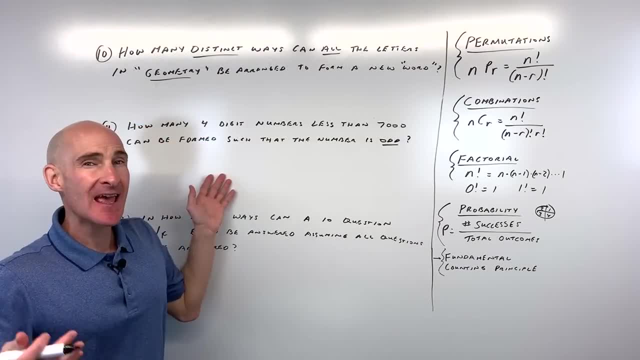 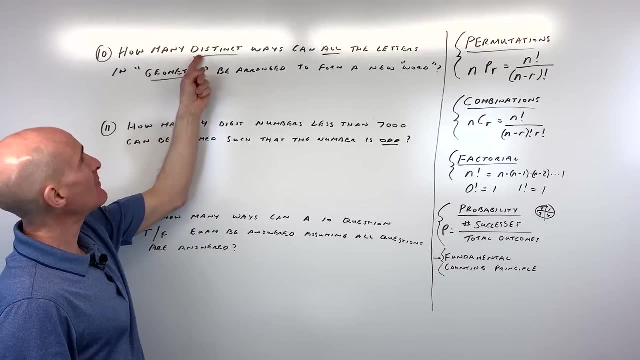 So it's a one in 435.. Okay, so I'm trying to give you a good sampling of all these different types of problems that come up when you're working with permutations, combinations, probability, etc. So number 10 is a little bit different. it says how many distinct ways can all the letters 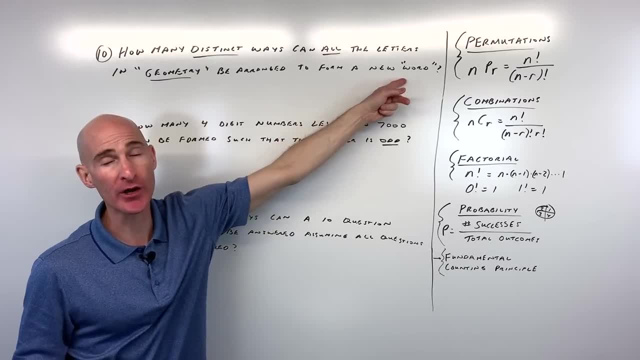 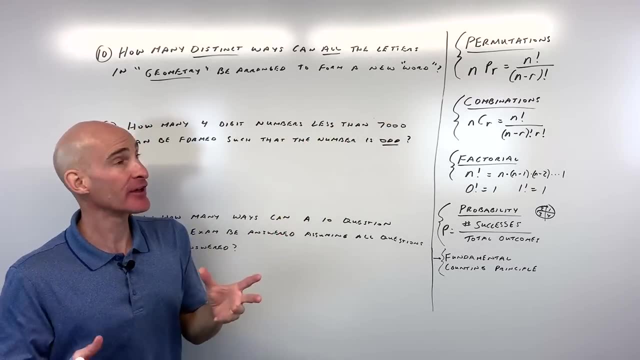 in the word geometry be arranged to form a new word. So we're using all the letters and we're making a new quote-unquote word. it might not actually be a word, it's just kind of we're calling it a word. 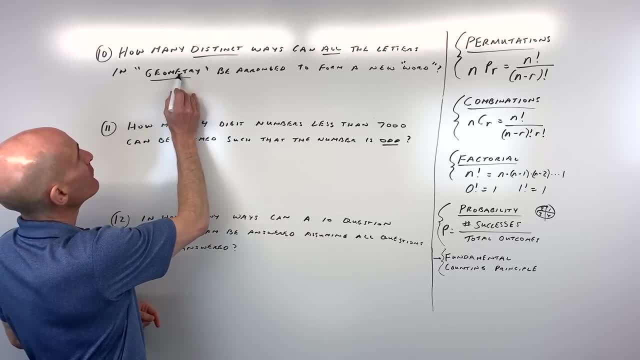 So the first thing we want to figure out is how many ways are there of choosing two students. The first thing we want to figure out is how many letters are there. There's one, two, three, four, five, six, seven, eight letters. 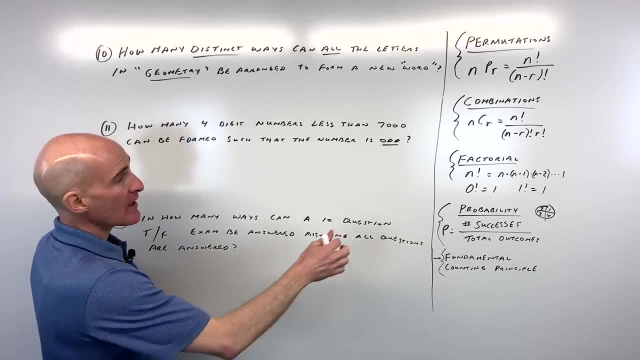 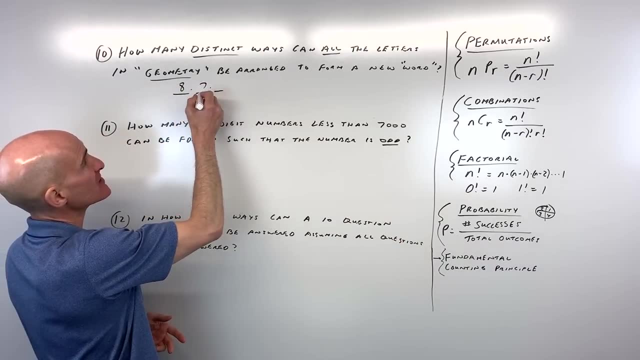 So when you arrange eight items, how many ways are there to do that? Well, that's going to be n factorial or eight factorial, You could say: well, there's eight choices for the first letter and then seven choices for the second letter and six for the. you know, it's like you're picking a letter out. 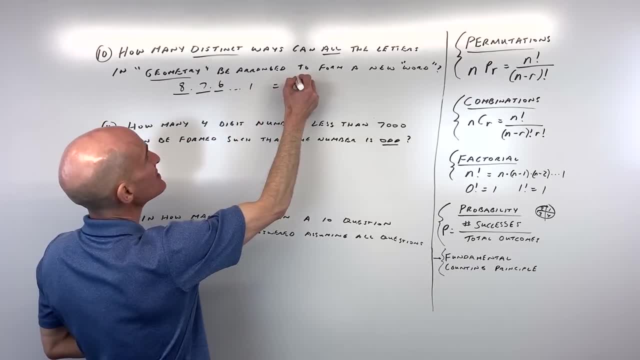 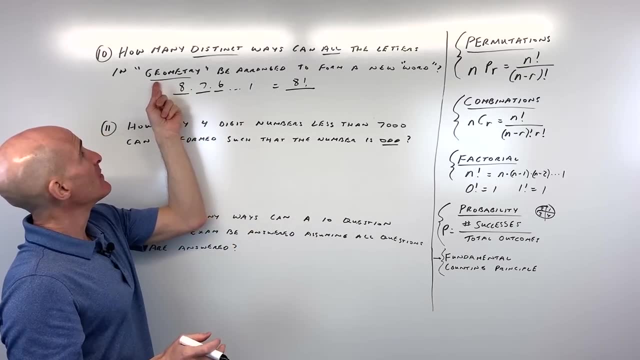 of a bag and there's eight letters, so all the way down to one. so we could say this is eight factorial. But we have a different situation here from the first problem we did, where we talked about the word math. Here you can see there's actually two e's, okay, so if I was to take this e and this, 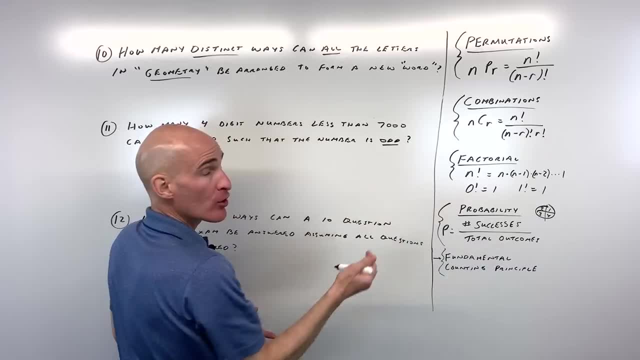 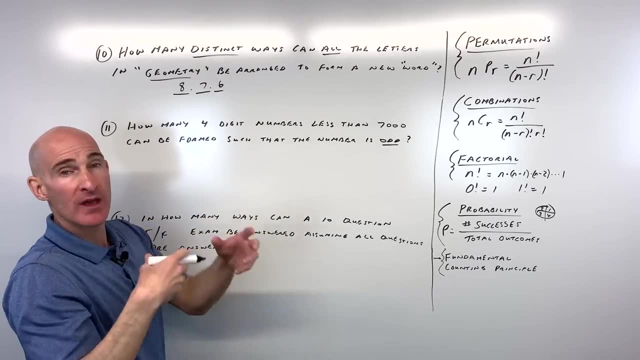 there to do that. well, that's going to be n? factorial or eight factorial, you could say. well, there's eight choices for the first letter and then seven choices for the second letter and six for the. you know, it's like you're picking a letter out of a bag and there's eight letters, so all the. 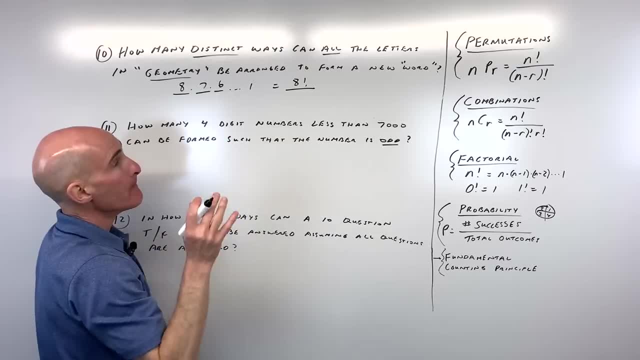 way down to one. so we could say this is eight, five, six, seven, eight, eight, eight, eight, eight, eight, nine, nine, ten. so we could say this is eight, three, four, five, six, seven, nine, eight, two, three, three, four, five, six, seven, eight, two, three. but we have a different situation here from the. 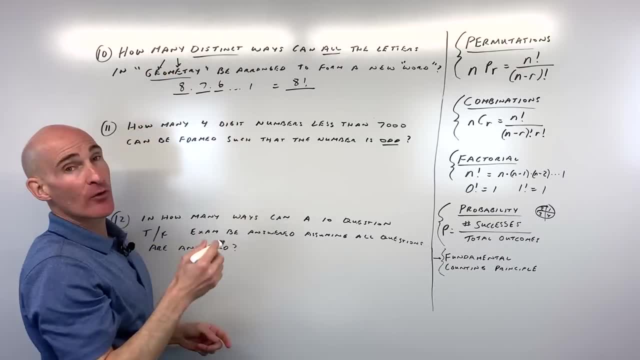 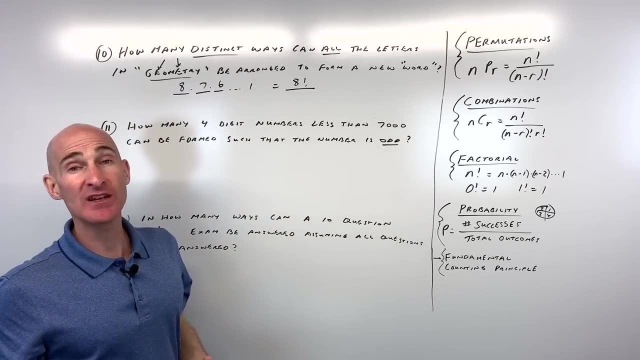 first problem we did when we talked about the word math. here you can see there's actually two. uh, e's okay. so if i was to take this e and this e and like interchange them, it would still look like the word geometry. it wouldn't be distinct, it wouldn't be unique, it wouldn't be different. 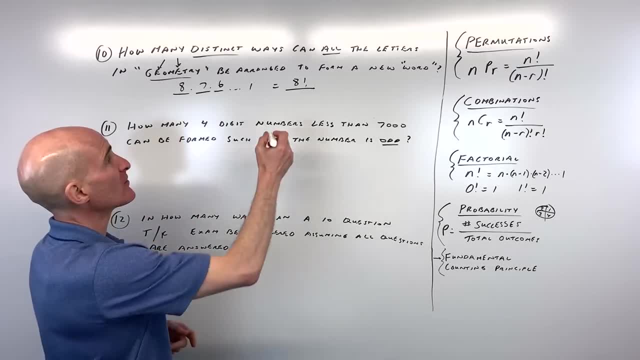 right. so we don't want to double count. you know when i switch these two e's. so to avoid double counting, what we have to do is we have to divide by two factorial. now two factorial is just two, And if I mispronounce something that I didn't do, then you have two e's. so you have two e's and if I change them by two, 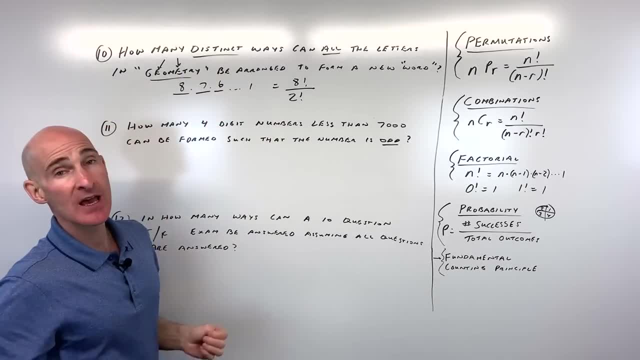 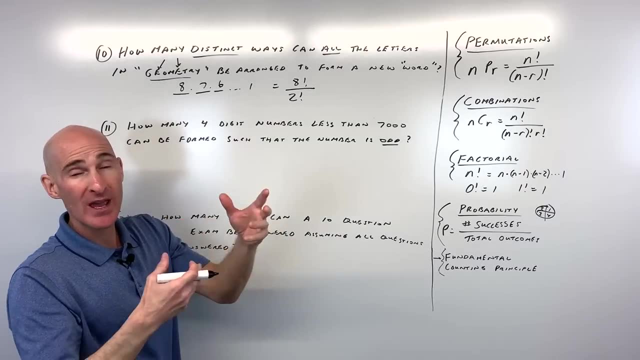 factorial is just two times one. it's just two because there's two different ways. If there was three e's, we would divide by three factorial, which is three times two times one, which is six. There would be six different ways that you could arrange those like three e's, but it would still look like 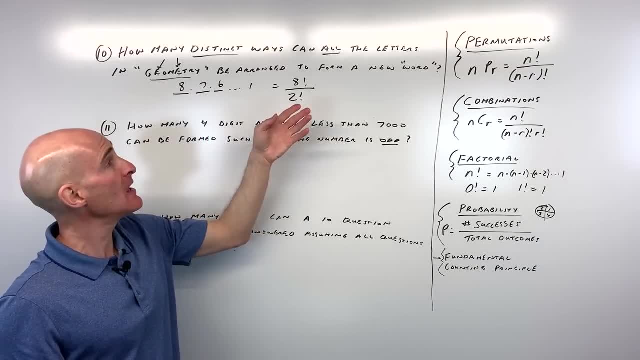 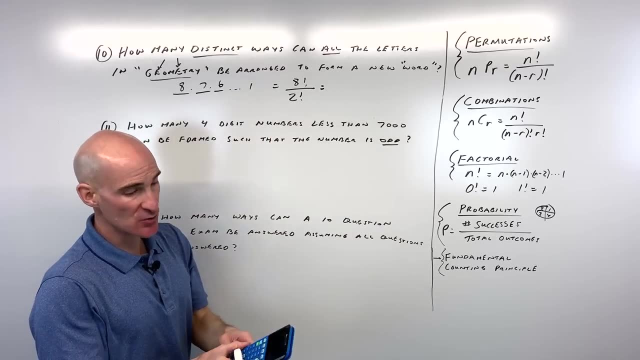 the same word, But in this case there's just two e's. we're dividing by two factorial, And let's expand this out. so this would be: let's see eight times seven times six times five, all the way down to one divided by two times one, and let's see what that comes out to. So eight factorial divided by. 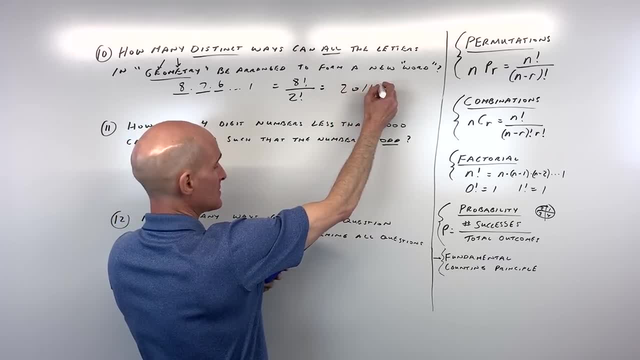 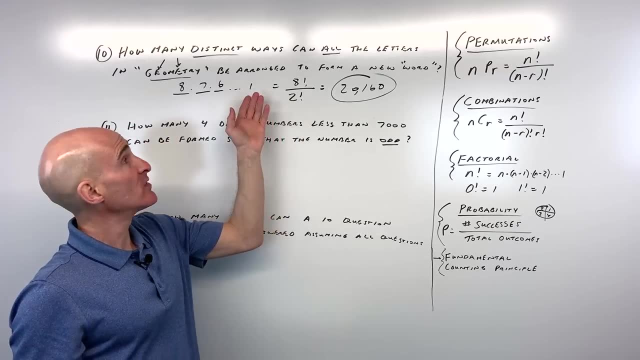 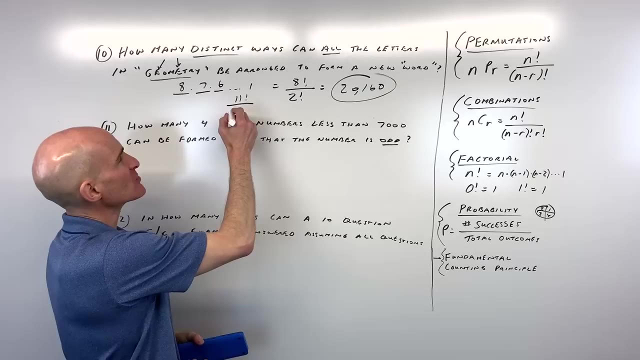 two factorial. so it comes out to two zero, one, six zero. So 20,160 ways that you could do that. A common example with this one that often comes up is like the word Mississippi, So Mississippi, actually there's 11 letters, that's 11 factorial. but there's four s's, there's four i's and there's. 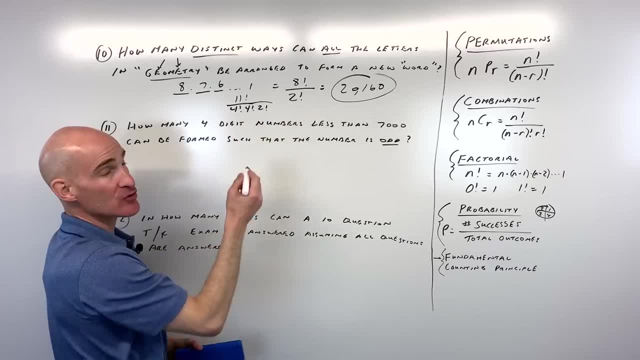 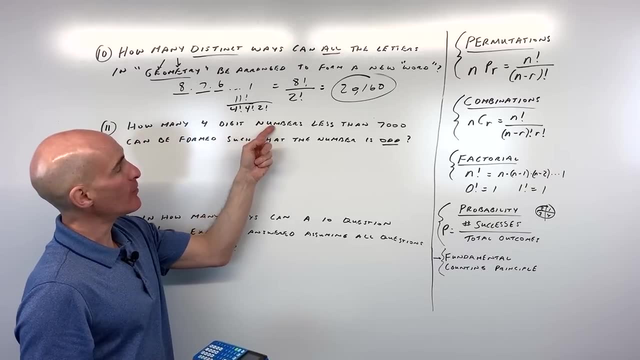 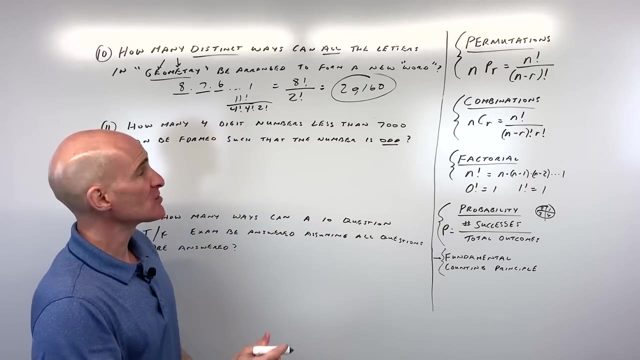 two p's You'd have to divide by four factorial, four factorial, two factorial to divide out those multiplicities. Okay, so let's look at number 11 now. It says how many four digit numbers less than 7,000 can be formed such that the number is odd. Okay, so what I like to do sometimes with 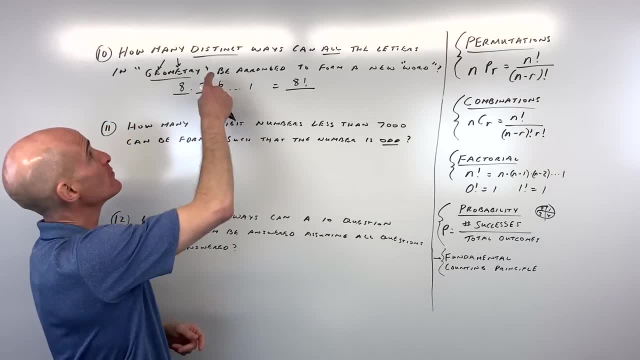 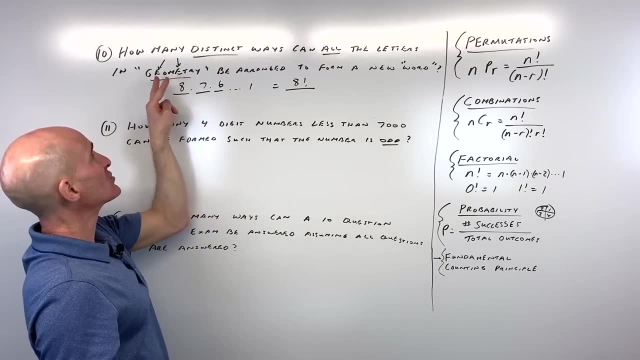 e and like interchange them, it would still look like the word geometry, It wouldn't be distinct, it wouldn't be unique, it wouldn't be different, right? So we don't want to double count, you know, when I switch these two e's, so to avoid double. 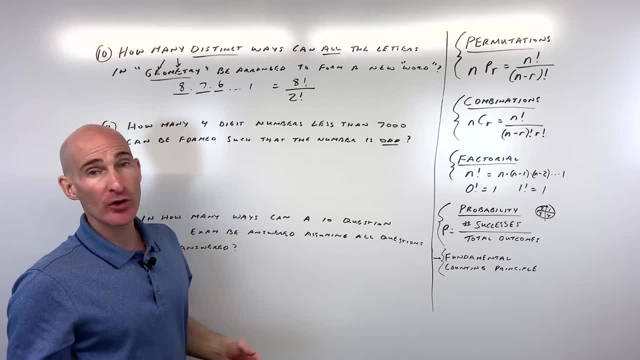 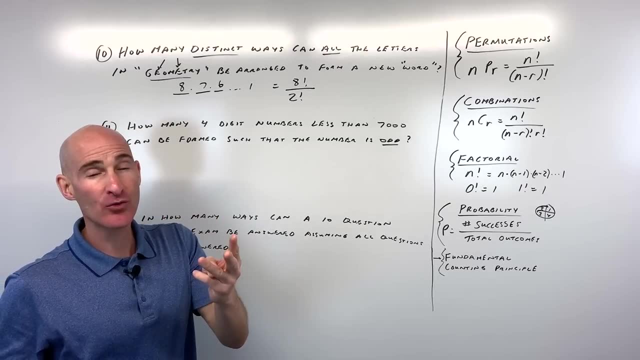 counting. what we have to do is we have to divide by two factorial. Now, two factorial is just two times one. it's just two because there's two different ways. If there was three e's, we would divide by three factorial, which is three factorial. 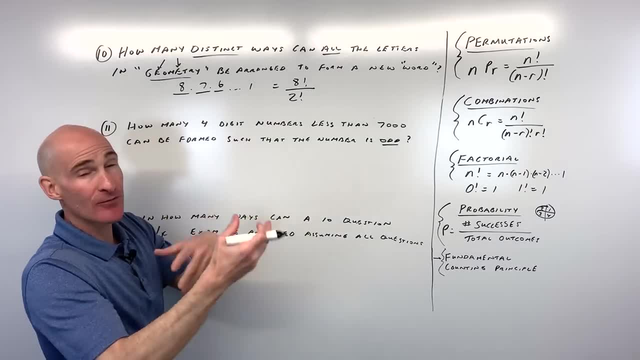 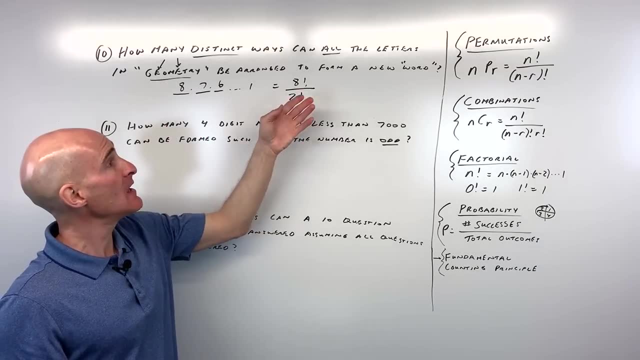 Okay, So that's three times two times one, which is six. There would be six different ways that you could arrange those. like three e's, but it would still look like the same word. But in this case there's just two e's. so we're dividing by two. factorial. 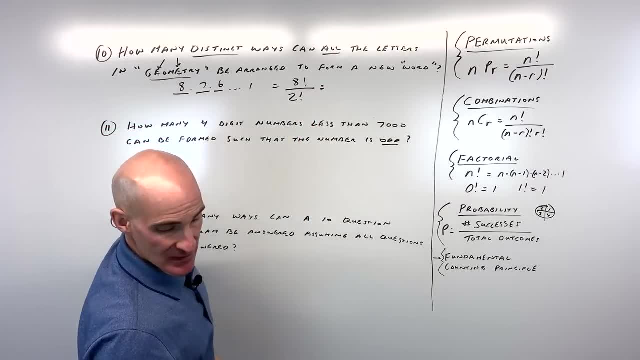 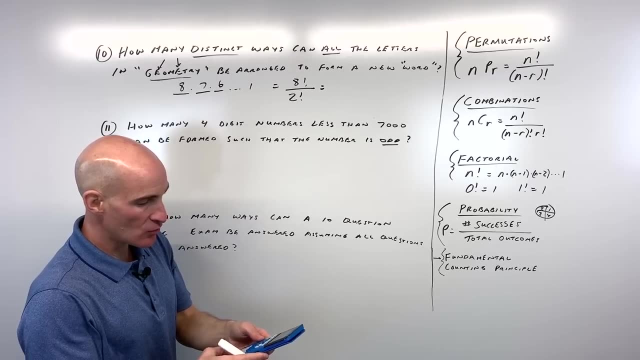 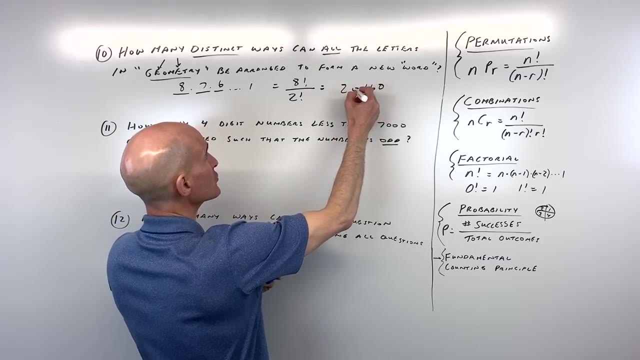 And let's expand this out. so this would be: let's see eight times seven times six times five, all the way down to one divided by two times one, and let's see what that comes out to. So eight factorial divided by two factorial. so it comes out to two zero one, six zero. 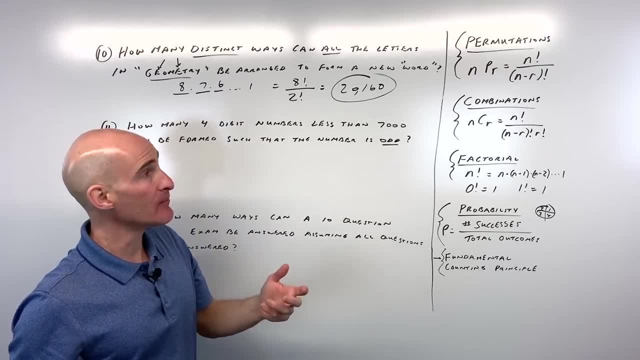 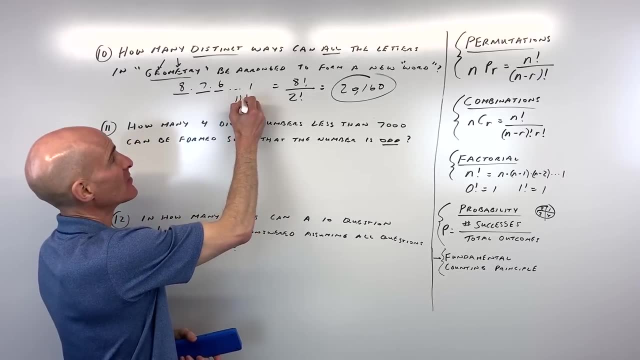 So twenty thousand one hundred and sixty factorial. So there's a lot of ways that you could do that. A common example with this one that often comes up is like the word Mississippi, So Mississippi, actually there's eleven letters, that's eleven factorial, but there's four. 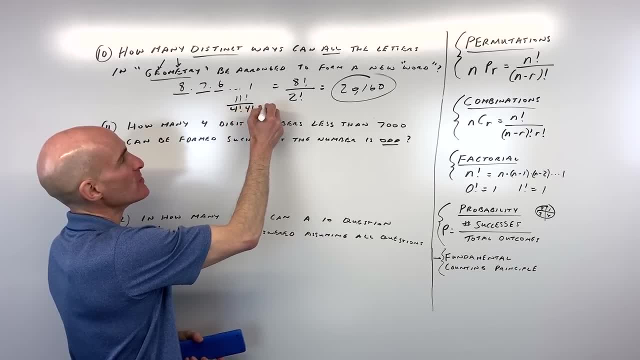 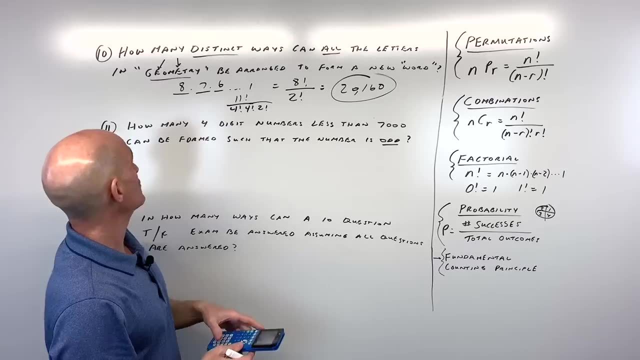 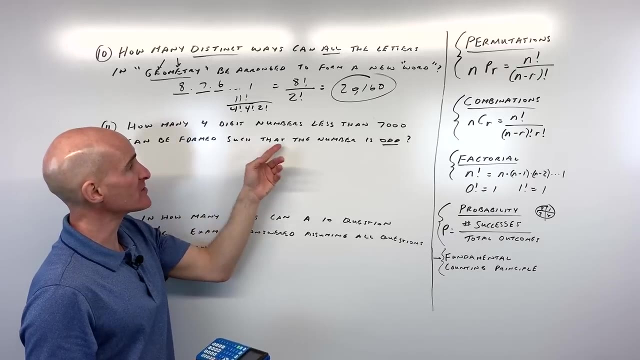 s's, there's four i's and there's two p's. So you'd have to divide by four factorial. four factorial, two factorial to divide out those multiplicities. Okay, so let's look at number eleven now. It says how many four digit numbers less than seven thousand can be formed such that the 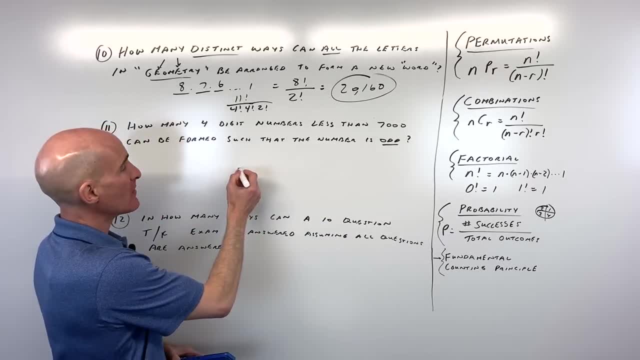 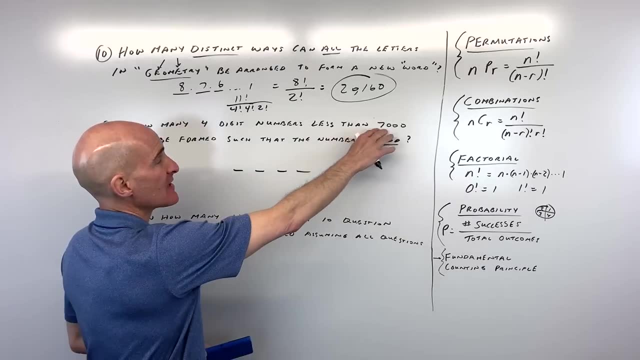 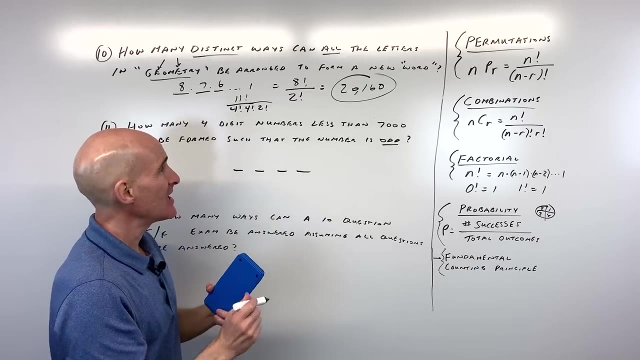 number is odd, Okay. so what I like to do sometimes with these problems is I like to diagram it out. Okay, it's a four digit number and it has to be less than seven thousand, So the first digit has to be what has to be a one, two, three, four, five or a six. 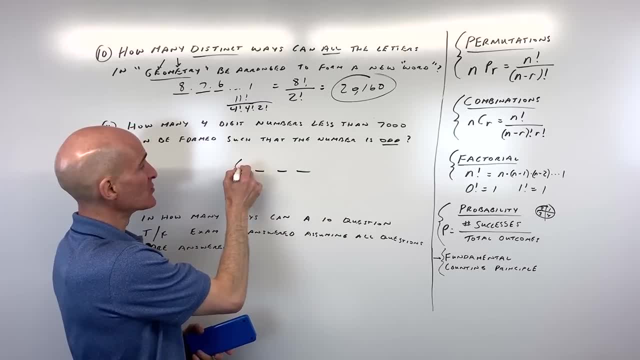 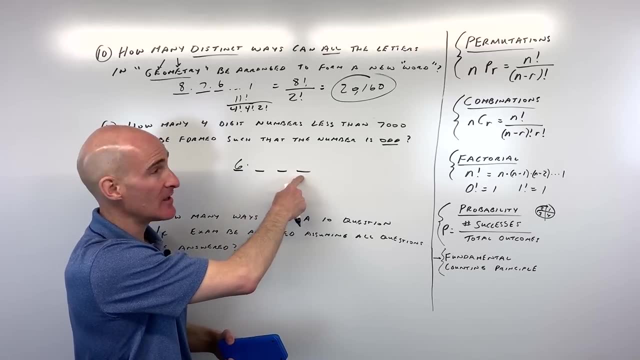 It couldn't be a seven, because then it wouldn't be less than seven thousand. So that means there's six choices for this first number. Now notice I didn't mention zero, because if it was zero then it would only be a three digit number. 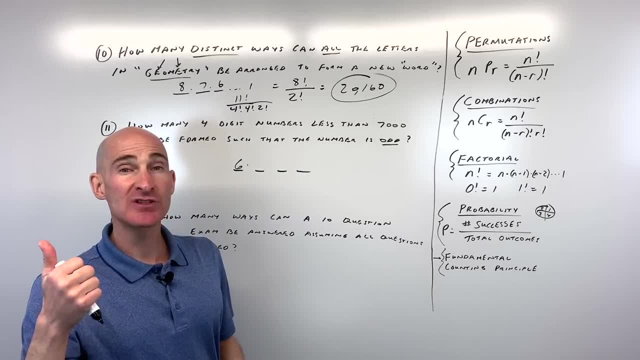 Let's jump to this last number here. If you want it to be odd, the only way it can be an odd number is if the last digit is odd. It has to be a one. three, five, seven, nine, right. 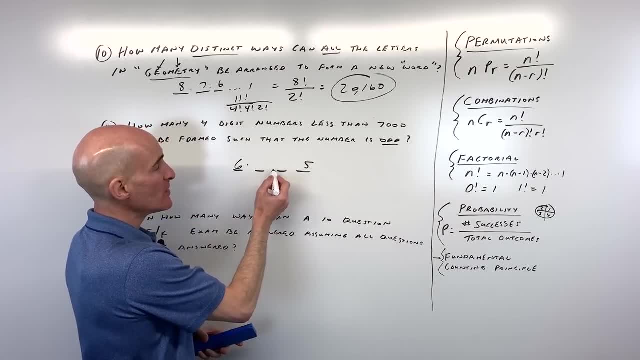 So there's five different outcomes for the last digit, but these two middle digits, they could be zero: one, two, three, four, five all the way up to nine. So zero through nine. if you add those up, there's actually ten possibilities for the. 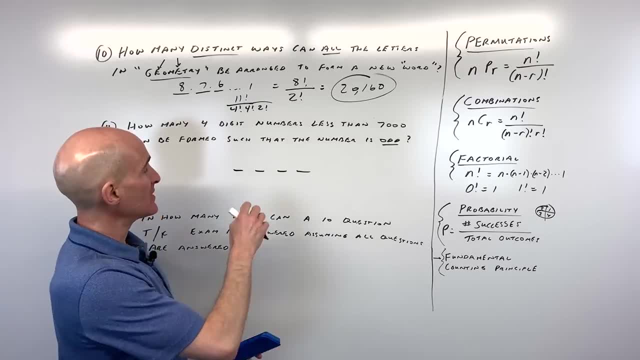 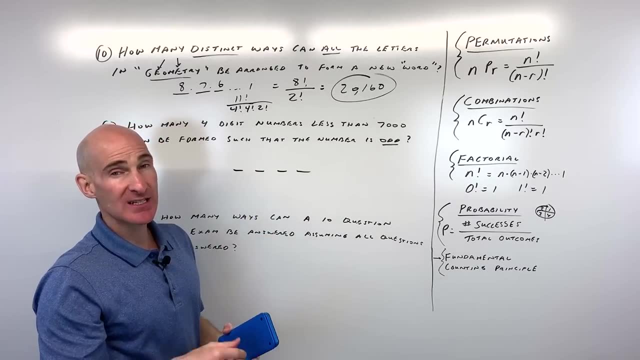 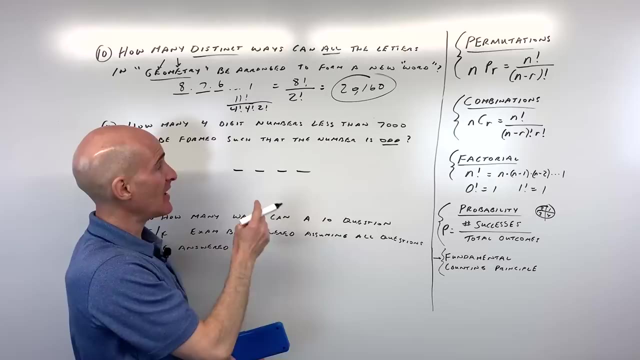 these problems is like to diagram it out. Okay, it's a four digit number and it has to be less than 7,000. So the first digit has to be what has to be: a one, two, three, four, five Or a six. It couldn't be a seven, because then it wouldn't be less than 7,000. So that means there's 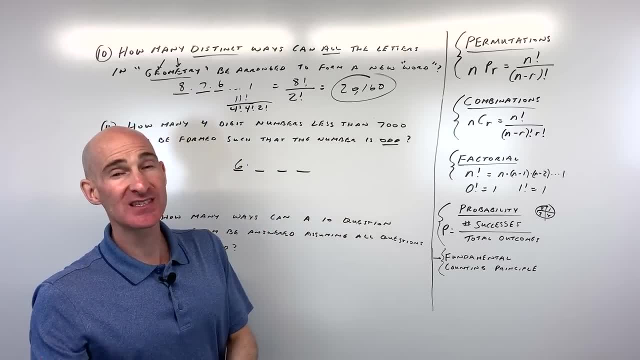 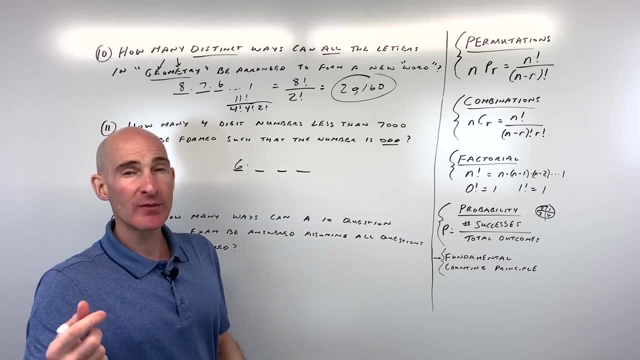 six. uh, choices for this first number. Now I notice I didn't mention zero, because if it was zero then it would only be a three digit number. Let's jump to this last number here. If we want it to be odd, the only way it can be an odd number is if the last digit is odd. It has to be a one, three, five. 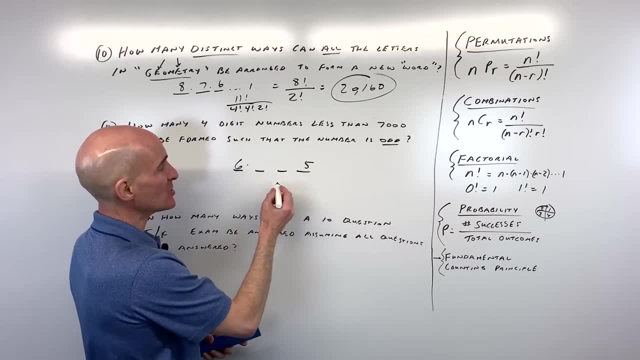 seven, nine, Right, so there's five different outcomes for the last digit. but these two middle digits, they could be zero, one, two, three, four, five, all the way up to nine. So zero through nine. if you add those up, there's actually ten possibilities for the second digit and ten. 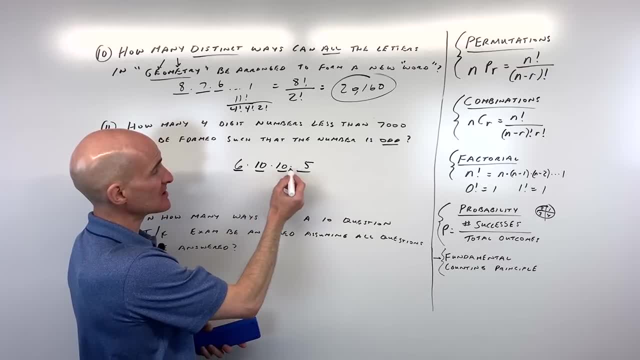 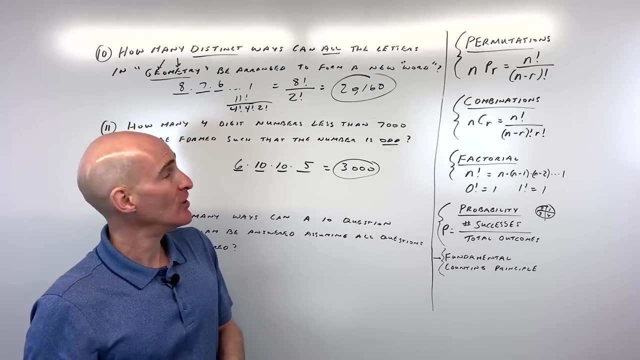 for the third. So if you multiply these together you're going to get six times five is thirty times a hundred, which comes out to three thousand, Which you probably could just figure that out, you know, uh, just on your own. You could say: well, from 1,000 to 7,000, that's 6,000 numbers, half of them. 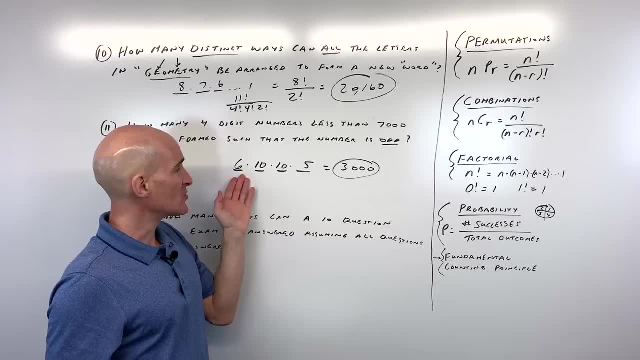 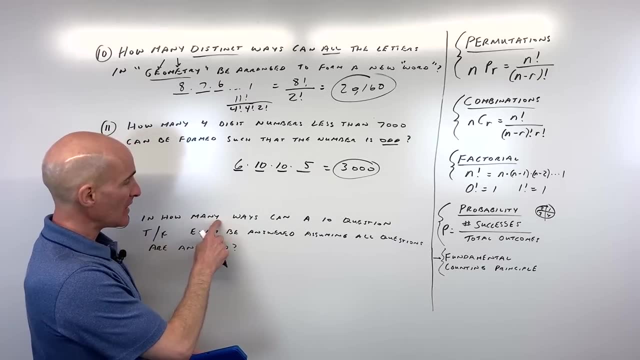 are odd 3,000.. But sometimes the problems are a little bit more complicated, so I wanted to show you this process of using this fundamental counting principle. Okay, for number 12 now. it says in high. it says: in how many ways can a 10 question true, false exam be answered, assuming that all questions? 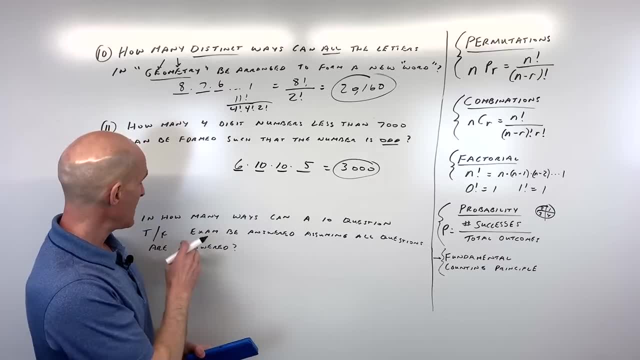 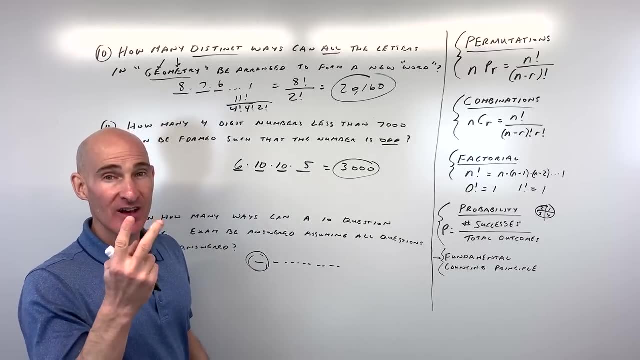 are answered. This is also a common problem that comes up Again if it's a 10 question exam. imagine those 10 questions. how many ways can you answer that first question? Two ways, right, either true or false. How many ways can you answer the second question? Two ways, right, true or false. How many? 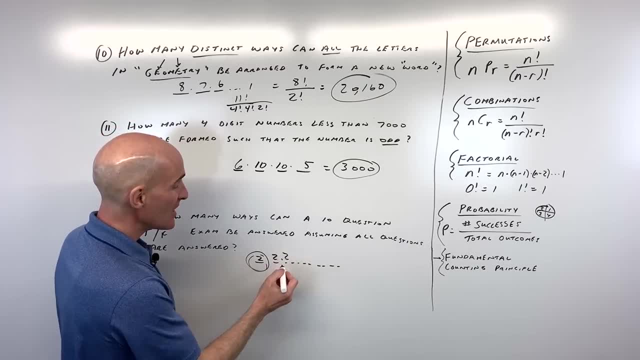 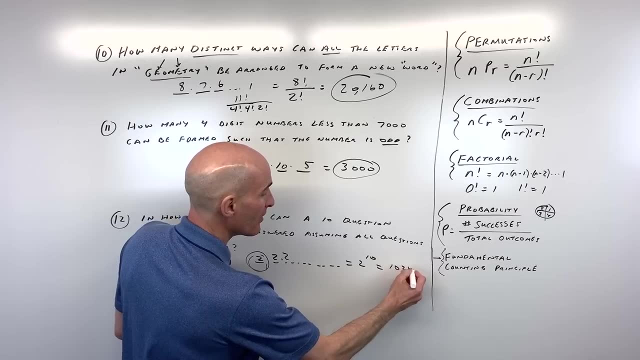 ways. can you answer the third question? Two ways? true or false? So what's two times two times? two times two, 10 times? Well, that's going to be 2 to the 10th, which is equal to 1024 different ways that. 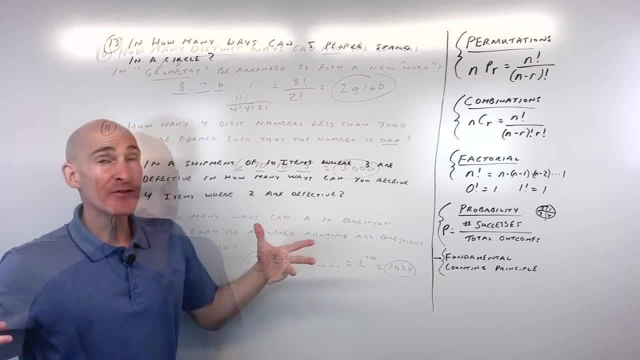 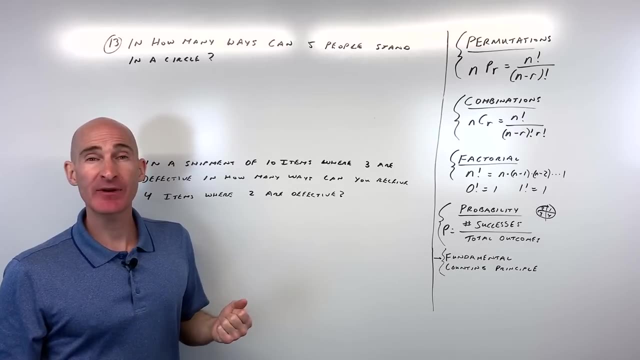 you could answer this true false test. Okay, if there's a problem that you have a question about regarding permutations, combinations or probability problem involving permutations and combinations that we haven't covered yet in this lesson, go ahead and put it in the comments below and, if you're 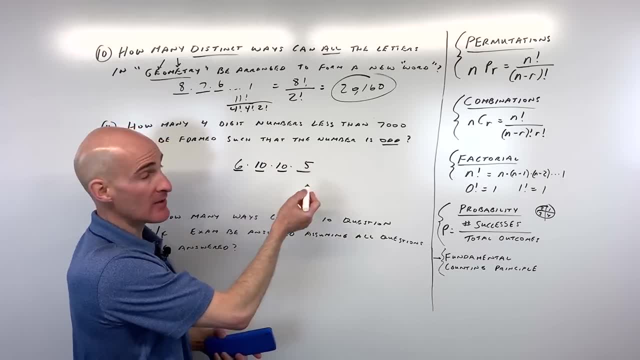 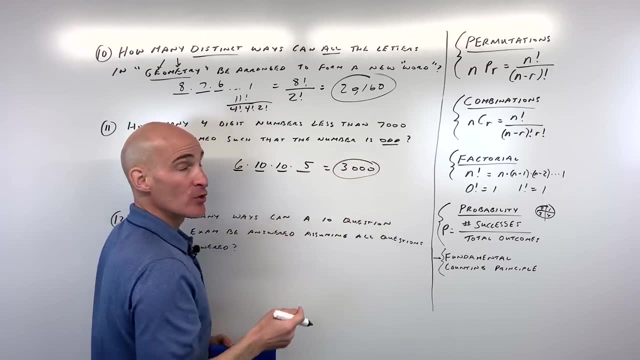 second digit and ten for the third. So if you multiply these together, you're going to get six times five, is thirty times a hundred, which comes out to three thousand, which you probably could just figure that out, you know, just on your own. 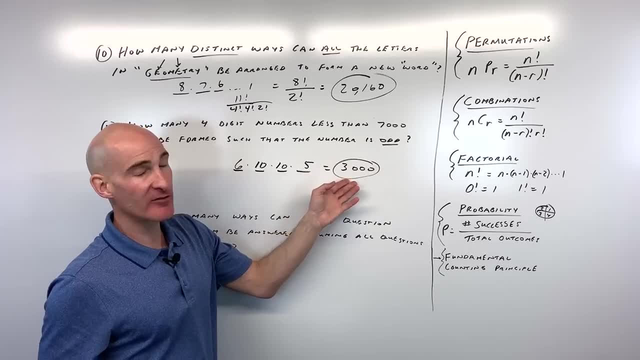 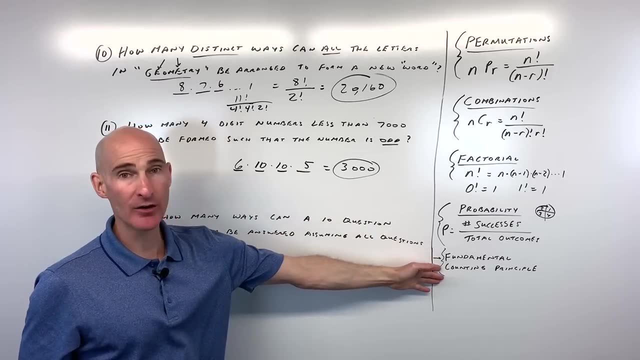 You could say: well, from one thousand to seven thousand, that's six thousand numbers, half of them are odd, three thousand. But sometimes the problems are a little bit more complicated. so I wanted to show you this process of using this fundamental counting principle. 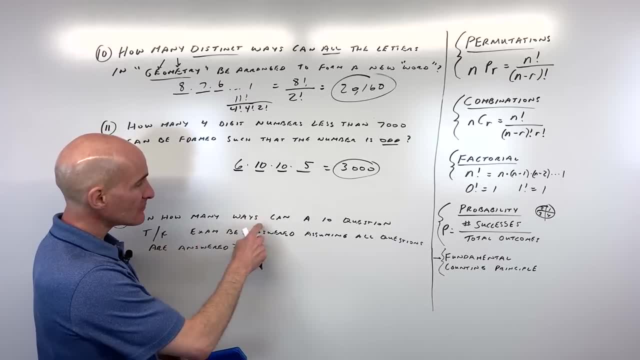 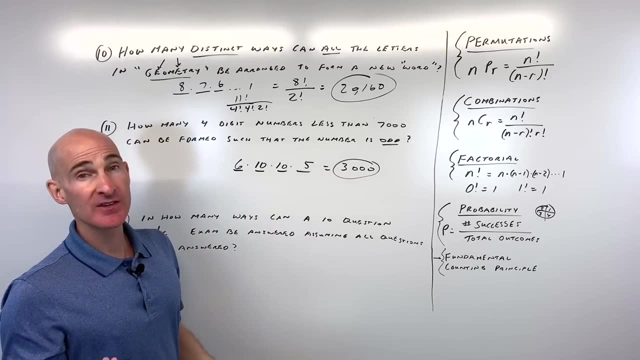 Okay for number twelve. now it says: in how many ways can a ten question true-false exam be answered, assuming that all questions are answered? This is also a common problem that comes up again if it's a ten question exam. imagine: 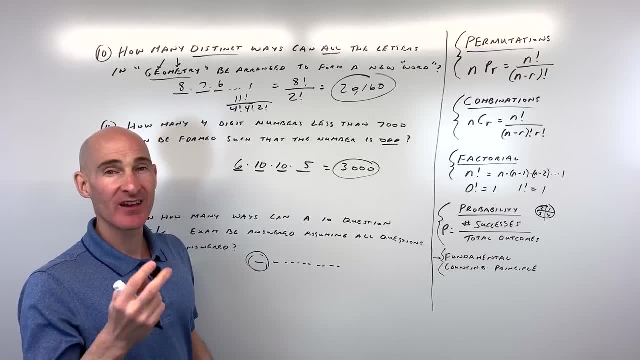 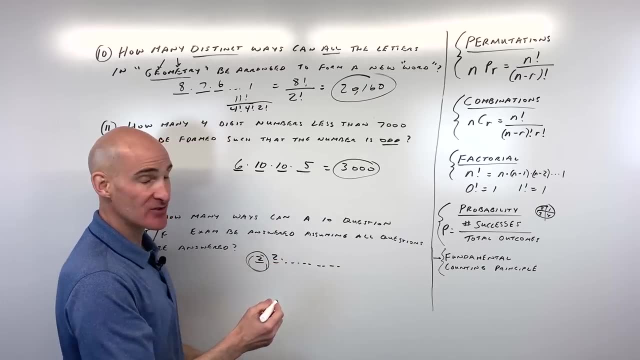 those ten questions. How many ways can you answer that first question? Two ways right, Either true or false. How many ways can you answer the second question? Two ways right, True or false. How many ways can you answer the third question? 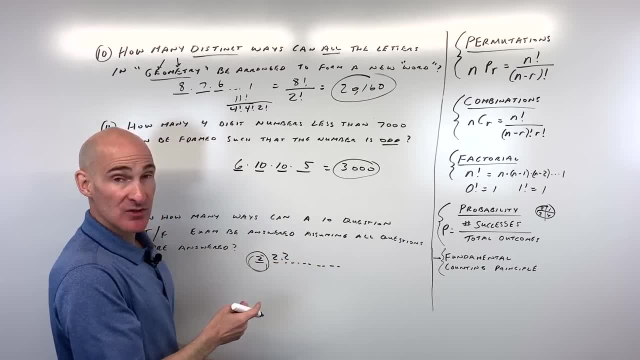 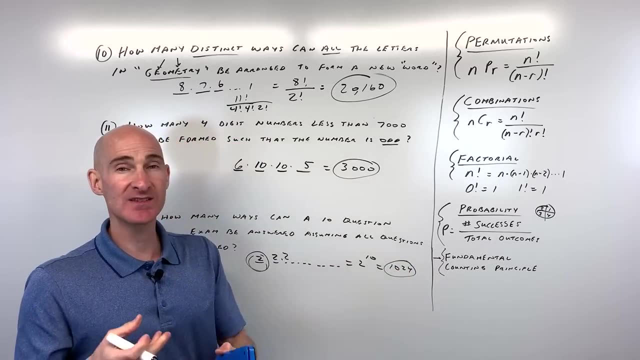 Two ways, true or false. So what's two times two times two times two, Ten times? Well, that's going to be two to the tenth, which is equal to 1024 different ways that you could answer this true-false test. 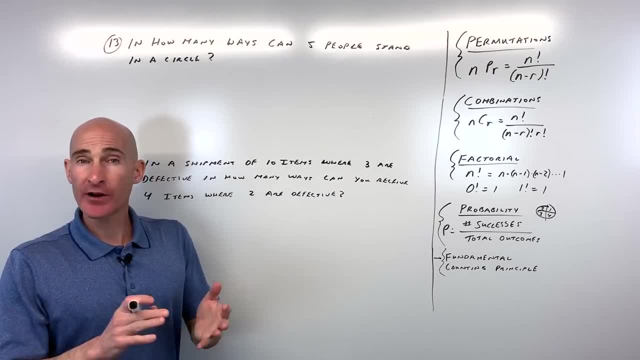 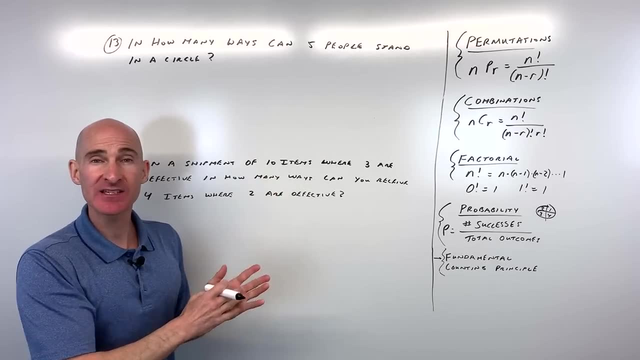 Okay, if there's a problem that you have a question about regarding permutations, combinations or probability problem involving permutations and combinations that we haven't covered yet in this lesson, go ahead and put it in the comments below And, if you're watching this video, see if you can answer those questions that people. 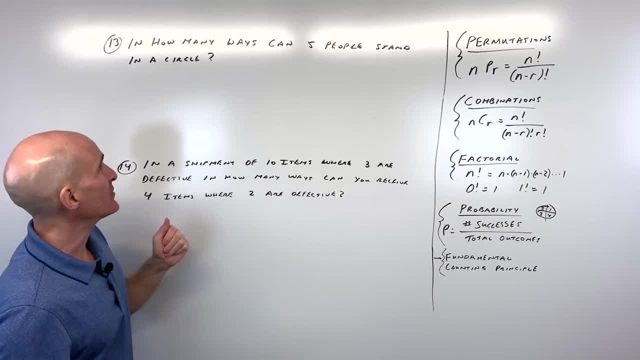 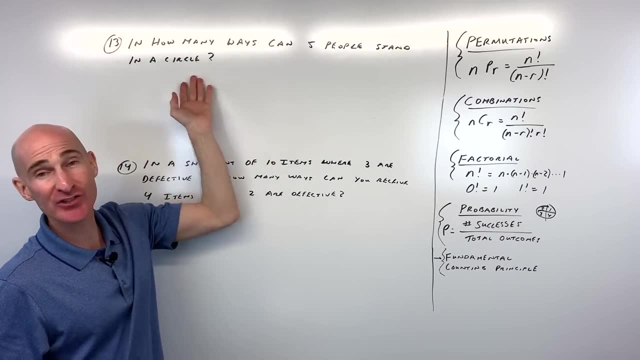 are posing down there in the comments questions in the comments. So for number thirteen now it says: in how many ways can five people stand in a circle? Now this is a little bit more complicated problem than if we say how many different. 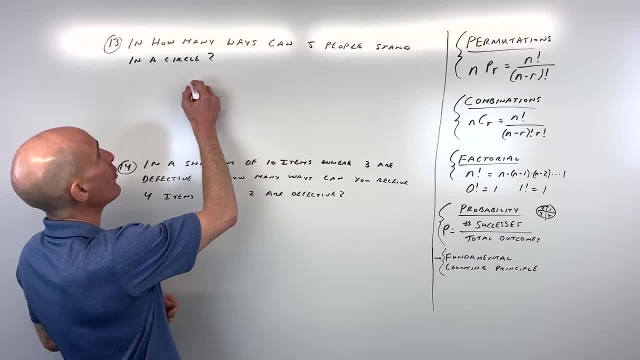 ways can five people stand in a row? See, if it was in a row, it would be like this: They could stand five choices for who stands here furthest to the left. Once that person stands there, there's four people to compete for. who's going to stand? 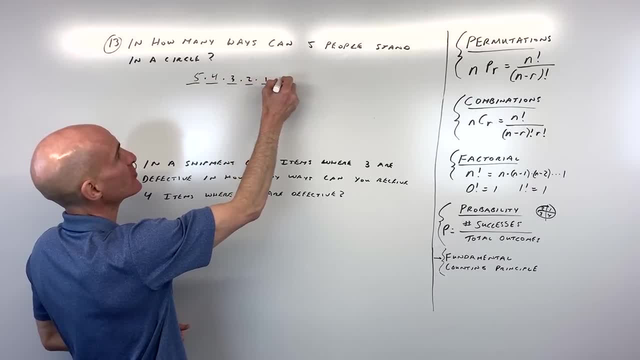 right here, and then three, and then two, and then one, and you would multiply all those together, and you'd say: there's 120 different ways. The problem here, though, is that, when you're standing in a circle, okay, kind of imagine. 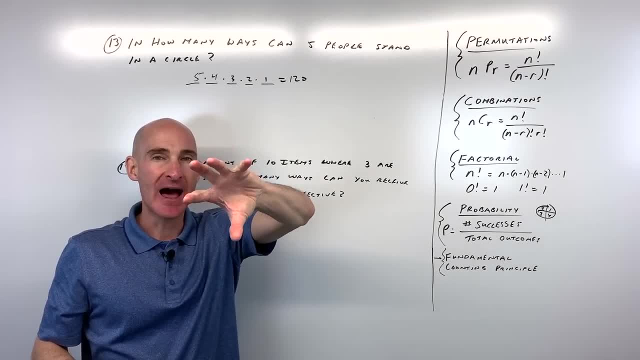 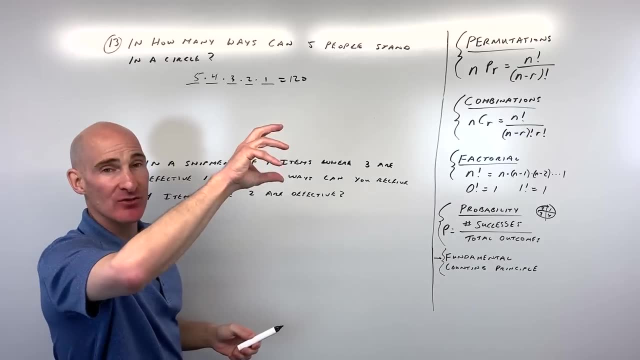 my five fingers here. it's like a dial or a knob, Like if I was to rotate like that right. the thing is, you can turn that knob five times right And get back to the original position, but whoever's standing on your left and who's 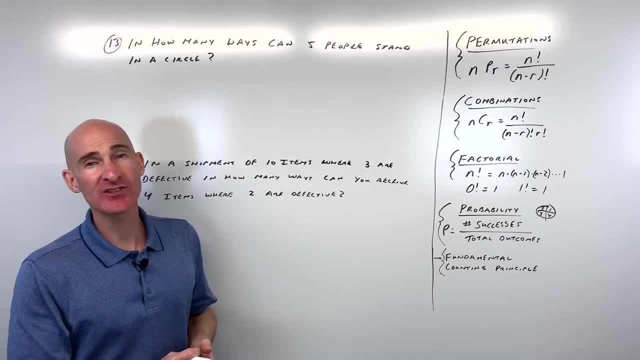 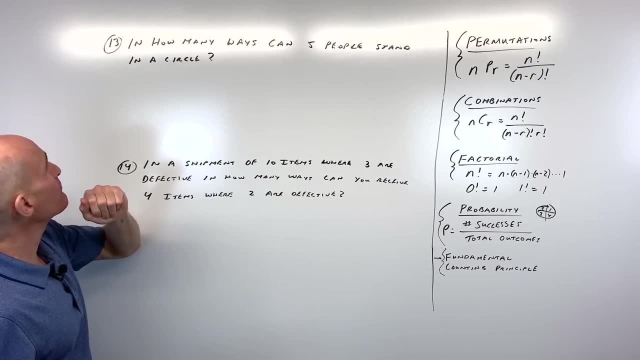 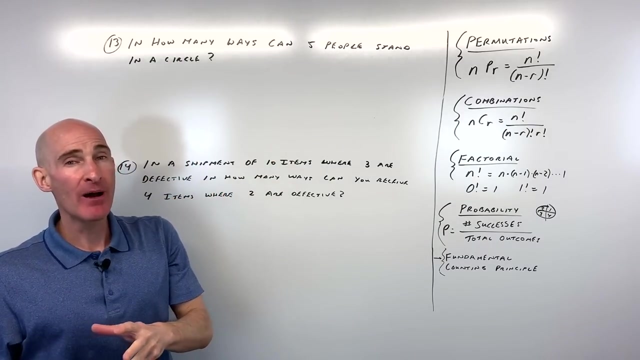 watching this video see if you can answer those questions that people are posing down there in the in the comments. So for number 13. now it says in how many ways can five people stand in a circle? Now this is a little bit more complicated problem than if we say how many different ways can five? 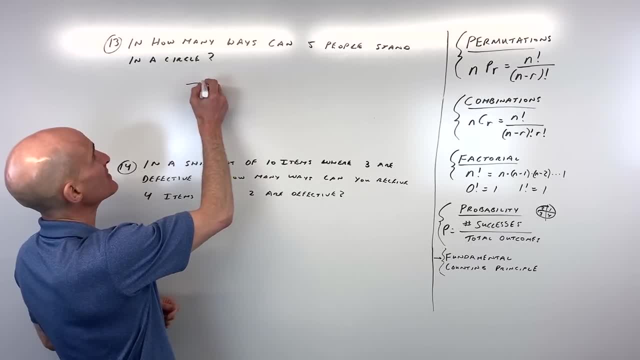 people stand in a row. See, if it was in a row, it would be like this: they could stand five choices for who stands here furthest to the left. Once that person stands there, there's four people to compete for who's going to stand right here, and then three, and then two, and 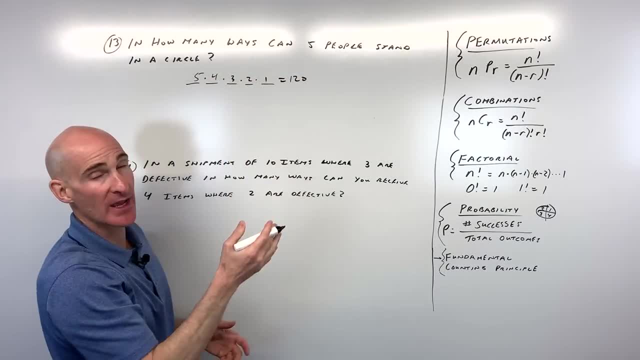 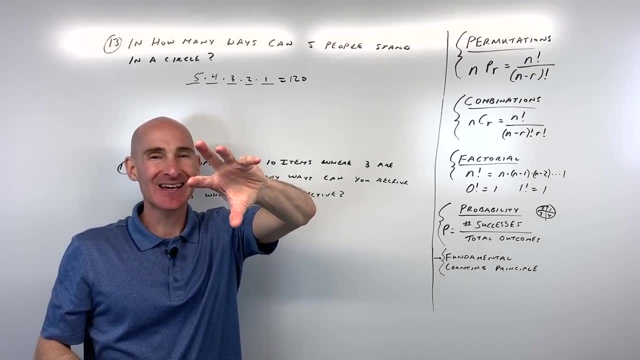 then one, and you would multiply all those together, and you'd say: there's 120 different ways. The answer here, though, is: is that when you're standing in a circle- okay, kind of imagine my five fingers here- it's like a dial or a knob, like if I was to rotate. 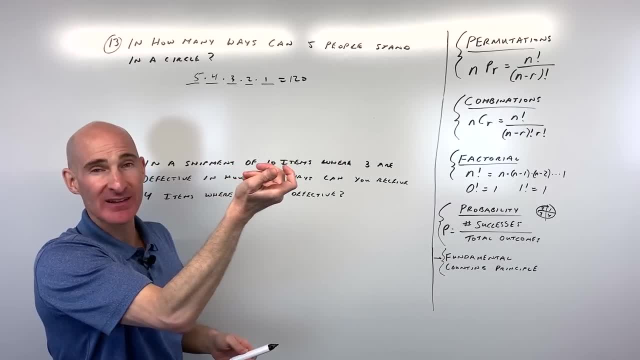 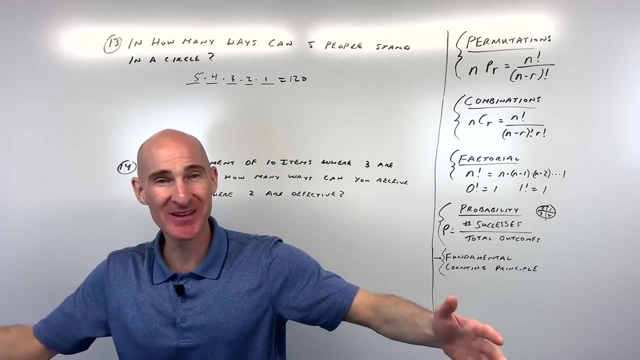 like that, right. the thing is, you can turn that knob five times right until you get back to the original position, but the whoever's standing on your left and who's ever standing on your right, when you keep turning like this, they're gonna, you're gonna be in the same. 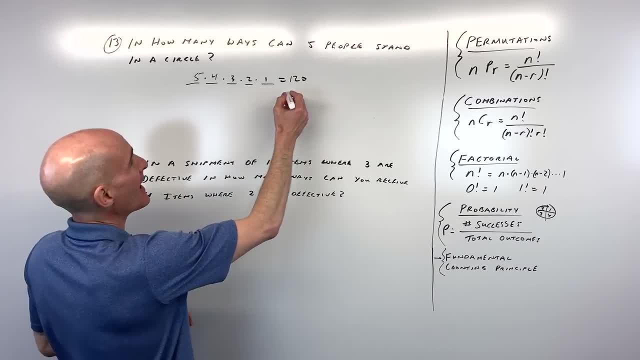 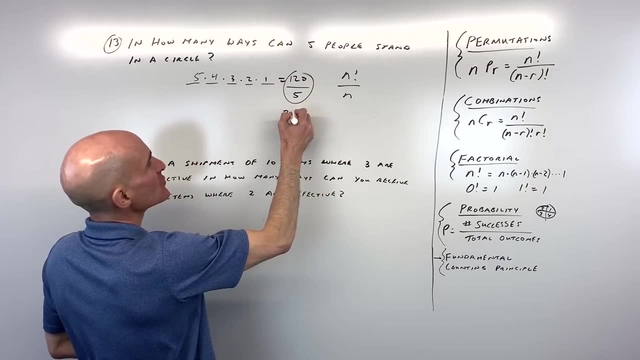 the same relative position to one another. So what you have to do is you have to divide by five. In the formula this would look like n factorial divided by n. so in this case there would be 24 different ways it can happen. Now, when you're doing these problems with some of these larger 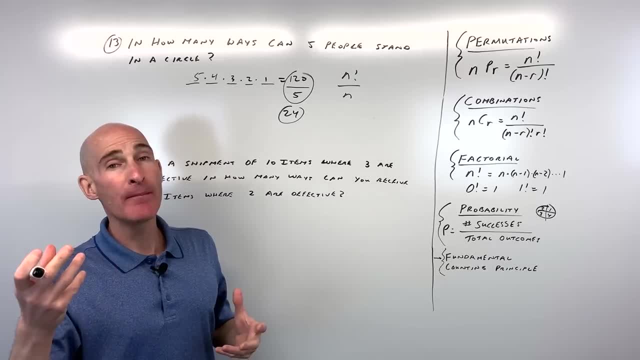 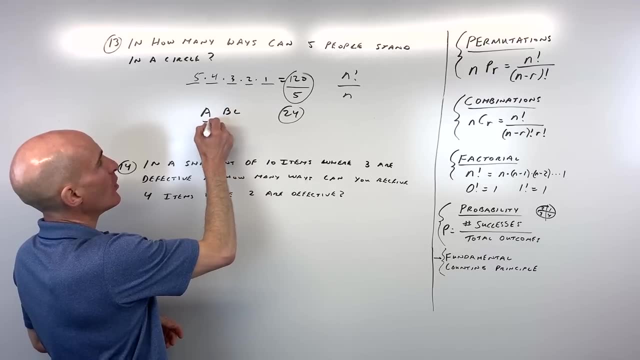 numbers, it gets a little bit abstract and what I recommend is to pose a simpler question. Maybe say, for example: the people are like this: uh, a, b and c, right, well, there's three people. that would be three factorial, which is three times two times one. there's six ways of ordering them in a row. 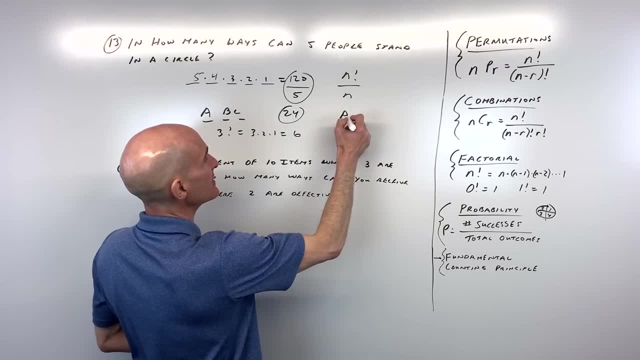 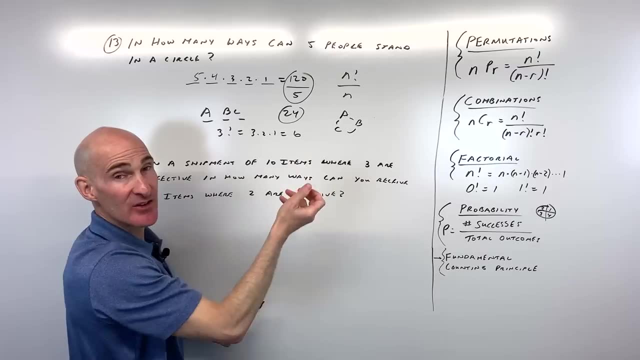 but imagine if it was in a circle now, like a, b and c, not much of a circle with three people, but you can see that like, so you can turn it like this one, two, you know what I mean. you can, you can rotate it. So that's, that's the idea here on this, on this problem. So let's look at number 14.. Here 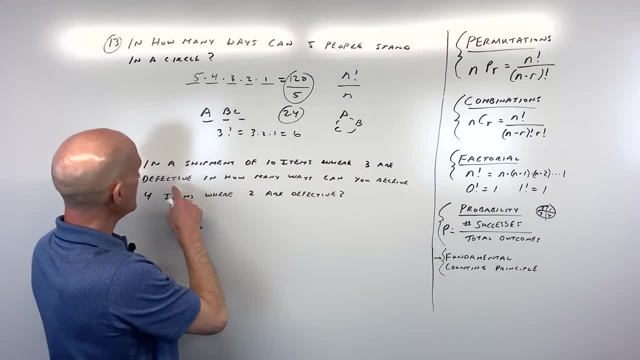 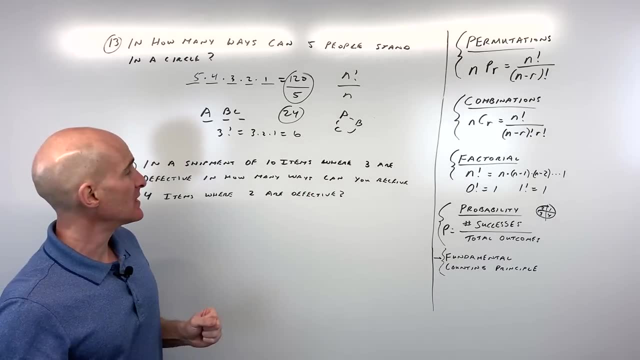 it says in a shipment of 10 items where three are defective, in how many ways can you receive four items where two are defective? Okay, so this one's a little bit challenging, in the sense that there's 10 items, three are defective. I'm just going to say three are bad, so that means that. 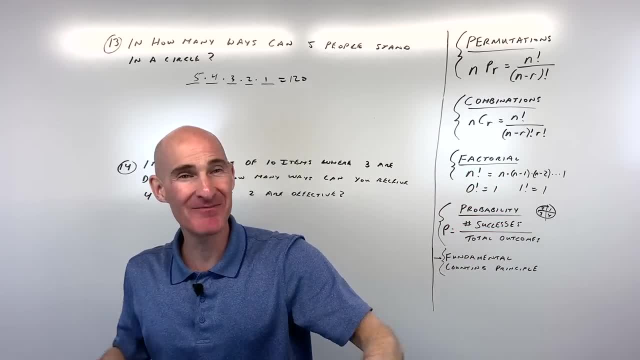 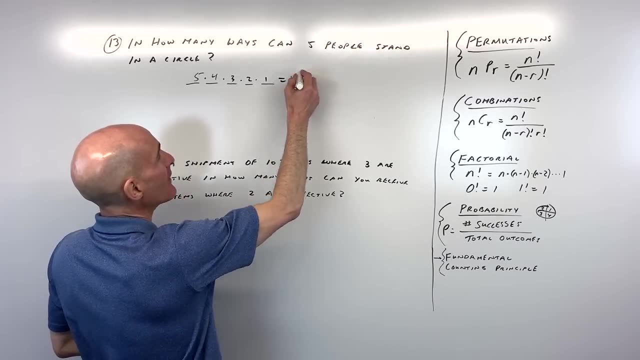 ever standing on your right when you keep turning like this, you're going to be in the same relative position to one another. So what you have to do is you have to divide by five. So if you wanted a formula, this would look like n factorial divided by n. 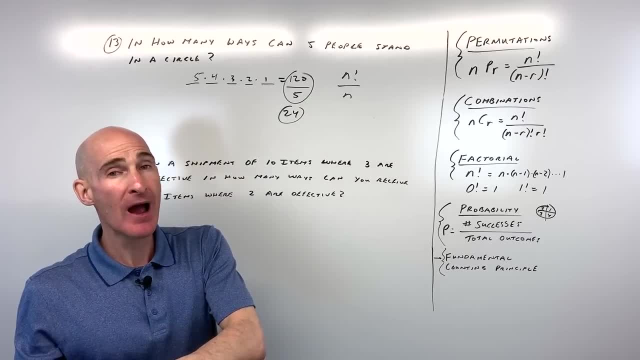 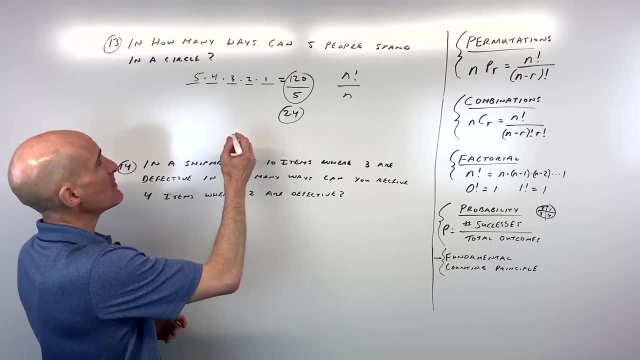 So in this case there would be 24 different ways it can happen. Now, when you're doing these problems with some of these larger numbers, it gets a little bit abstract, And what I recommend is to pose a simpler question. Say, for example, the people are like this: A, B and C- right, 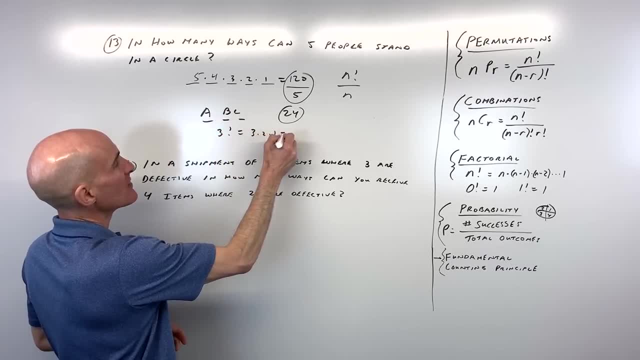 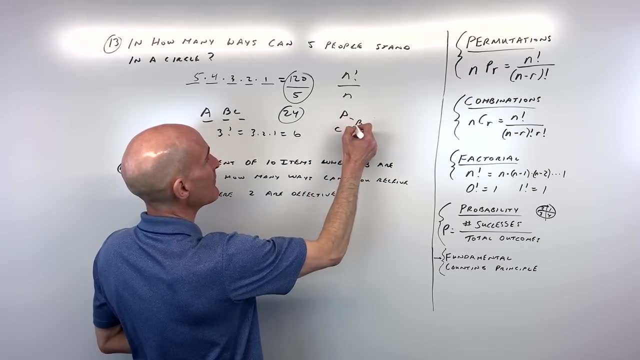 Well, there's three people. that would be three factorial, which is three times two times one. There's six ways of ordering them in a row, But imagine if it was in a circle now, like A, B and C. not much of a circle with three. 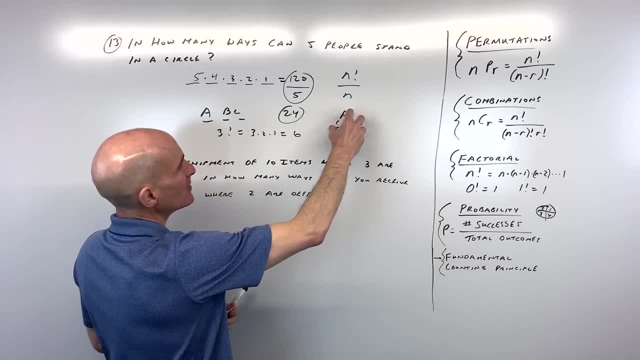 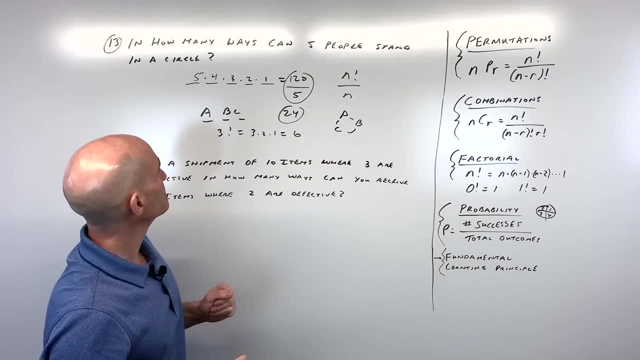 people. But you can see that like. so you can turn it like this one, two, you know what I mean. You can rotate it. So that's the idea here on this problem. So let's look at number 14 here. 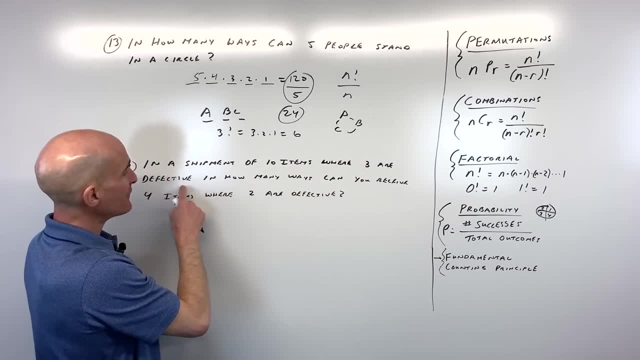 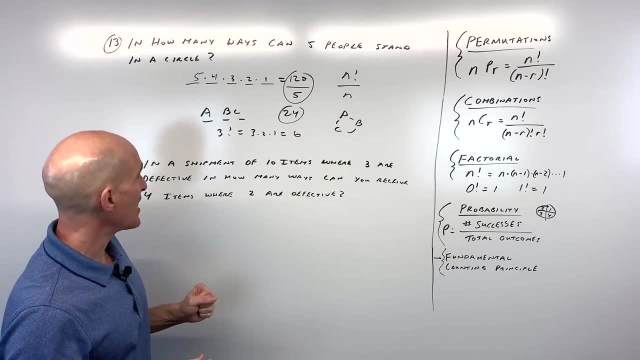 It says Okay. so this one's a little bit challenging in the sense that there's 10 items, three are defective. I'm just going to say three are bad. So that means that seven are good. So let's say seven good, three are bad. 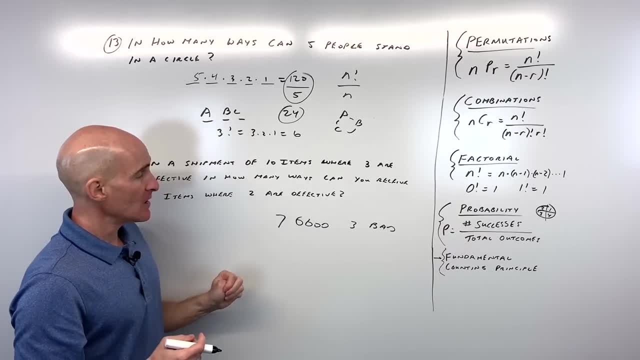 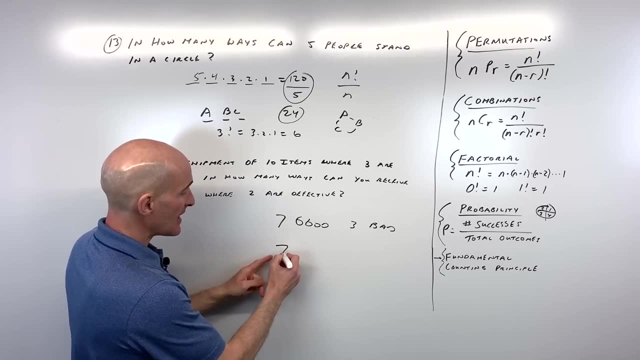 But you're trying to receive the shipment where you're going to get four items right. You want to find out how many ways are to get two defective or two bad. That means that two are good. So the way this would happen is: there's out of the seven good, how many ways are there? 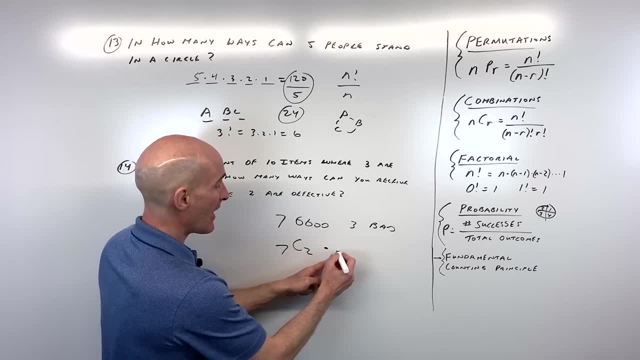 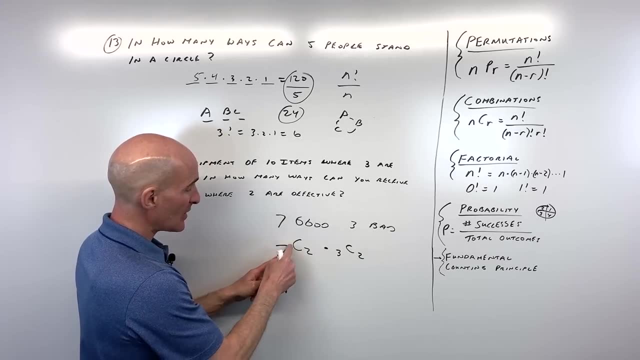 to choose two times out of the three bad. how many ways are there to choose two of those three bad ones? and you're going to multiply these together. So again, remember that first number. that's how many are in that group? seven, good, how? 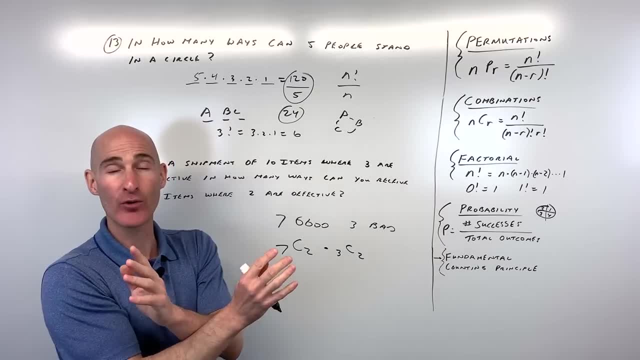 many ways are there to choose two out of seven where the order doesn't matter, it's not important? And out of the three bad ones, how many ways are there to choose two where the order is not important? So let's go ahead and multiply those together.